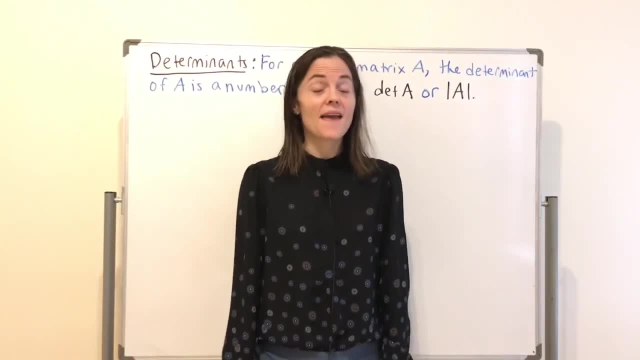 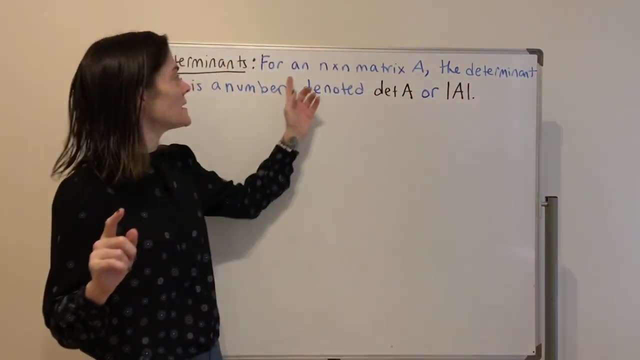 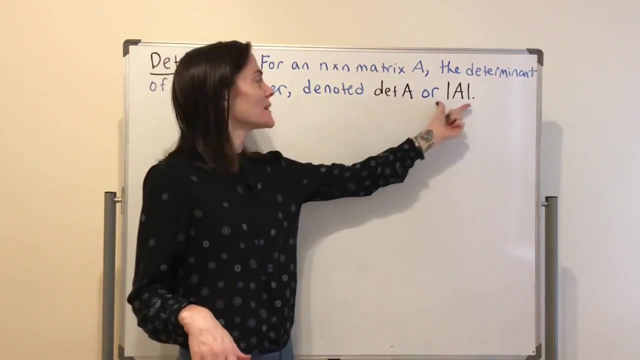 What is the determinant of a matrix? First of all, it's only defined for square matrices. We need square, okay. And then the determinant is a number. Here's some notation, or like this: It looks like absolute values, but when a matrix 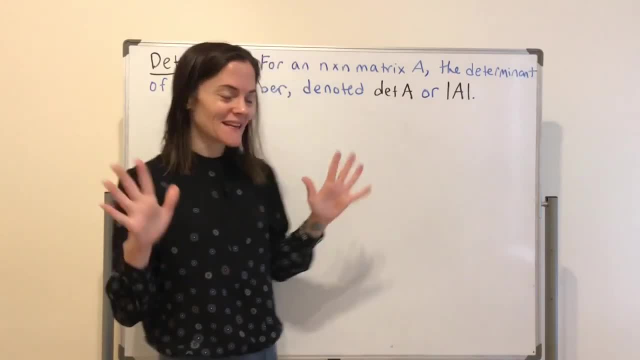 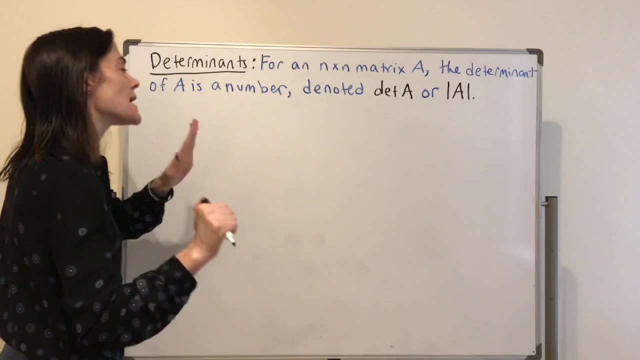 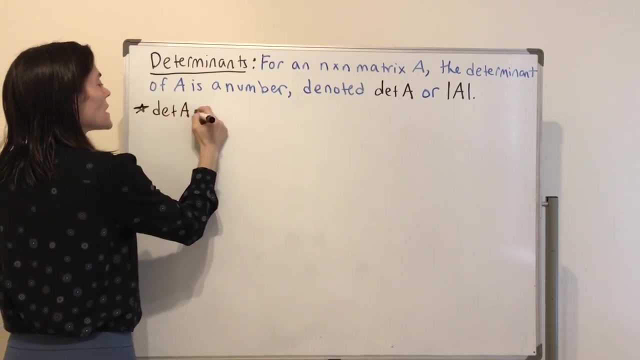 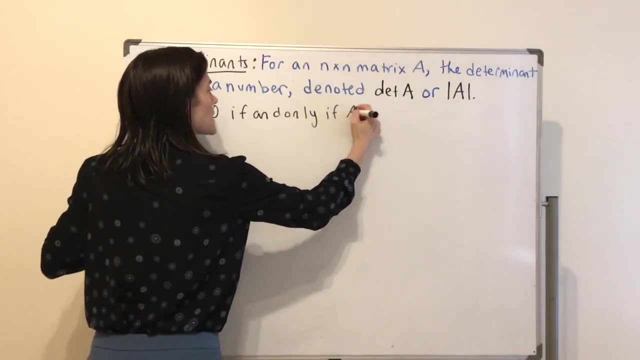 is on the inside. this stands for determinant. Okay, well, the most important thing, or I should say, okay, determinant is a number. And then- this is one of the key properties- that the determinant of A is not equal to 0 if, and only if, A is. 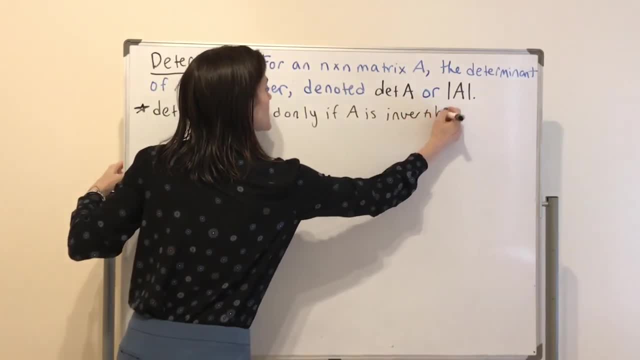 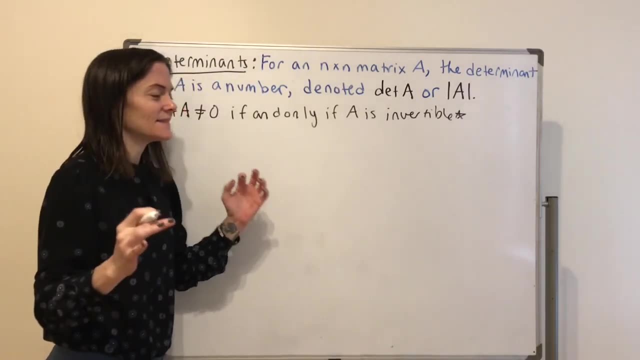 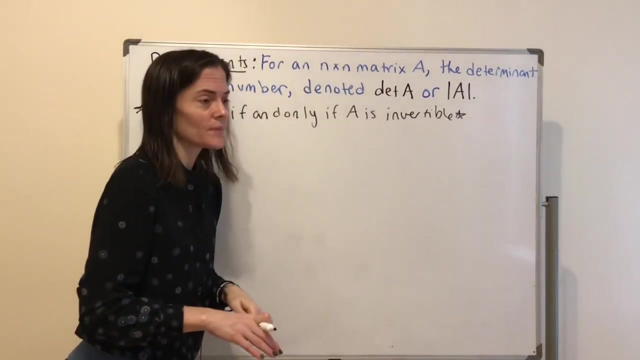 invertible. This is one really nice thing about determinants, and we will begin with many properties of the determinant, but a key one is that this is a number. number is not equal to zero. if, and only if, your matrix is invertible, okay, well, 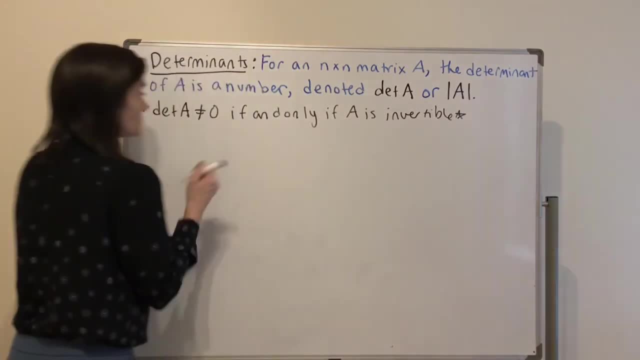 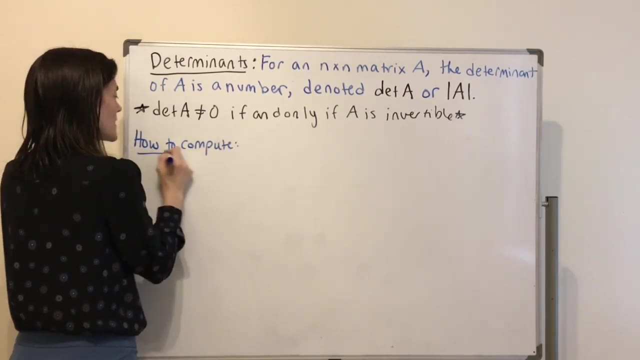 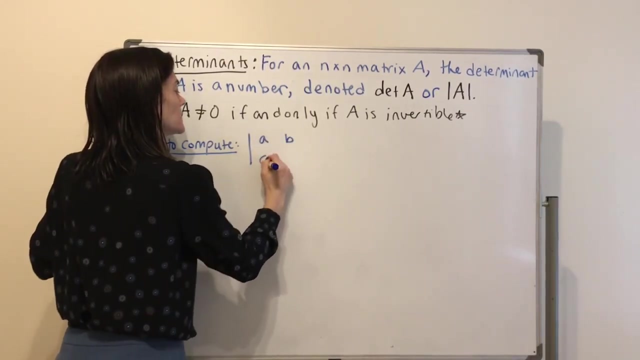 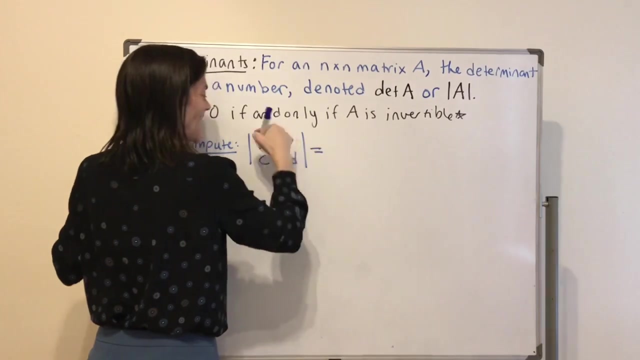 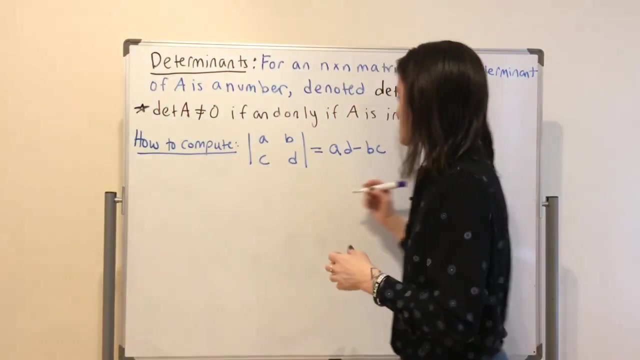 how do we compute a determinant? we know how to compute for a 2x2 matrix, and this we discussed quite a while ago here. see these bars. is these bars? okay, good, this is a D minus BC. this is the determinant for 2x2 matrices. 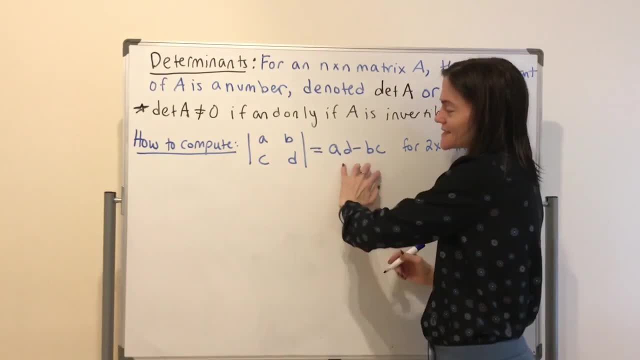 and we know, of course, this number being nonzero, is quite important for a 2x2 matrix to have an inverse, because the inverse of a matrix, ABCD, is 1 over this. and then you flip the diagonals, take negative of the off diagonals and to take one over a number. 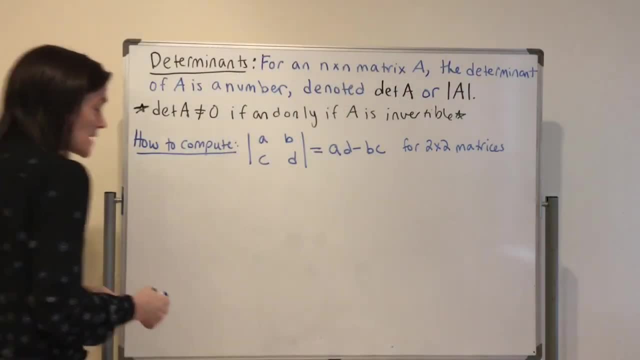 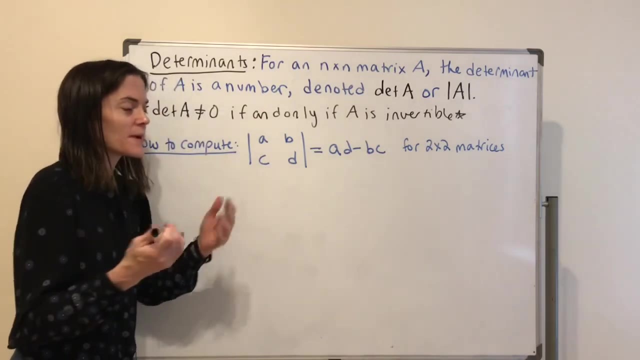 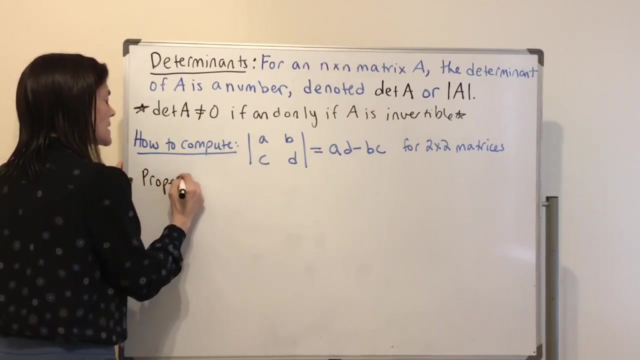 and we need it to be nonzero, very nice. well before we get into how to compute for three by three, four by four, five by five, things like this, I think it's important to understand the properties. we will now discuss some properties, and I'm not too going to do every single property at once, because the German it. 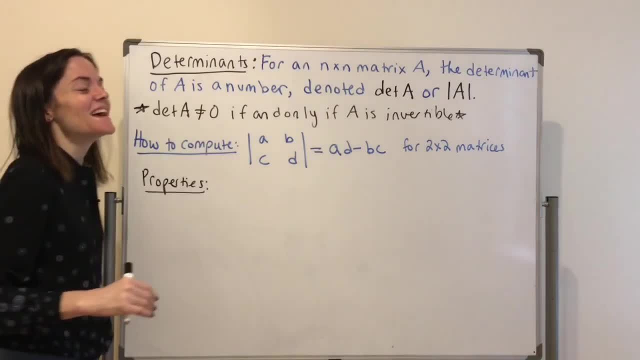 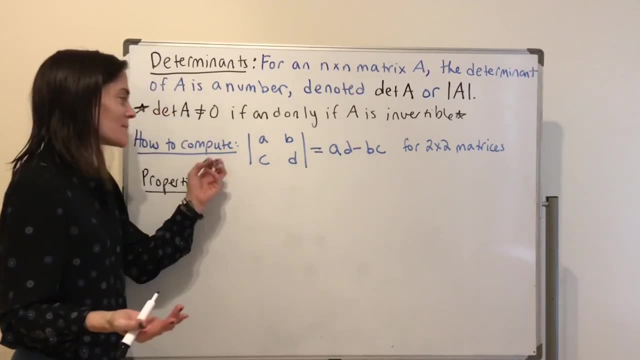 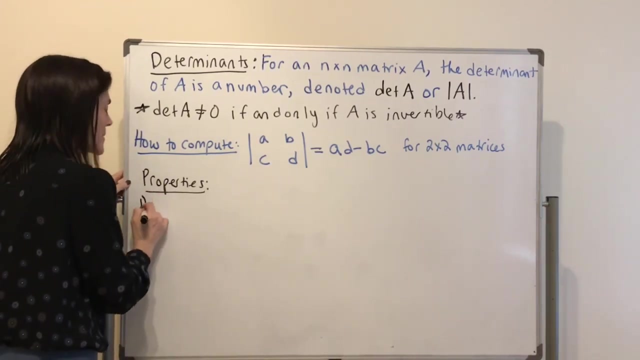 has so many properties. well, one will you've already mentioned, but we're going to do a number of them. then we will talk about how to compute for larger matrices, and the first one that I would like to mention. so what I'm going to do here's: 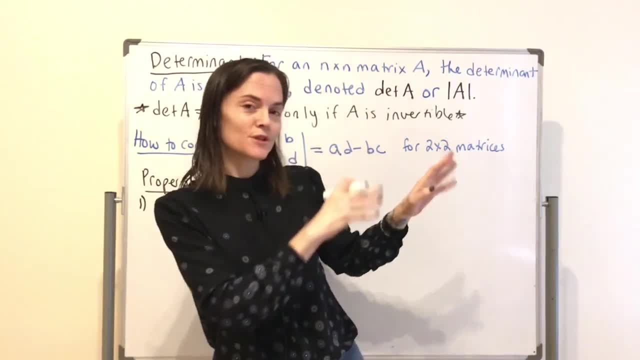 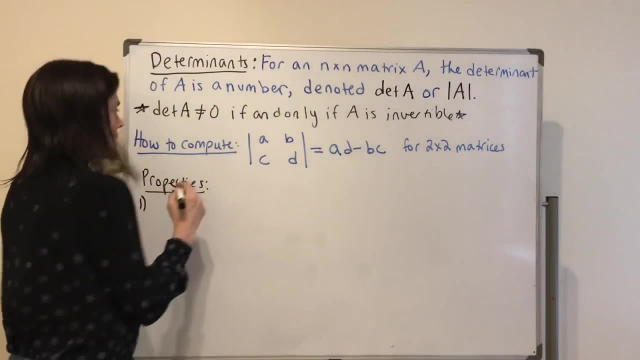 gonna be what I do. show up for a two by two matrix property. show up for a two by two matrix like this. this is how we're going to do, at least for at the beginning. okay, well, the determinant of the identity matrix is one, and now let's show it for two by two. 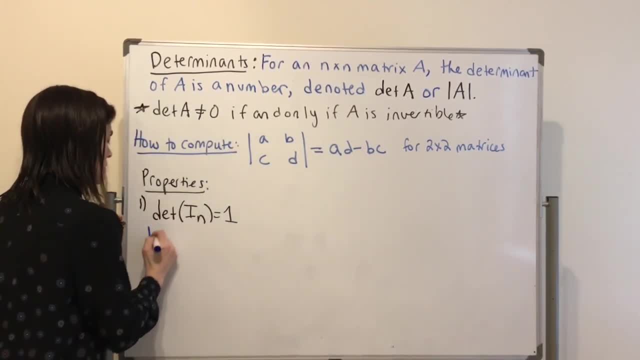 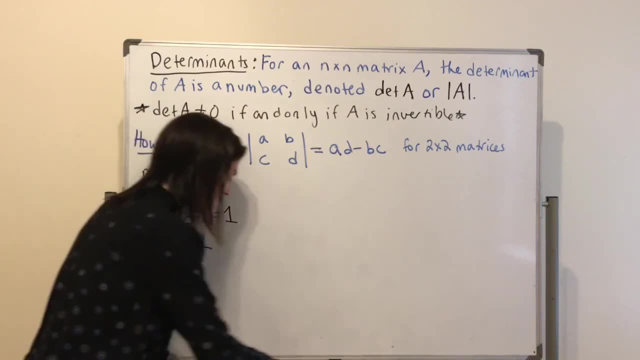 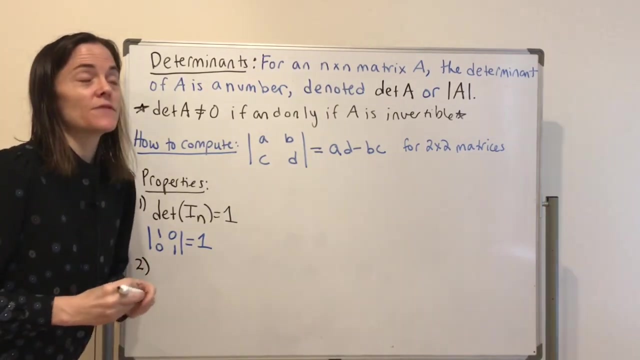 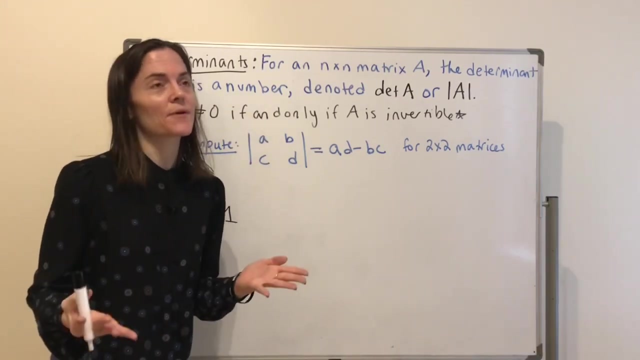 okay, that one wasn't too hard. but what's the next property that i want to mention? okay, if you take a matrix a and you interchange two rows, this is one of our elementary row operations. this multiplies the determinant by minus one, okay, so if you take a matrix a and you interchange two rows, this is one of our elementary row. 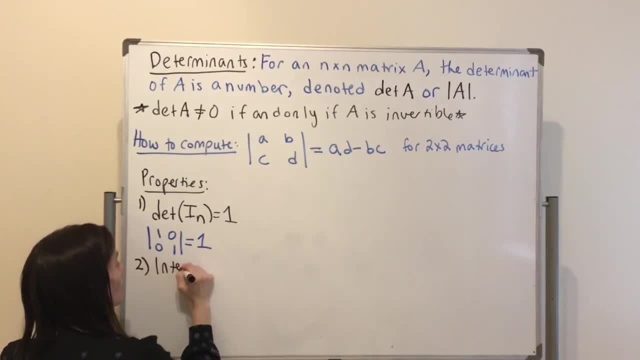 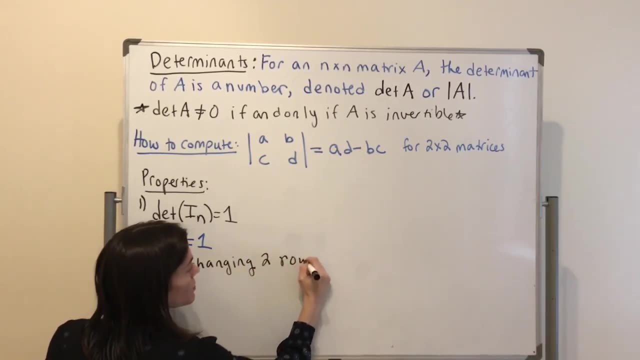 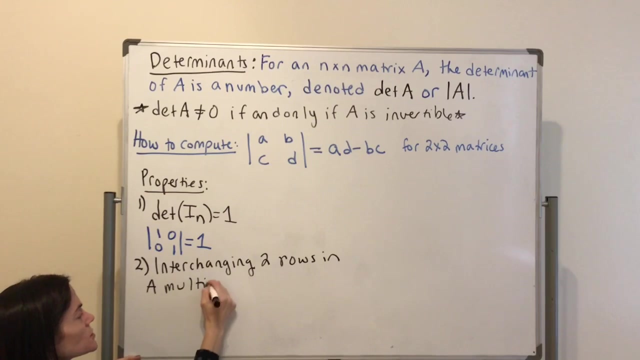 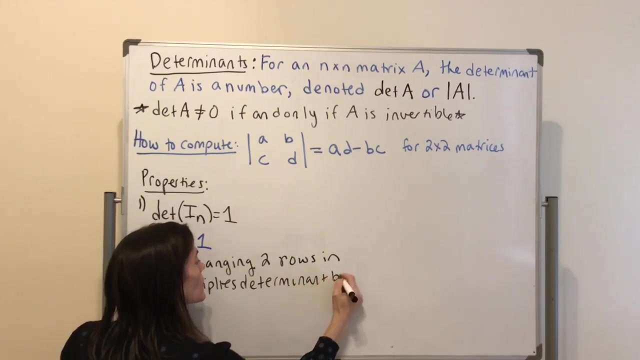 okay. so interchanging two rows in a matrix, a multiplies the determinant by minus one. okay, now let's see this for two by two matrices. okay, now, let's see this for two by two matrices. well, what i'd like to do is look at this: c, d. 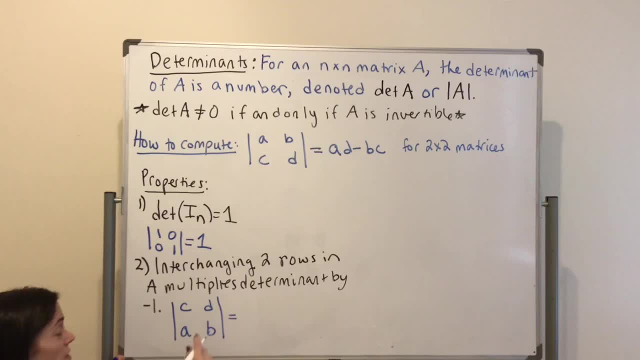 well, what i'd like to do is look at this c d. well, what i'd like to do is look at this: c d, a b, this determinant, a b, this determinant, a b, this determinant. i've just interchanged the only two rows. i've just interchanged the only two rows. 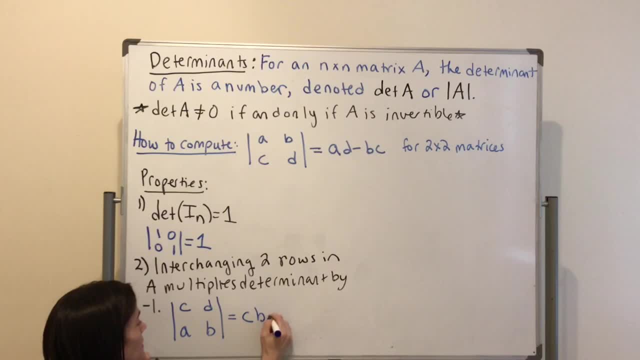 i've just interchanged the only two rows of this matrix. well, this is of this matrix. well, this is of this matrix. well, this is c b minus d a, c b minus d a, c b minus d a. which is? which is? which is negative, negative, negative a d minus b c. 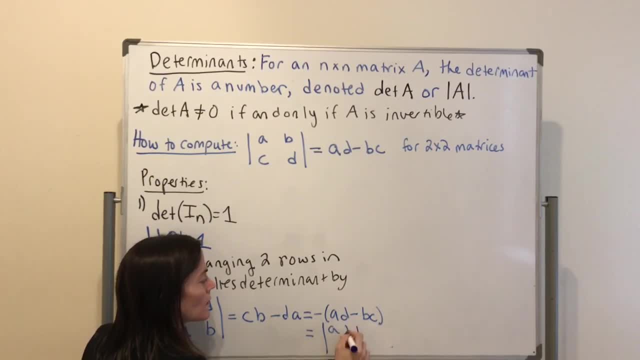 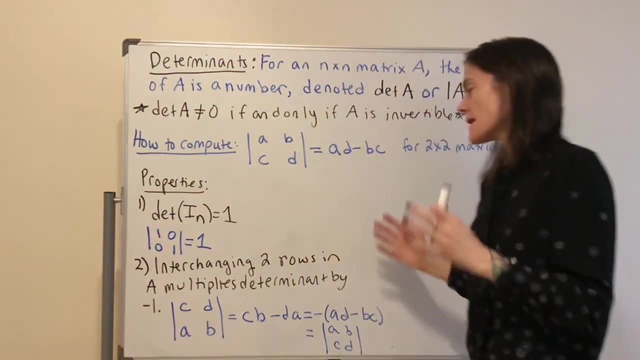 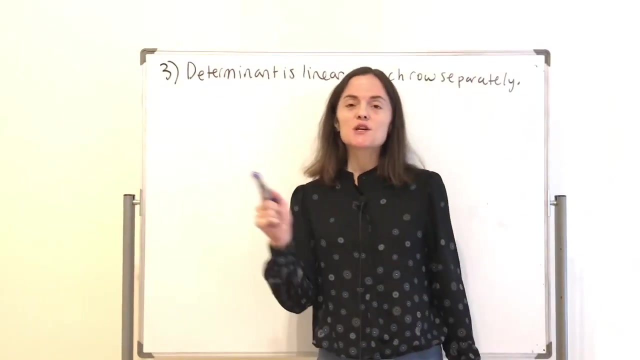 a d minus b c, a d minus b c, and this one is this determinant and this one is this determinant and this one is this determinant. Okay, so we see this property for a two by two matrix, but everything I mentioned, or I will mention, these properties hold in general. Property three says the determinant. 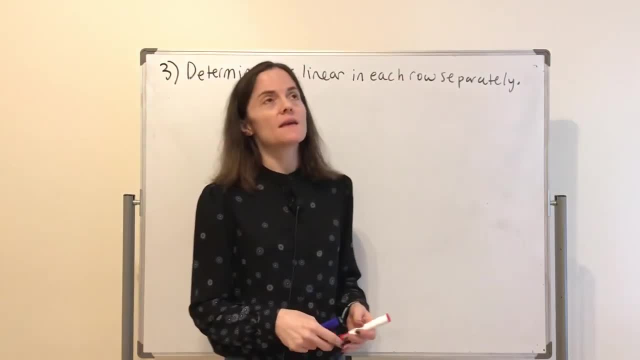 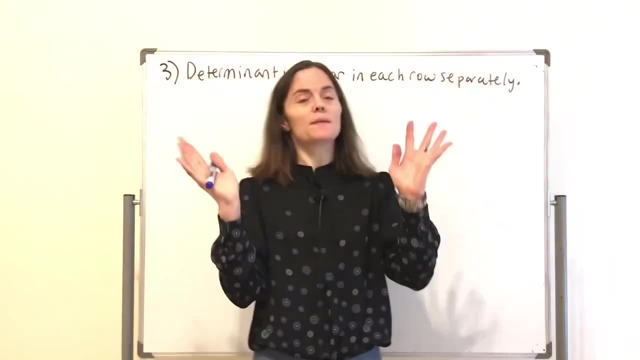 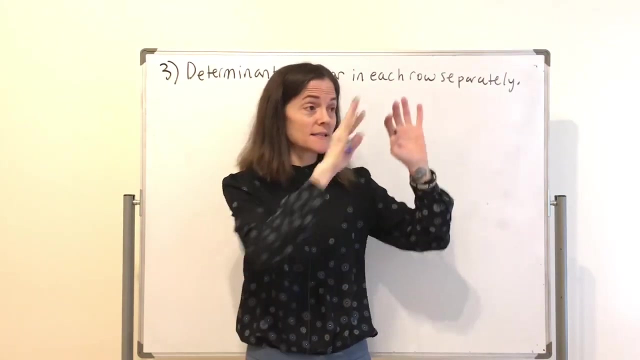 is linear in each row separately. This is referred to as multilinear, but let's talk about what this means. What is linear? Remember when we talked about linear transformation. say it says T of X plus Y is T of X plus T of Y and similarly, the other part of linear was that T of 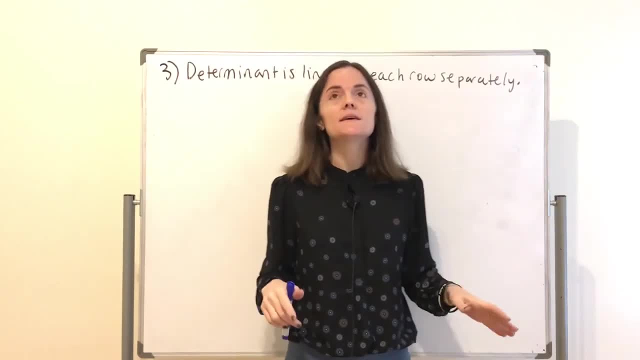 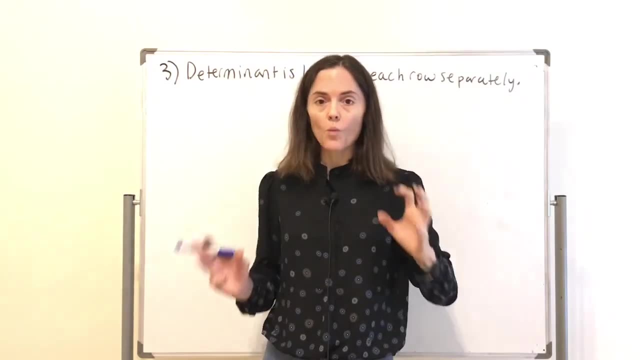 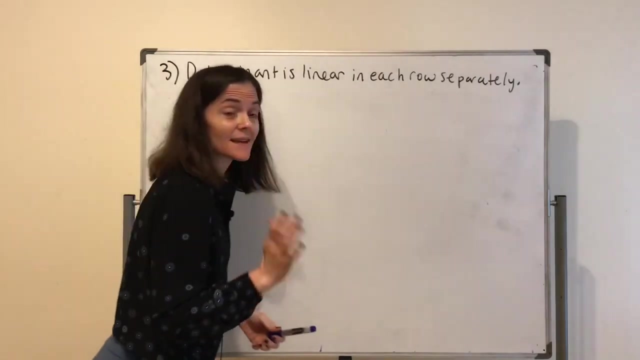 KX is K times T of X, and this is the same notion, except it's in each row separately. so if you fix all the rows but one, then it's linear in the one that you did not fix. So let me make that explicit in the two by two case here where we will actually check this linearity. 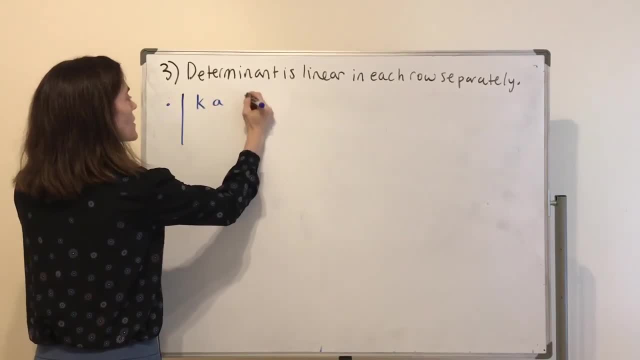 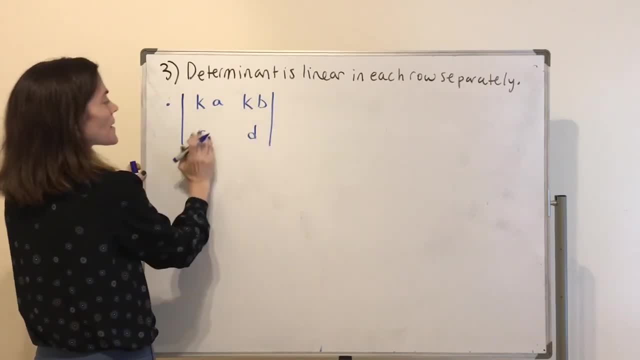 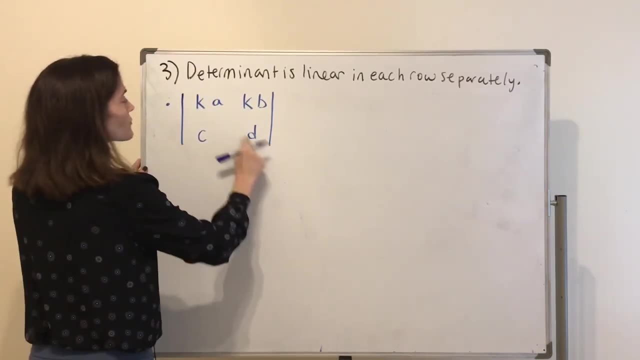 multiple here. so you see, I'm fixing the second row, although I could have made the same argument and fix the first row, it would work out also. but you fix one row and now I look at this determinant. I take a multiple of this row. well, this is. 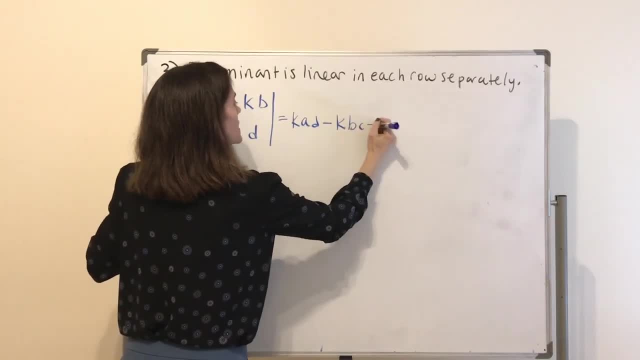 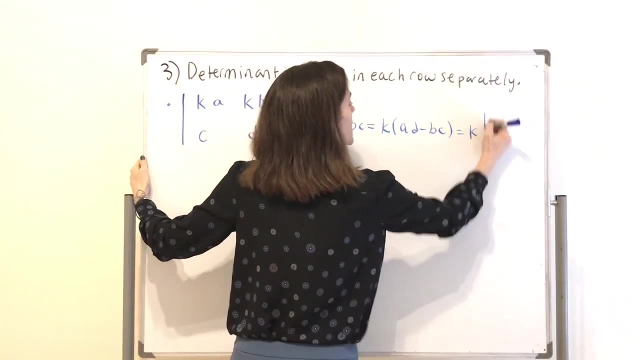 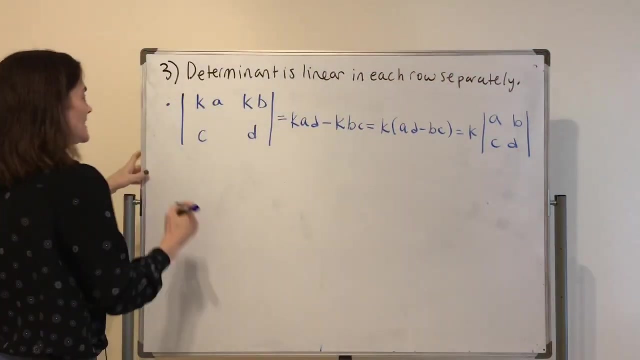 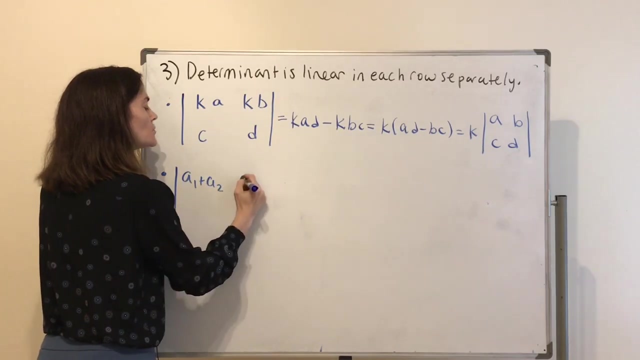 K AD minus K BC. this is K a, B minus BC and you see this is K times this determinant: a, B, C, D. okay, and the second part of linearity is if you have a sum, say you have an a 1 plus a 2 and a B 1 plus B, 2, C, D, right. 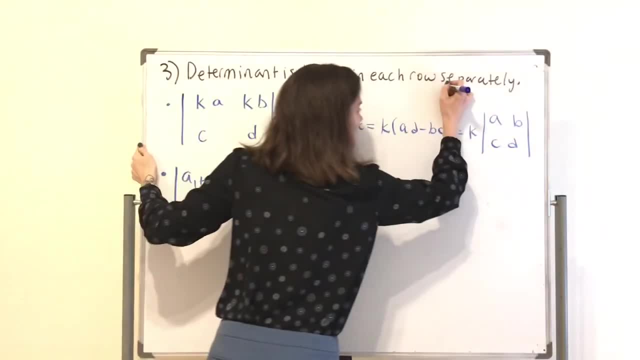 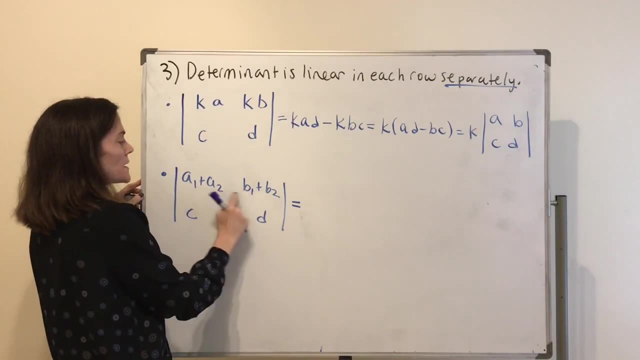 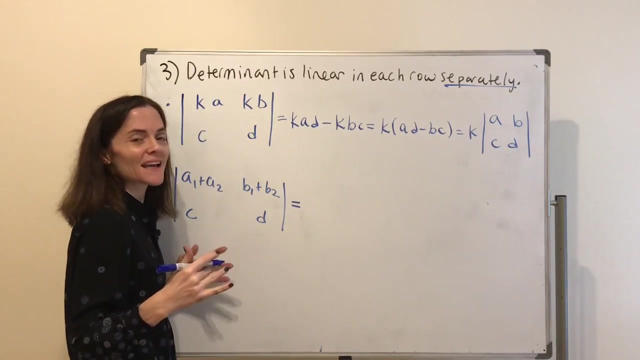 just a 371.. in one row, underline: very nice, okay. well, what is this? it should be a 1 b, 1 c d and a 2 b, 2 c d, sum of those two determinants. but let's see it, we are verifying a lot of these properties. 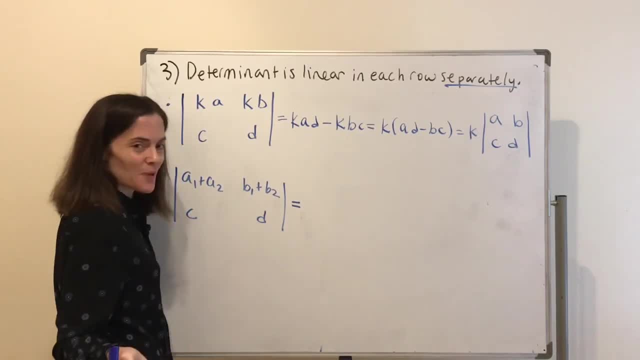 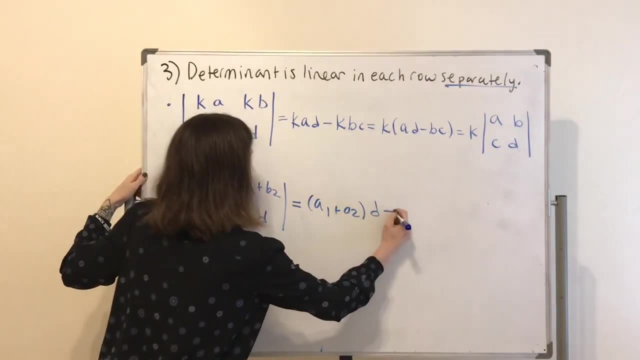 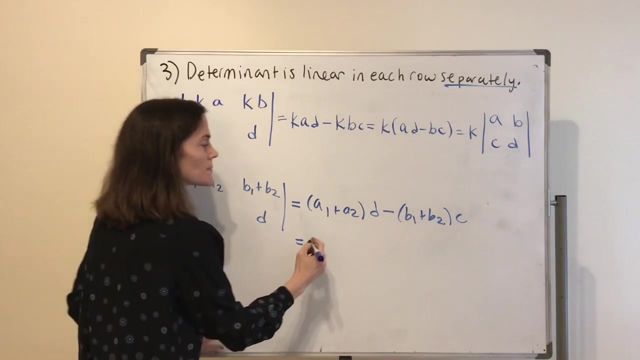 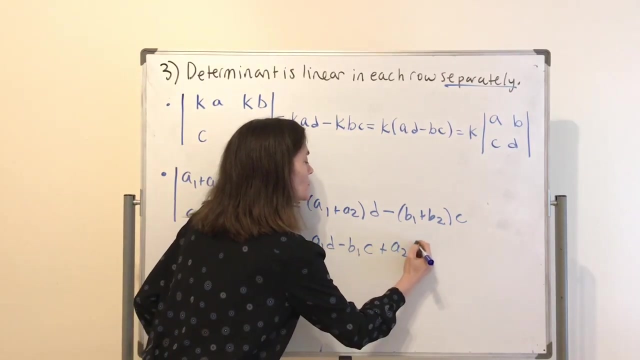 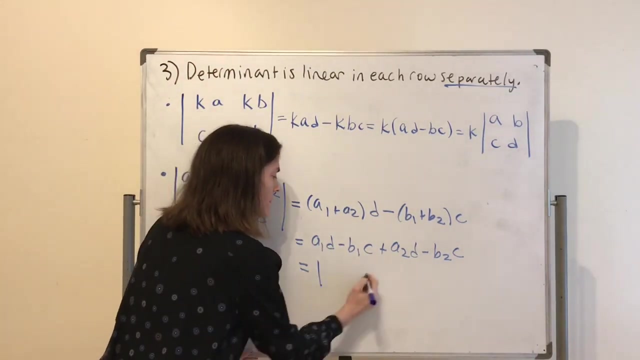 initially for two by twos helps us understand what the property is saying. okay, here we go. this is a 1 plus a 2 times d minus b 1 plus b 2 times c. and now what I need to do is just rearrange some things. this is a 1d minus b 1c, plus a 2d minus b 2 c. and now, look, this is a determinant. 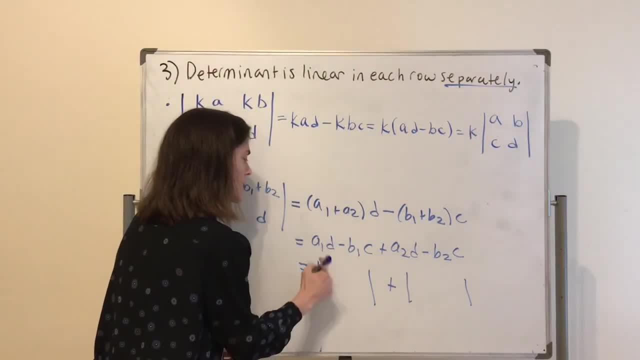 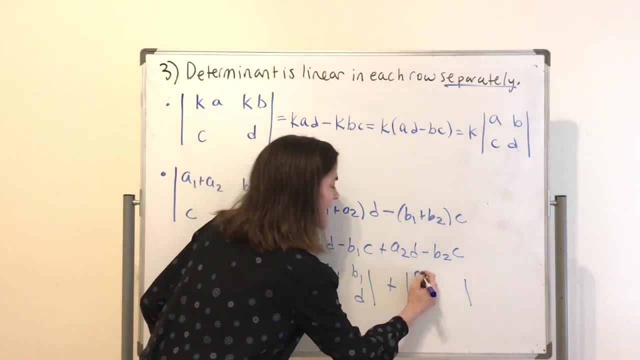 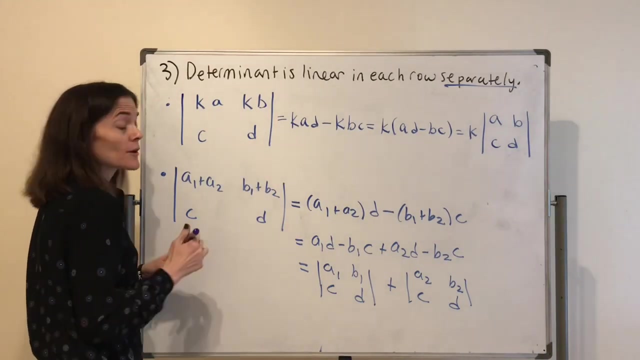 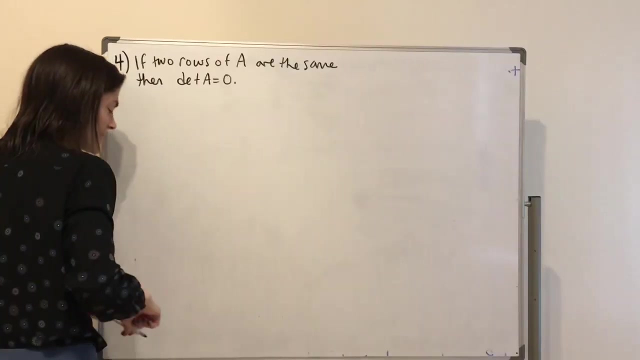 this is a determinant. this one one is a1, b1, c d, This one is a2, b2, c d And this is the linear, in each row separately property that I was referring to here. So this is property three. This property, if two rows of a 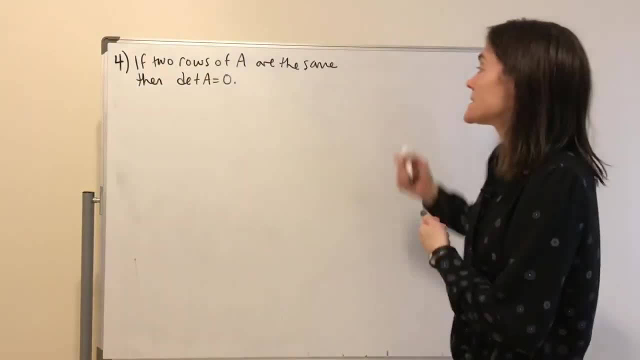 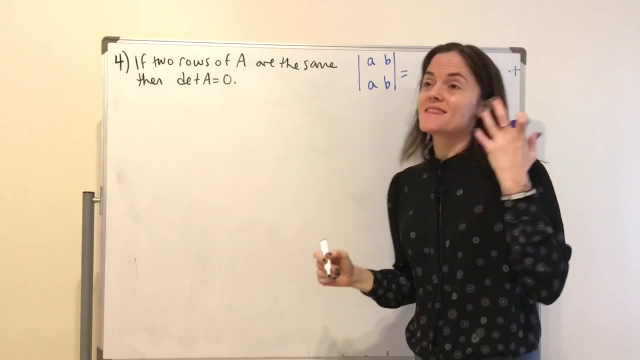 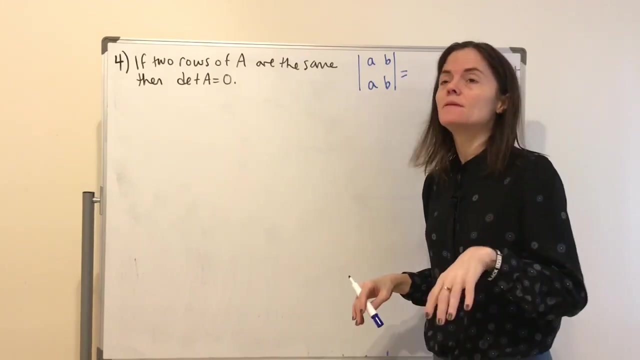 are the same, then the determinant is zero. We can see this for two by two, like this, But also just thinking about it, although I haven't verified this. generally, if you have two rows of eight that are the same, the matrix is, without a doubt, not. 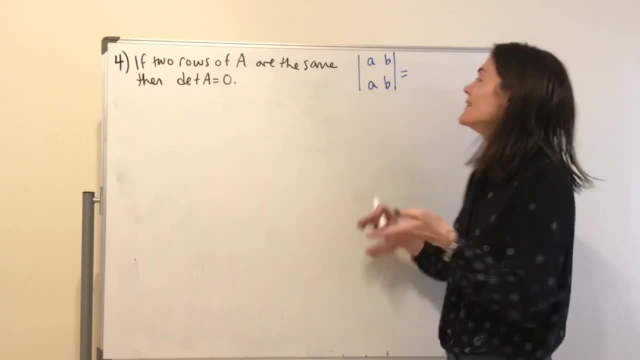 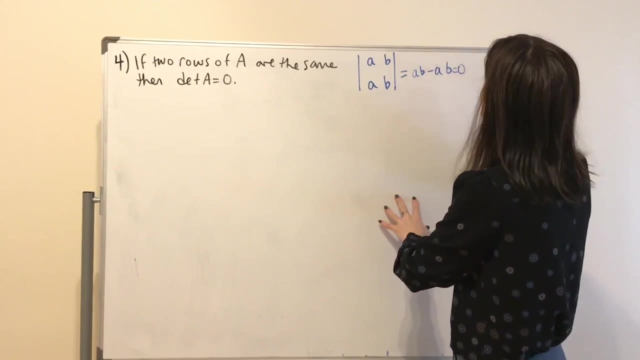 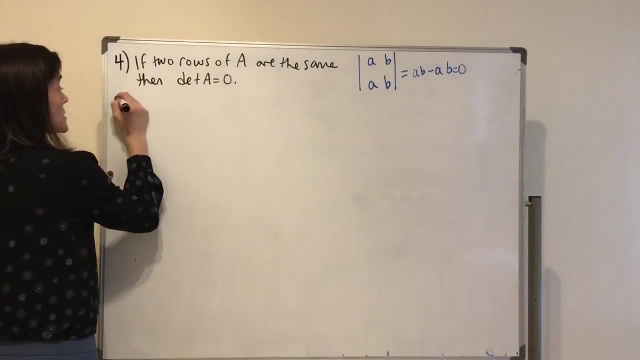 invertible right, Because the rank will not be n. But just to verify this, you can see we get ab minus ab, which is zero. And then one more thing that I want to say right now, which is going to lead us into some great observations, is adding a multiple. 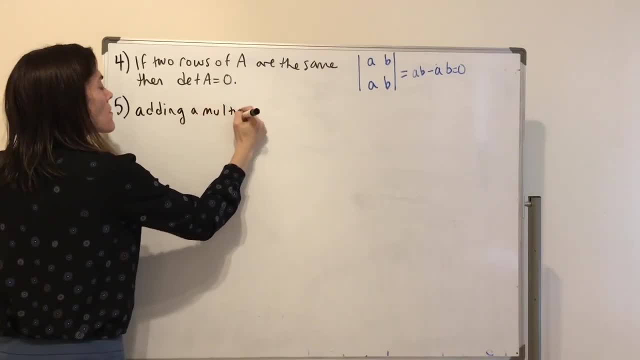 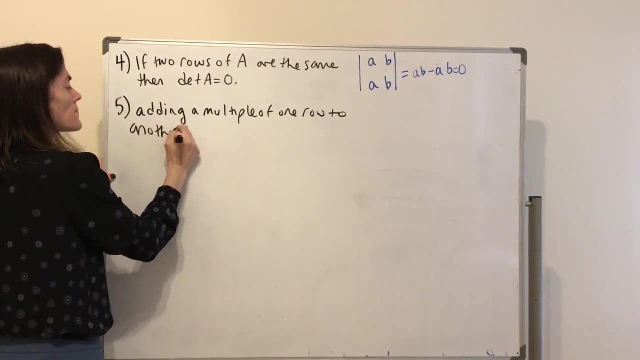 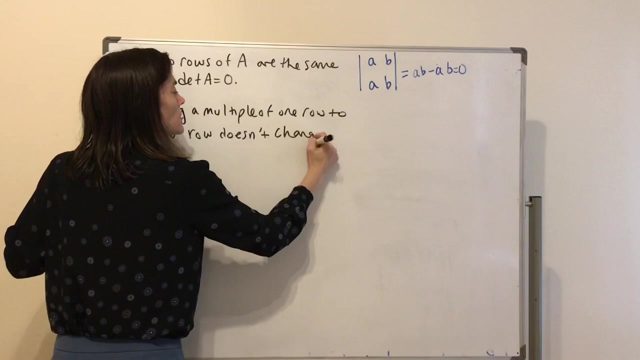 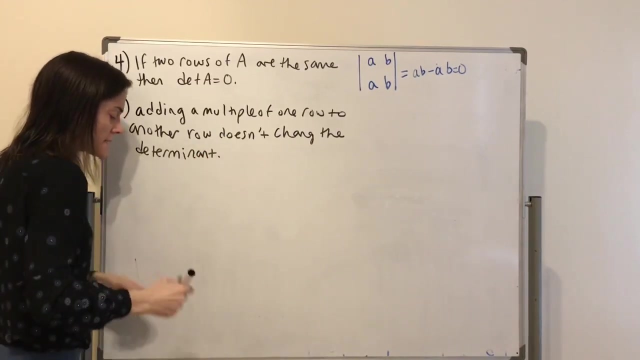 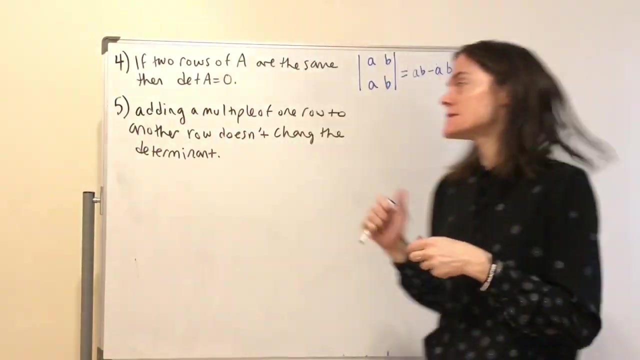 of one row to another row does not change. Now, why must this be true for two by two, right? This is all we're looking at so far, because we know it's a very simple formula for two by two matrices, and we can see these. 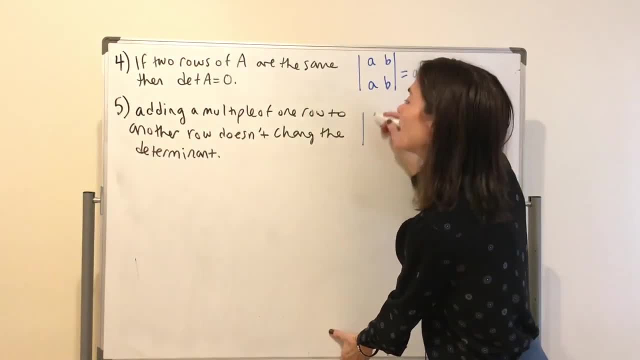 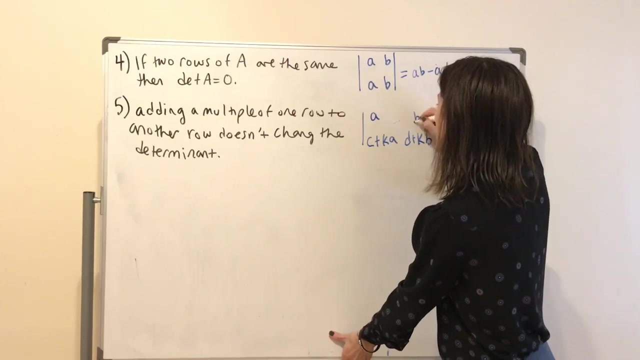 properties in action. Okay, well, what does this look like? Something like ab and then say c plus k, a and b. So we're going to add a multiple of a, b, c, d plus k, b. Maybe I should now space this better. 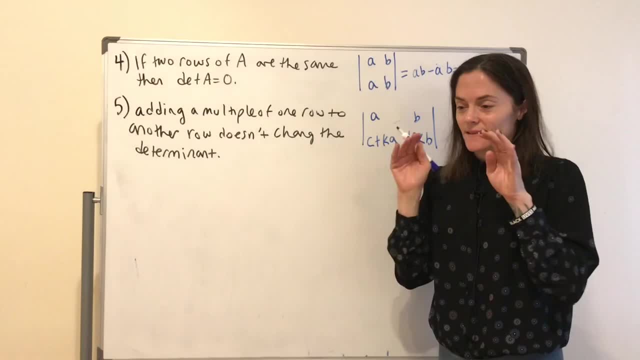 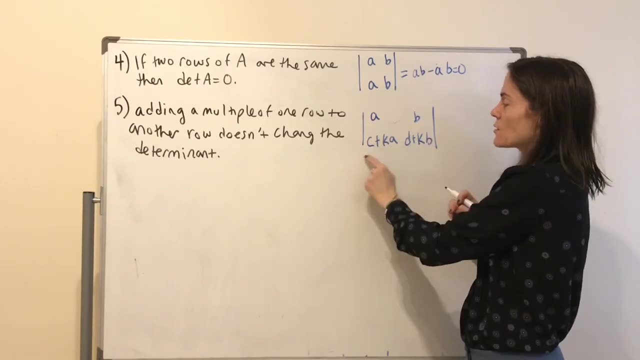 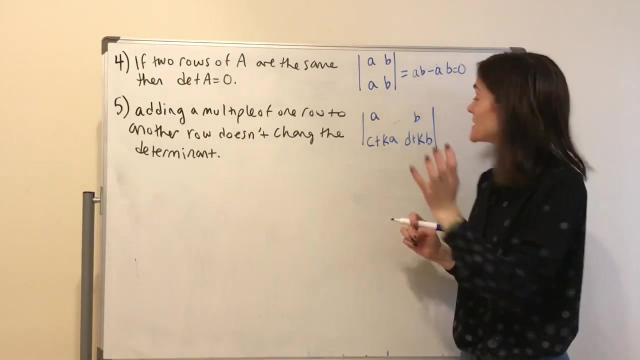 Right, What I have done is I took ab c d and I added this multiple, multiple of this row- to this row. right, We should get the same here. if this property holds, which I'm saying it does- we should get the same determinant as the determinant of ab c d. 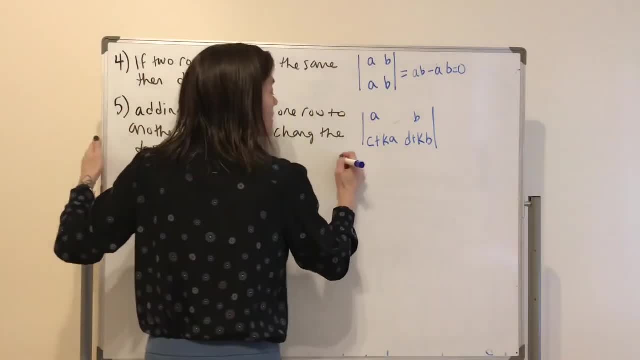 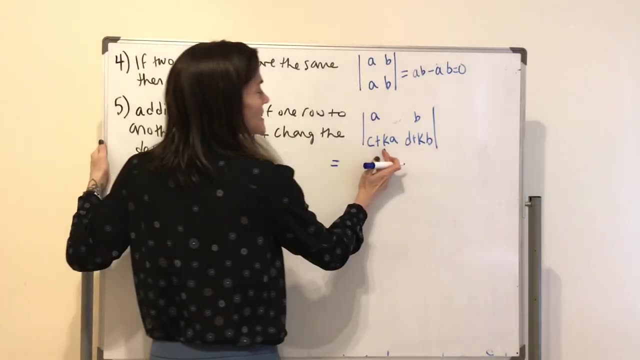 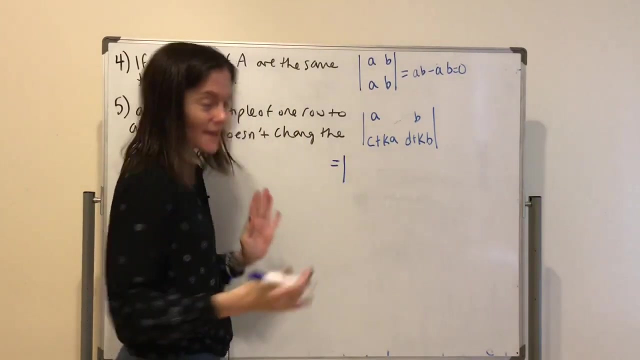 So here we go. Let's look at this one and I will. okay, we're going to use properties we've already discussed. So you notice, here this is a sum, so this and it's linear in each row separately. 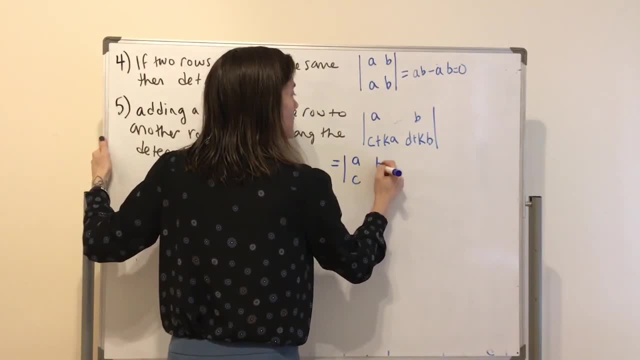 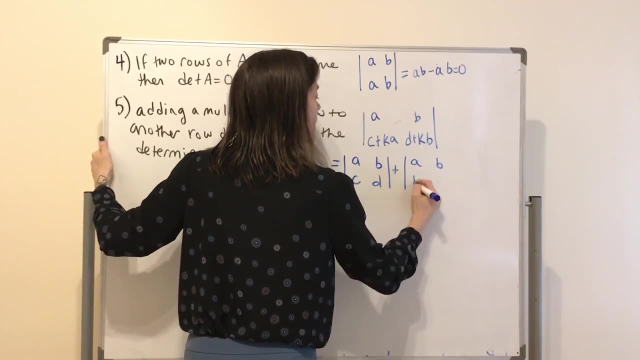 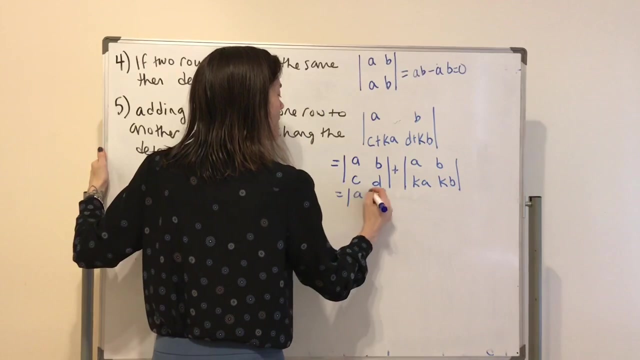 So this will be a, c, b, d plus. this is going to be this: a, b, k, a k b, That's using the sum part of the linearity and then using the constant multiple part. 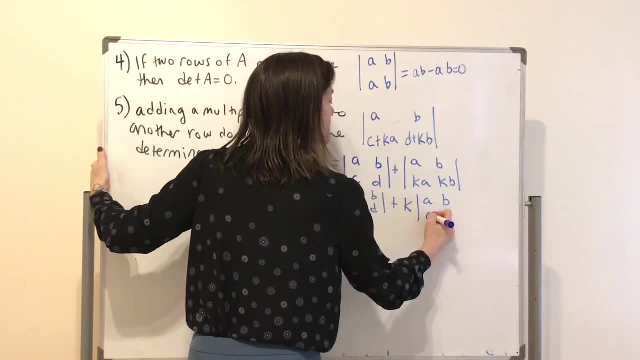 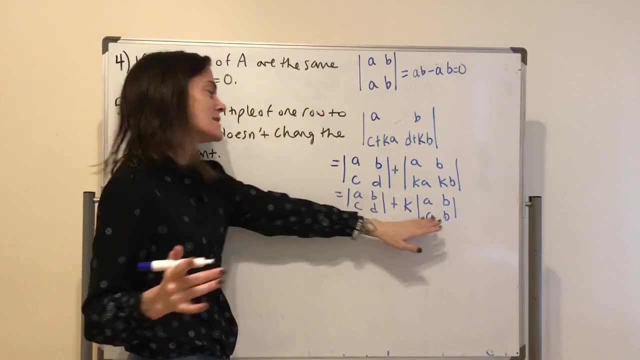 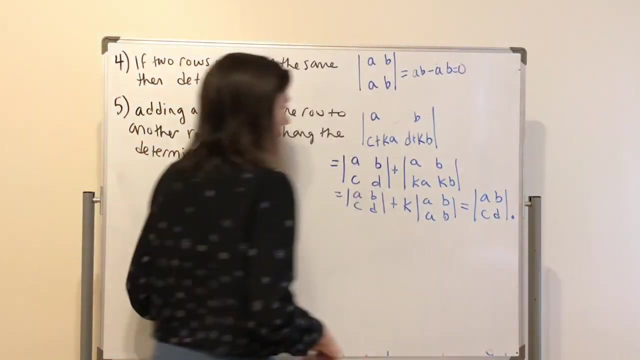 of the linearity in each row. we get this, And now this matrix is has a. two rows are the same, so this determinant is zero and in fact we do get. this is just ab, c, d, Okay. 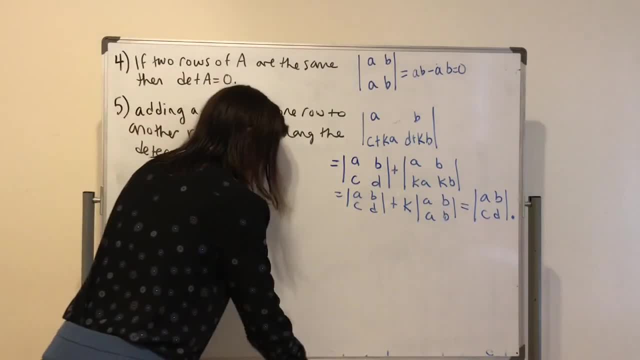 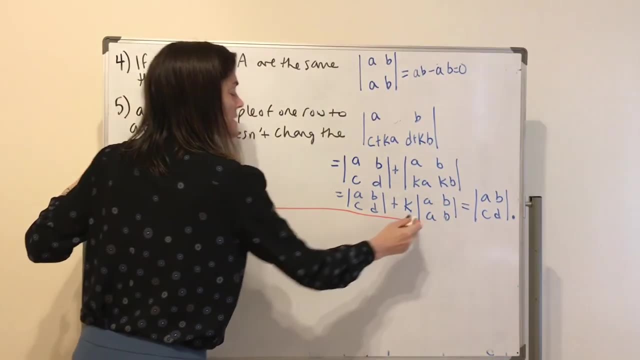 Now. so what we see now. I'm going to parse this out Now. I'm going to pause. now We have a lot more properties to discuss, but I'm going to start with these five for the moment and I'm going to make some observations. 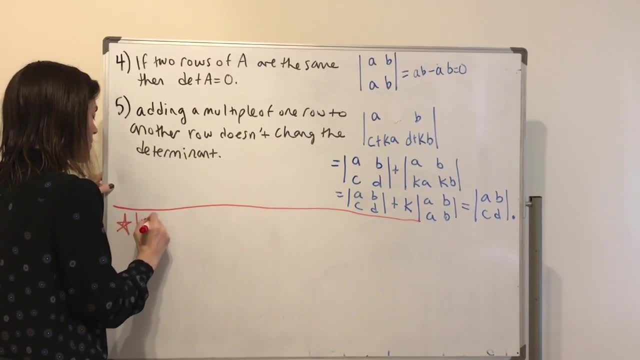 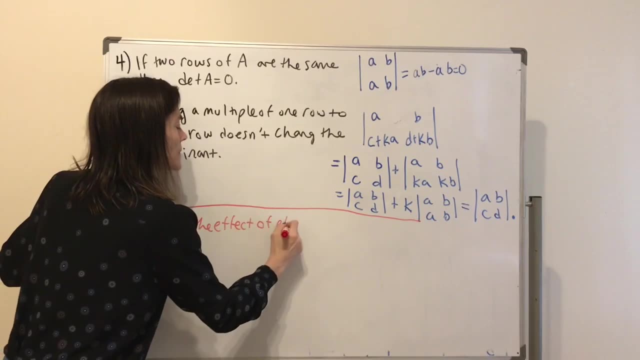 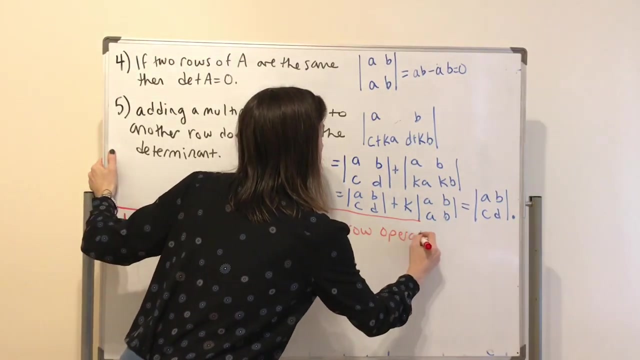 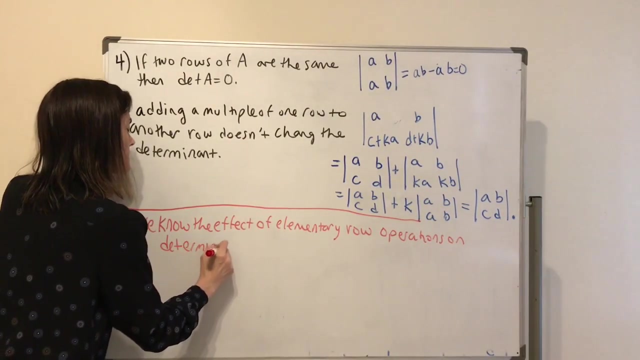 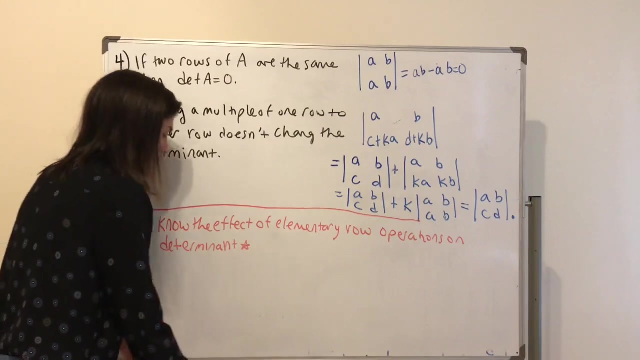 Okay, What we see is, we know the effect of elementary row operations on, let's say, a, b, c, d, d. Okay, On the determinant, Combining a few of the properties we have mentioned. right, because what are the elementary? 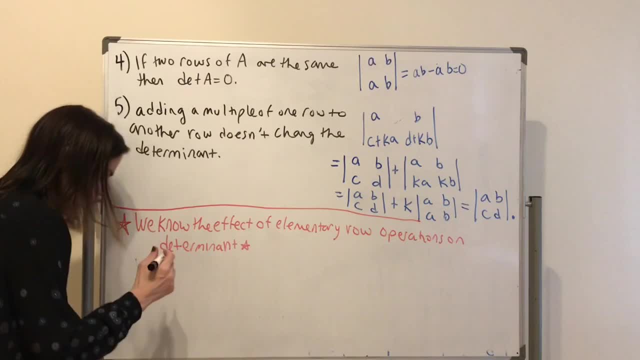 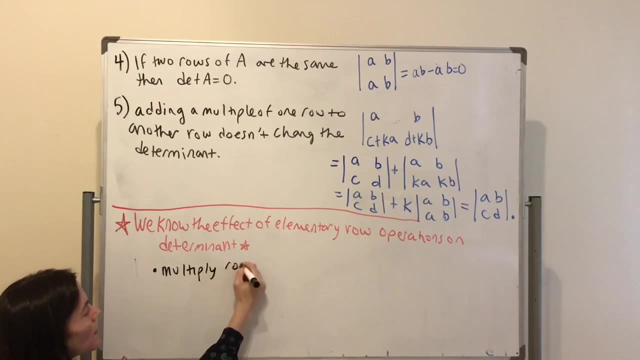 row operations. This goes back to the first week of class. Okay, Well, if you multiply a row by a constant, a row by a non-zero right, Okay, Okay, Okay. What if you multiply a row by a zero constant? 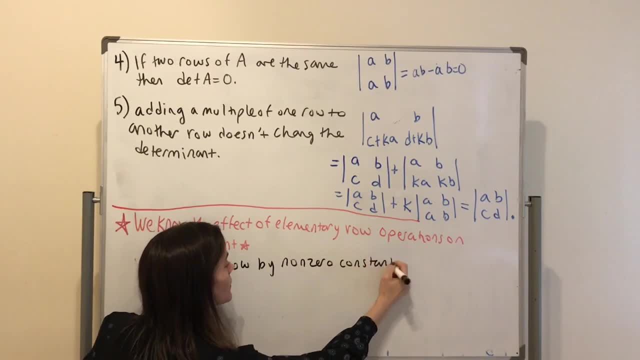 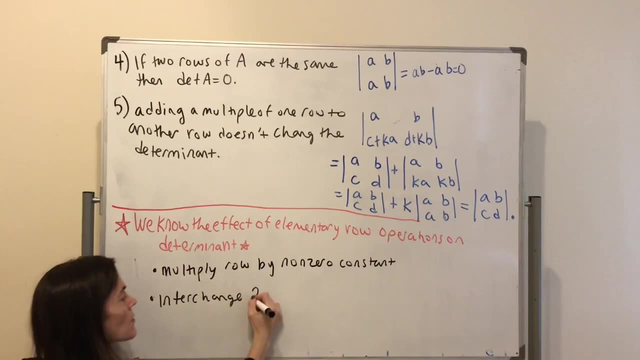 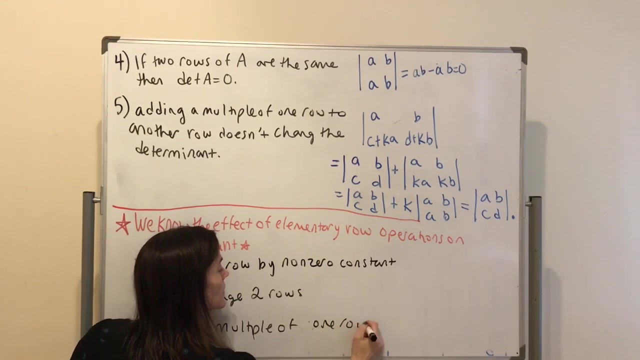 You can interchange two rows and you can add a multiple of one row to another, of one row to another. Okay, Okay, Another. What effect did each one of these have on the determinant? Well, the last one. it's still on the board. 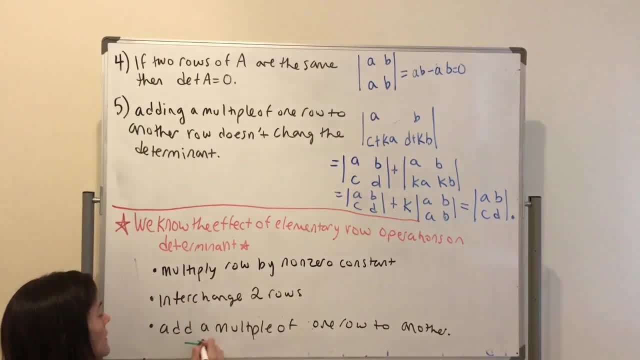 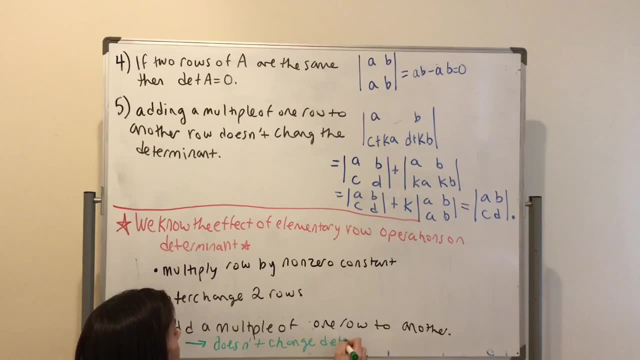 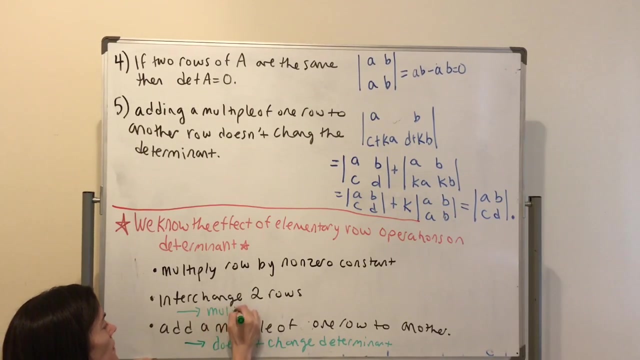 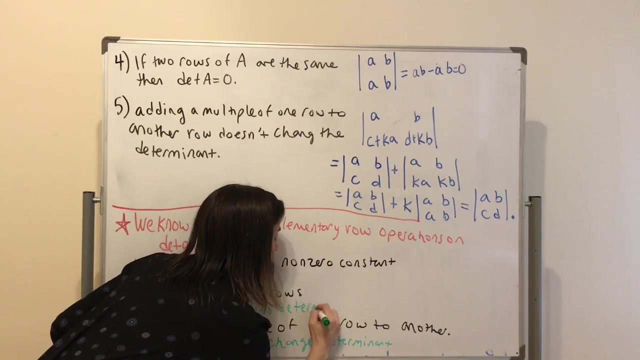 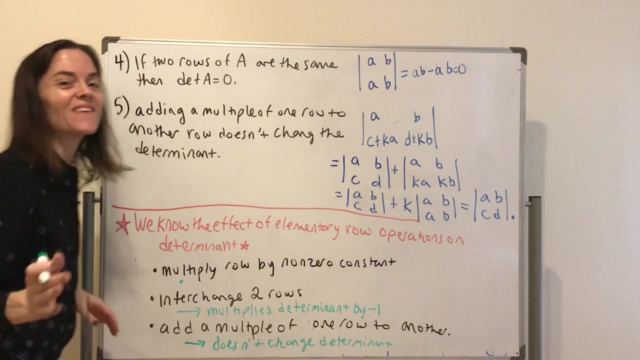 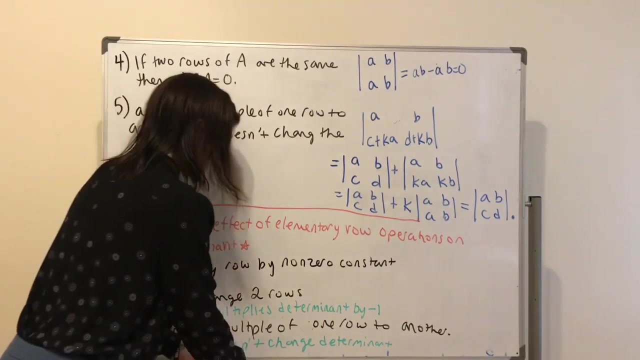 It does not change the determinant. So this one doesn't change the determinant. This one multiplies the determinant By minus one And finally, or firstly, depending on which way you read this one, well, this multiplied. let's see, I've got to give it a name. 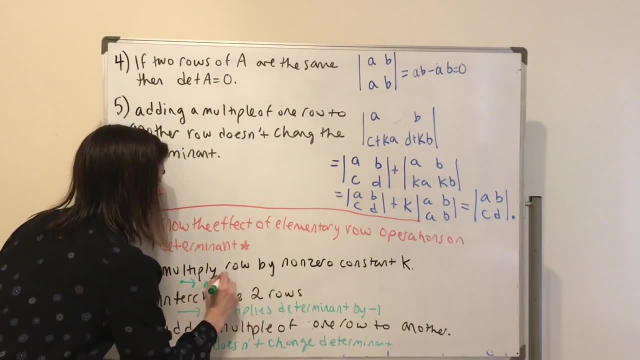 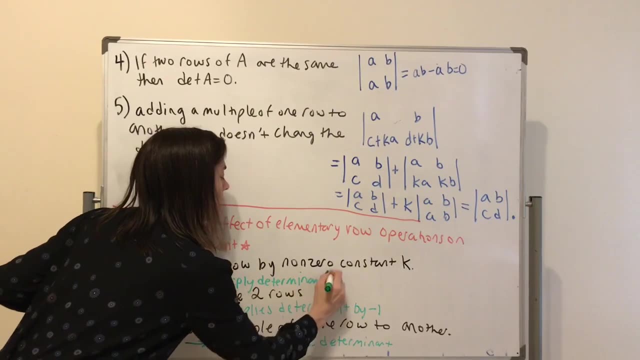 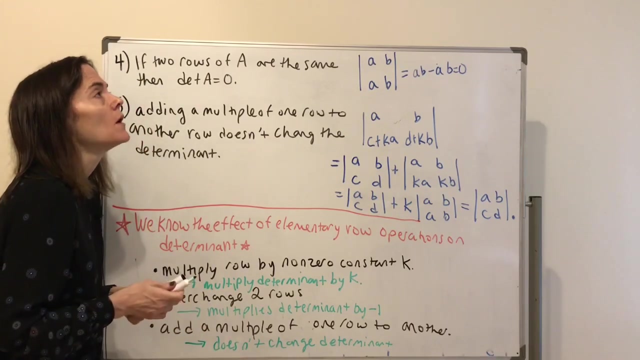 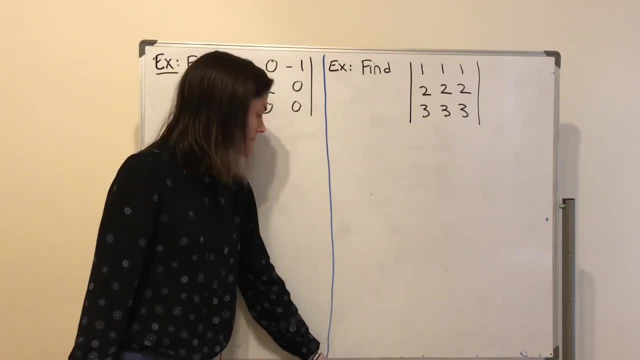 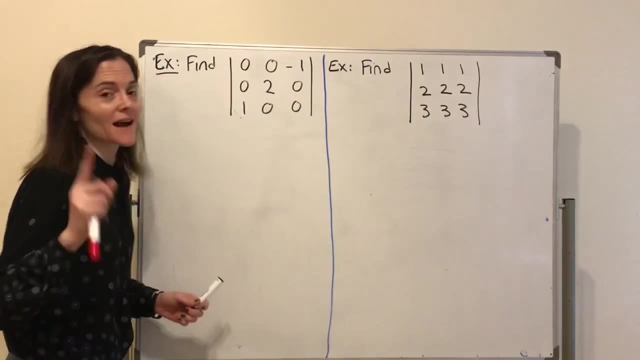 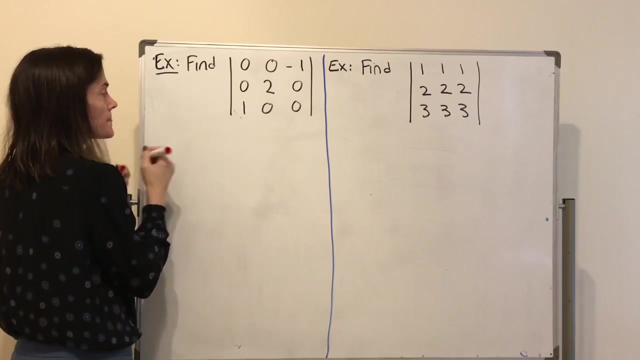 Let's perform some elementary row operations. So let's look here at this one. This one, we can keep track of what we do and get ourselves to the identity. So the first thing I'm going to do, maybe I will write a little bit. 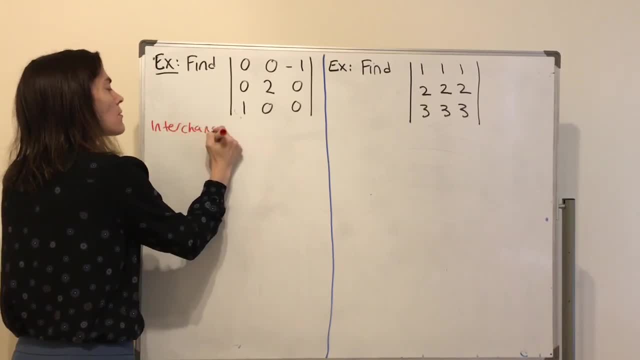 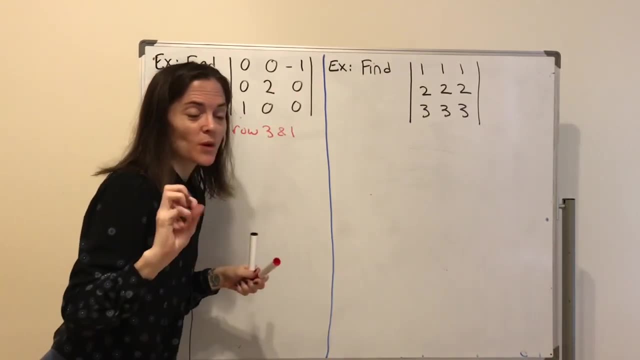 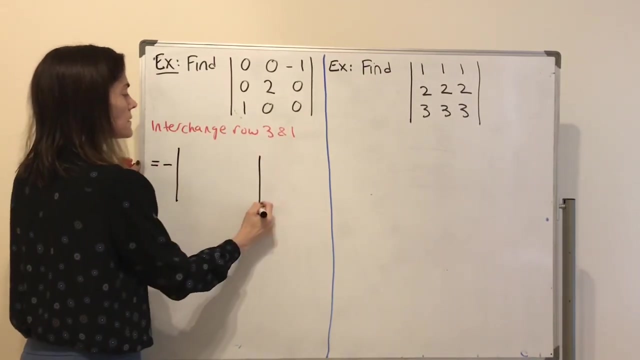 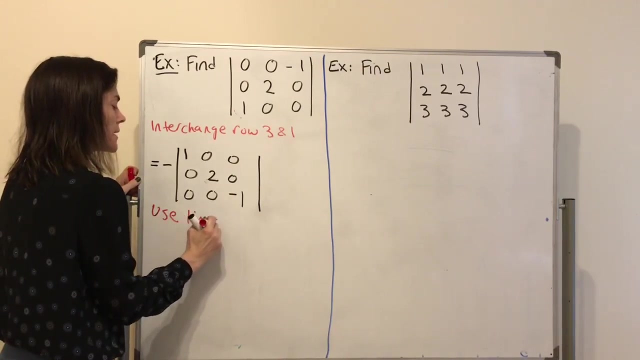 I will interchange row three and one, And we know what happens here. Multiplies the determinant by minus one, So this determinant equals negative. this determinant Where I interchange these rows- And I'm going to write this at the undetermined And I'll do a little bit of my own- 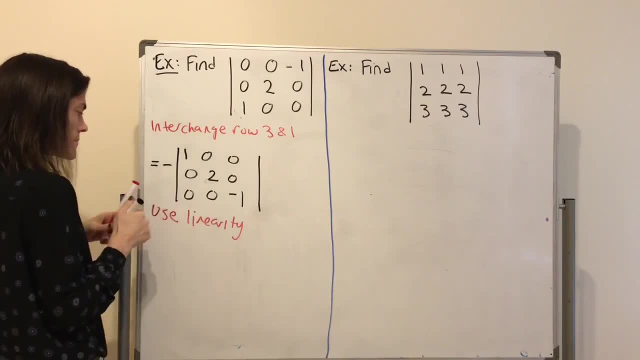 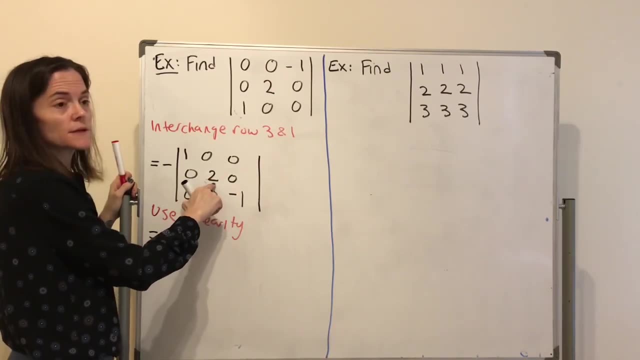 but it's going to be very important. Okay So, say, I have this set of two rows. Okay So I have this set of three rows, So I have this set of two rows, And now we want to get this one. 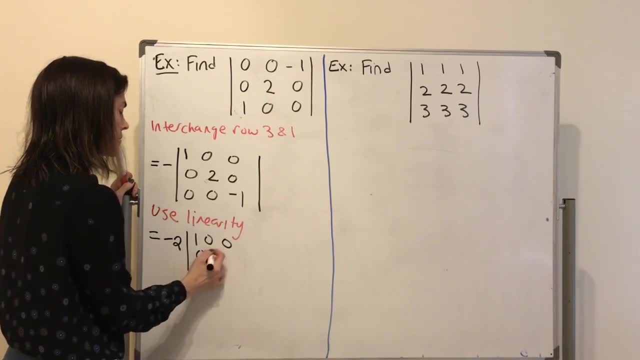 So we're going to write this one And then we're going to use linearity. Okay, Use linearity, Okay. So this is well, I have. this row is two times the row zero-one-zero, So this is going to be negative two times this determinant. 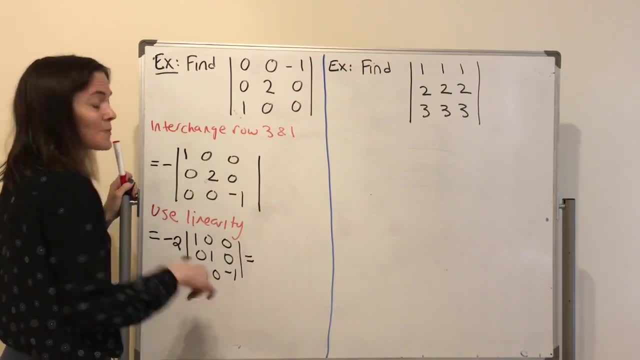 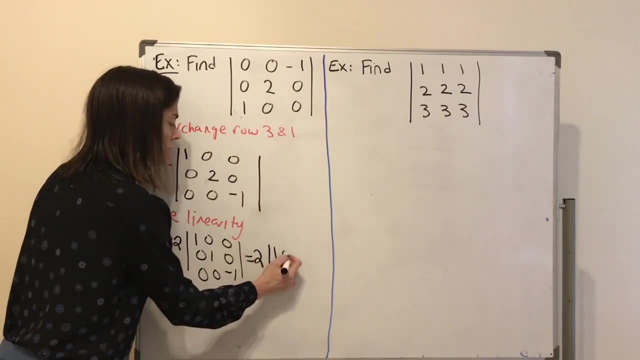 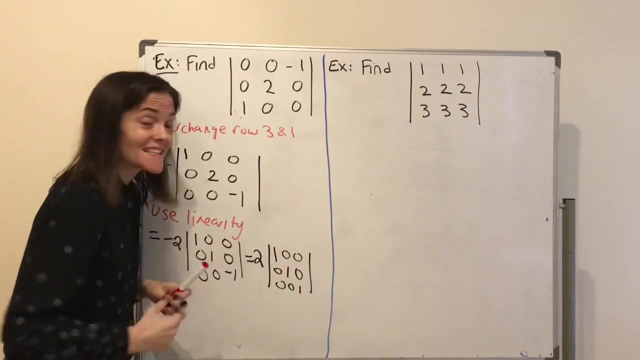 And now the bottom row is minus 1 times 0,, 0, 1.. So this is positive 2.. Just multiplying that by minus 1 times this determinant, This is the determinant of the identity. So now we have here 2 times 1,, which is 2.. 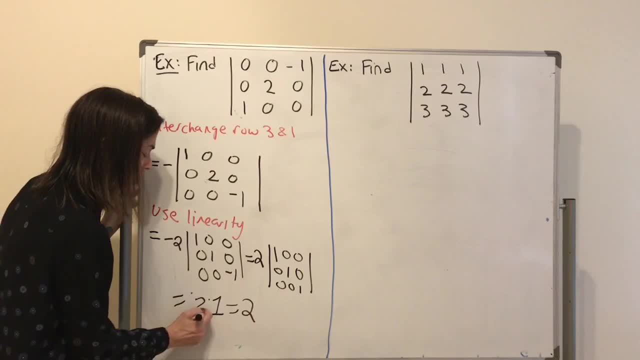 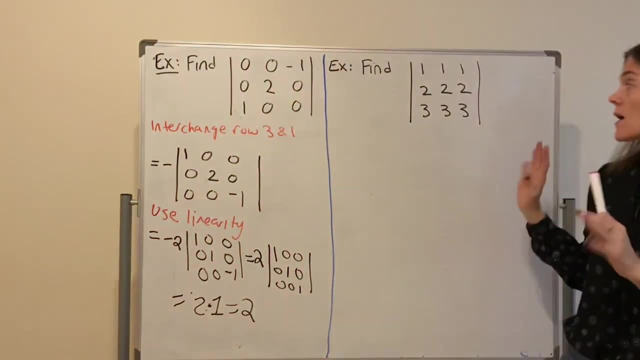 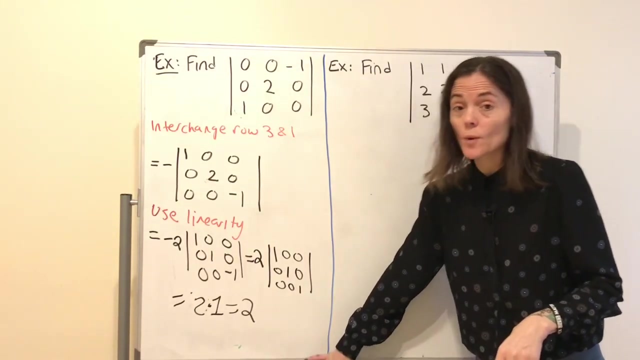 Okay, very good, We have found our first 3 by 3 determinant. Now here, hopefully, you can look at the matrix and say, Oh, I know. immediately the answer is 0, because this matrix is not invertible. This is a rank 1 matrix. 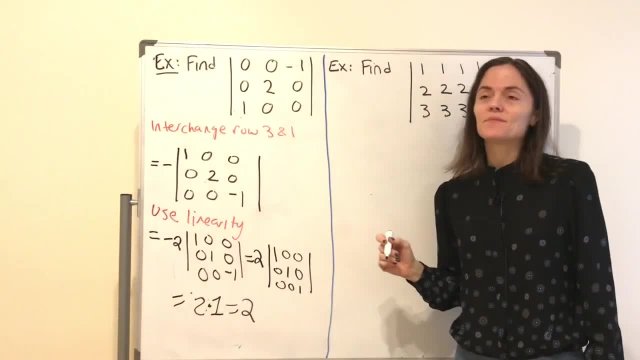 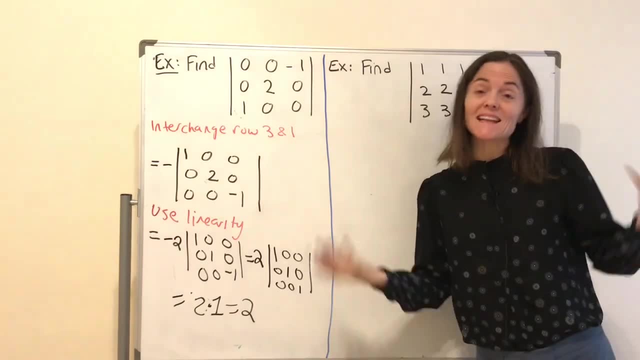 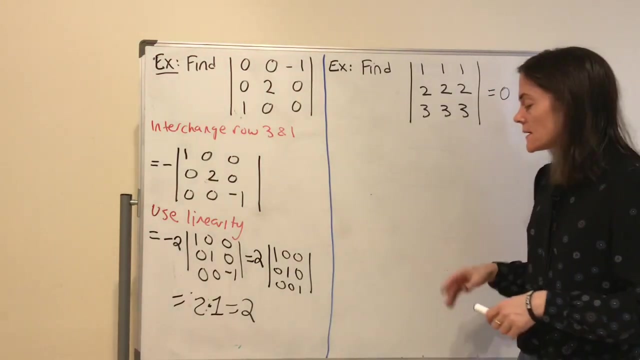 Every column is identical And I mentioned that the determinant is 0.. Well, the determinant is 0 if, and only if, the matrix is not invertible. Or it's non-zero, if, and only if, the matrix is. But okay, so this is the answer. 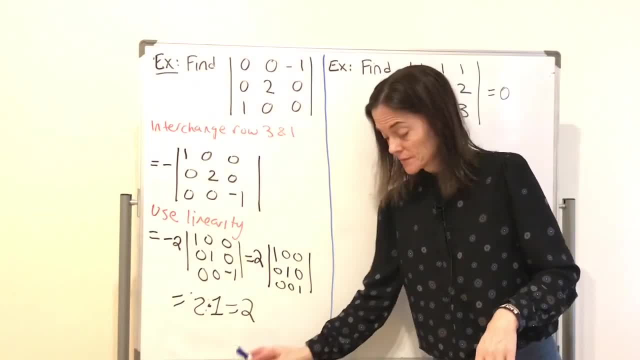 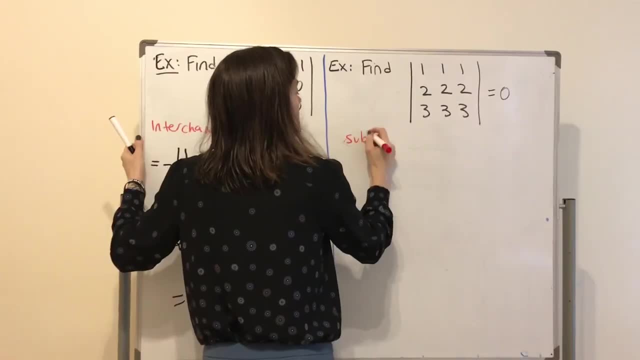 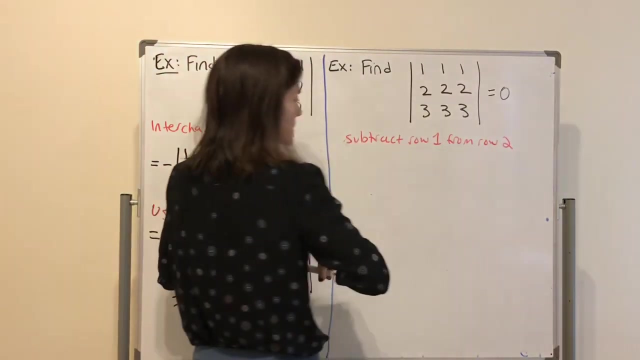 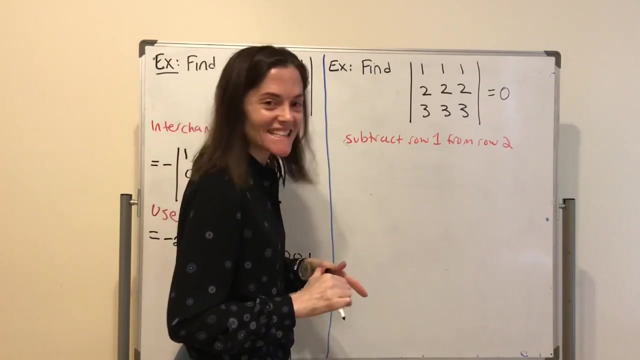 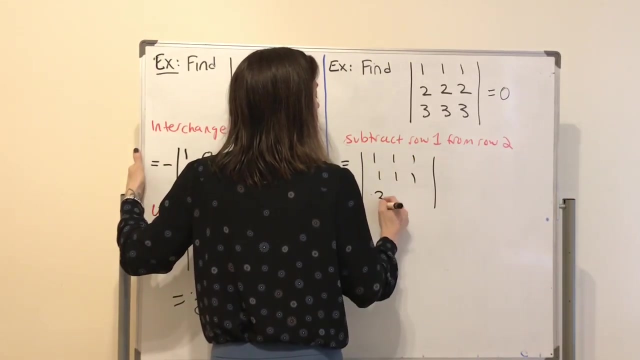 But if you want to see it with elementary row operations, through that process we can subtract row 1 from row 2. And we get the following: Adding a multiple of one row to another does not change the determinant. So we would have this: equals this determinant: 1, 1, 1, 1, 1, 1, 1, 3, 3, 3.. 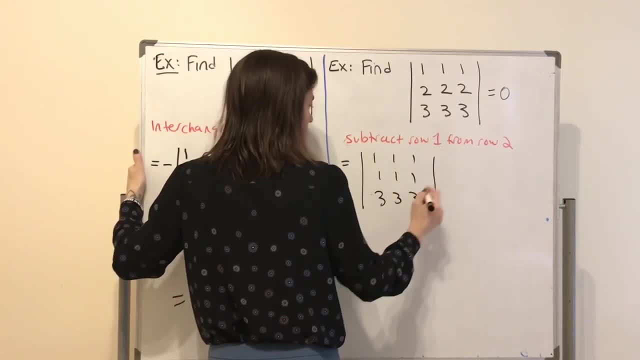 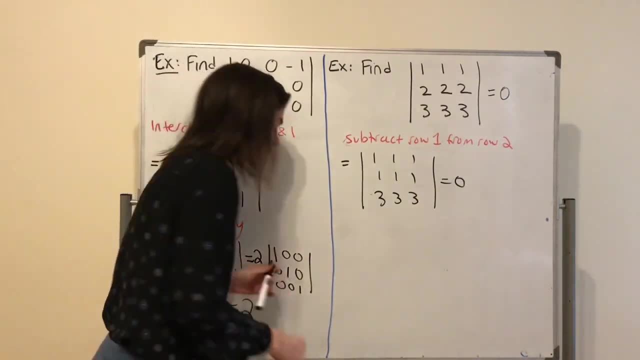 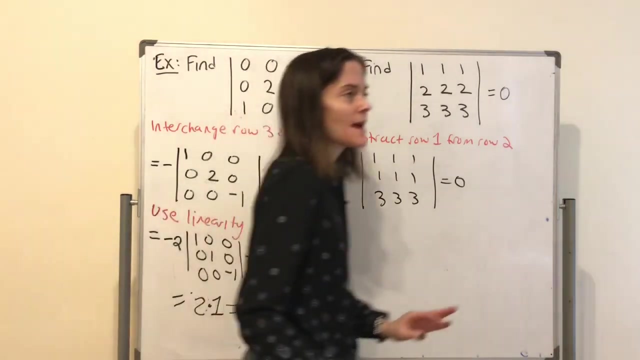 And now two rows are the same, The determinant is 0.. Something like this. So this is this idea of using row operations. Now let's do a few. Oh no, maybe I'll make one more comment And then we'll do a few that are seemingly more abstract. 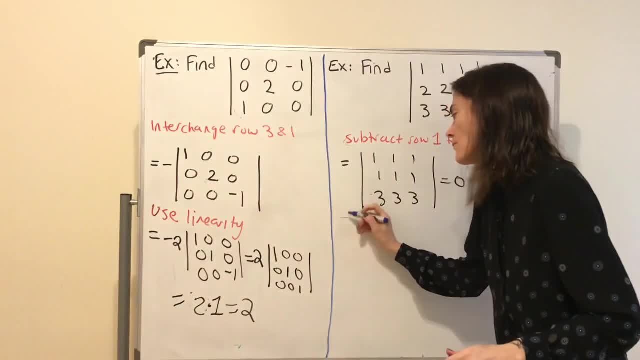 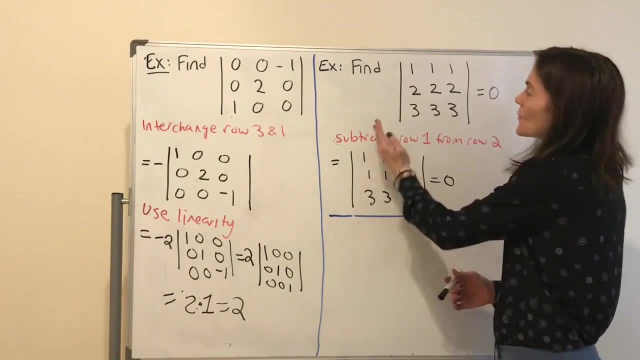 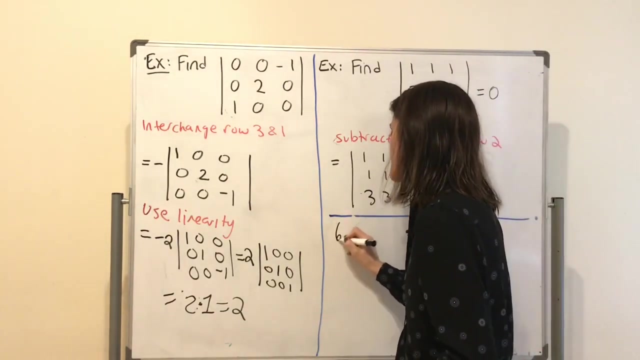 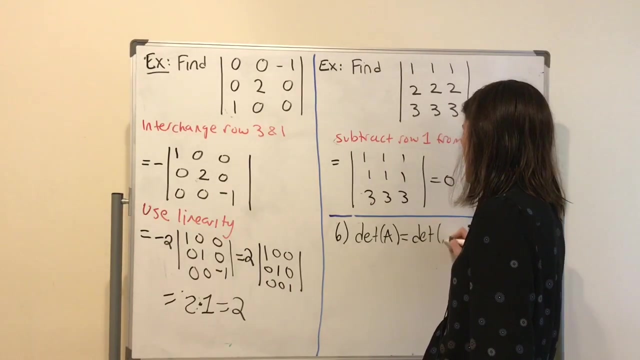 But they're just using the exact same thing. I'd like to mention a sixth property now, which is sort of motivated by looking at this matrix, And that's the following: So property 6 is that the determinant of A is equal to the determinant of A transpose. 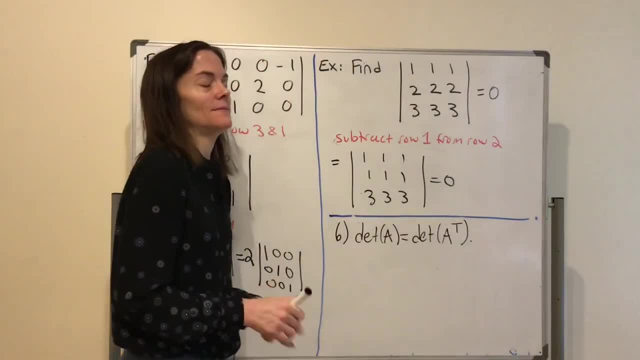 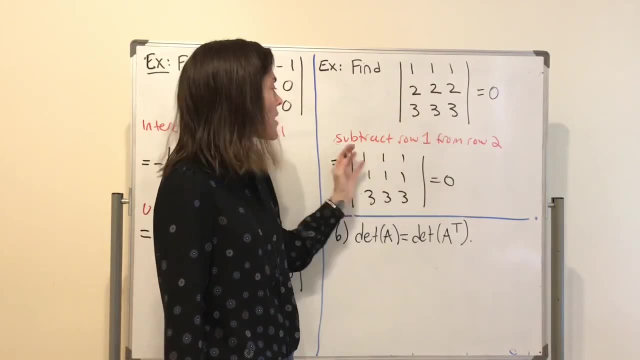 So what does this mean? And then I'm going to do something a little bit more abstract in a moment. What does this mean? What does this mean? Well, the reason why this example motivated it is because, I already said, one property was: if you have two rows that are identical, then the determinant is 0.. 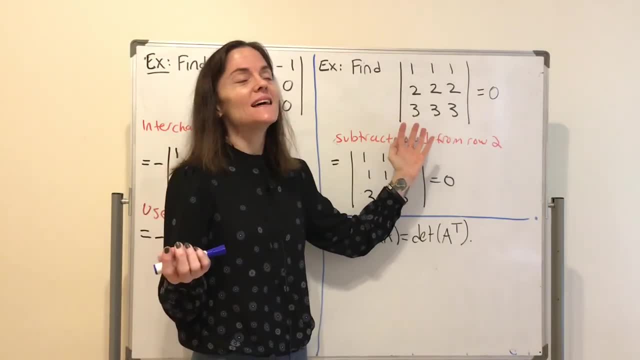 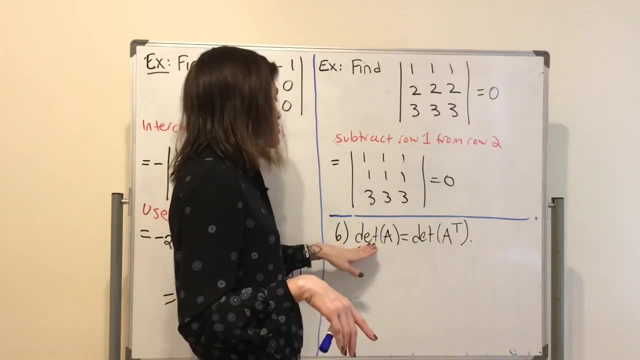 Well, you look at this and, as we see it, doesn't have two rows that are identical, but we do have two columns that are identical. OK, This property, that the determinant of A is equal to the determinant of A, transpose. 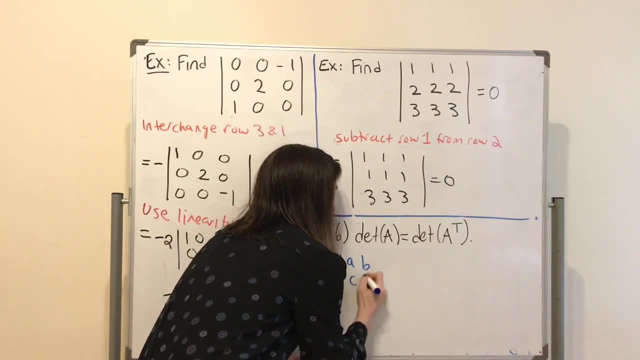 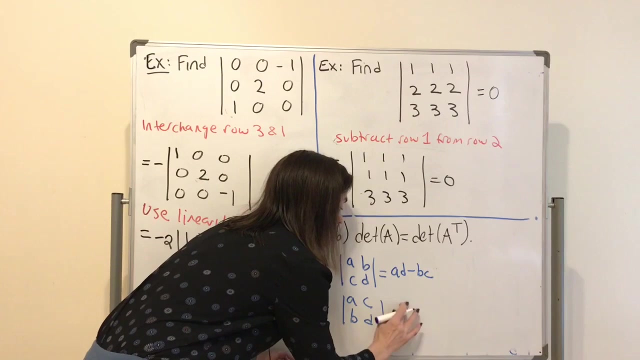 I mean certainly, we can, just as we did check it For 2 by 2, this is AD minus BC, and A transpose is this: We make this a row, and then we make this a row, and this is also AD minus BC. 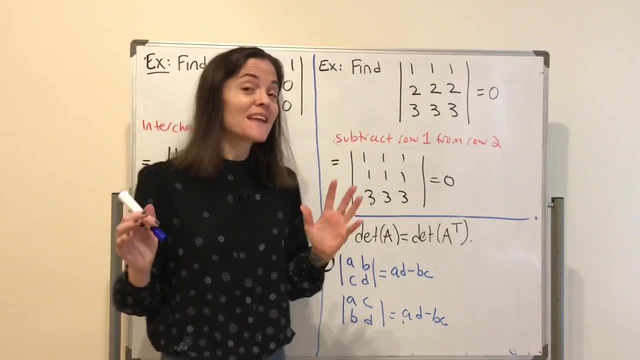 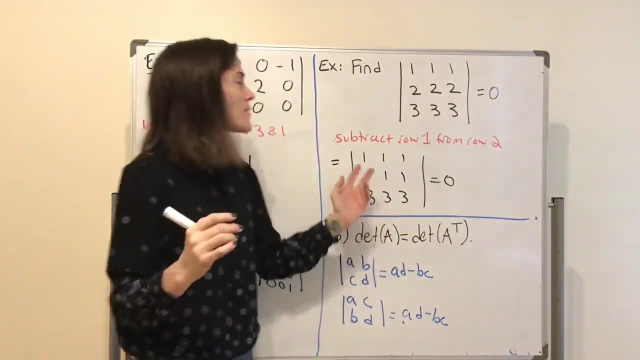 But what that allows us to do for larger matrices is we can also do things on the columns. So, for example, we'd look at this and say: oh, two columns. Two columns are equal Immediately. the determinant is 0.. 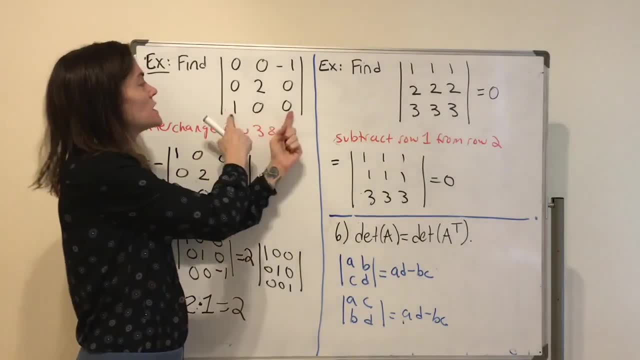 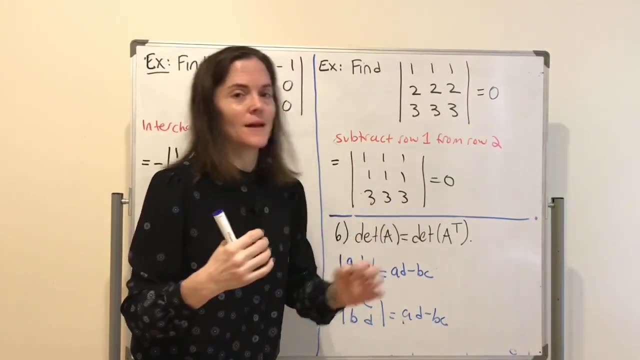 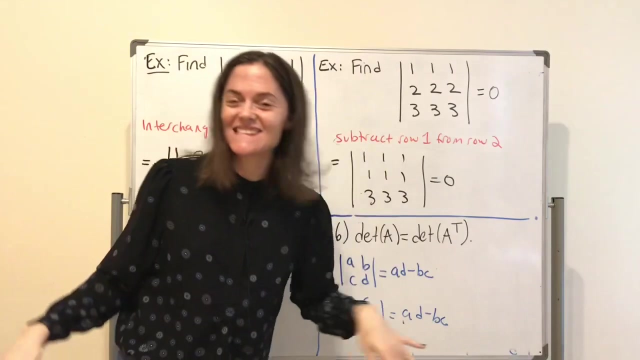 Or you could have started by interchanging these two columns, Or you take N and you multiply a multiple of one column And that will affect the determinant. by multiplying by that multiple K, say, It's a number. OK. 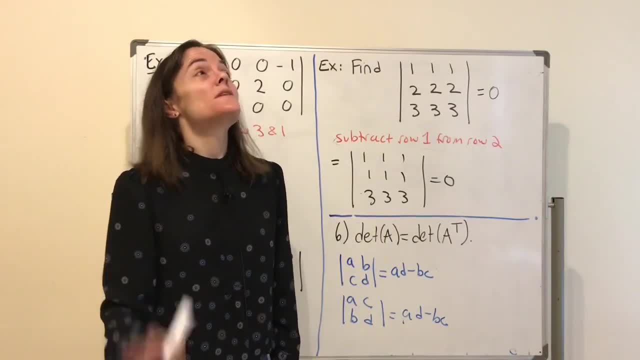 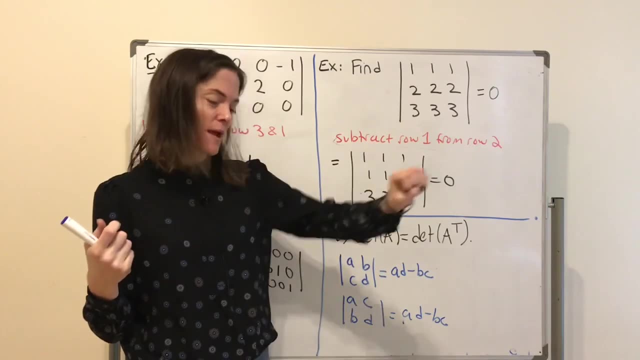 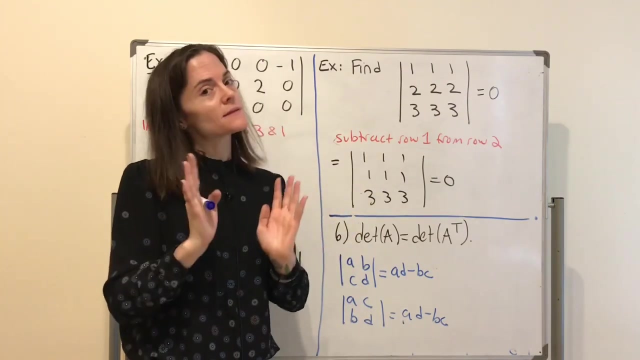 OK. So the determinant is this multilinear function Which takes in a N by N matrix, gives you a number right. That's a function. And it's multilinear in the rows, OK, But it's also multilinear in the columns. 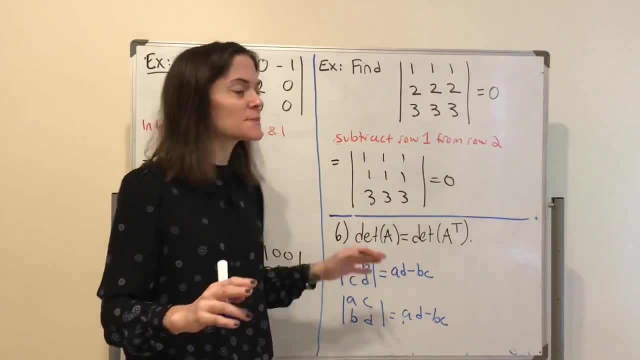 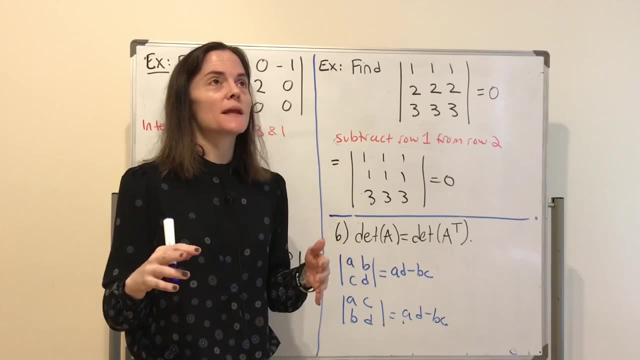 OK, Well, that was an observation I wanted to make, Just because this notion of either working with the rows or working with the columns, when we get into actually computing the determinant, it's going to be an important one. Well, here are a few examples. 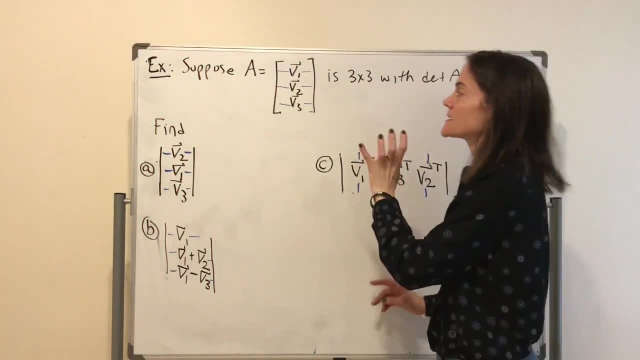 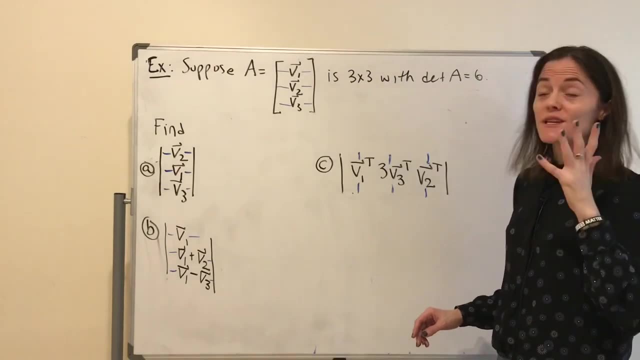 A, B, C, But they all start with this matrix A, And here V1,, V2, V3 are rows OK, And A is 3 by 3.. We are told the determinant of A is 6.. 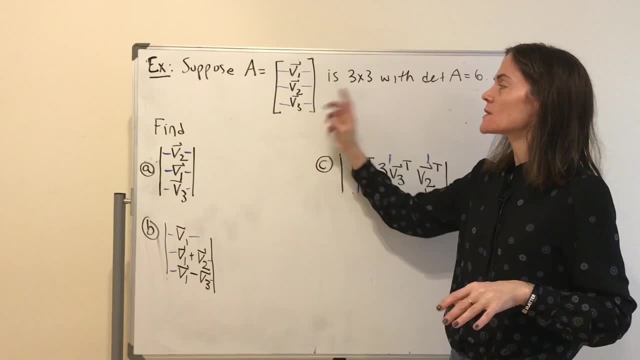 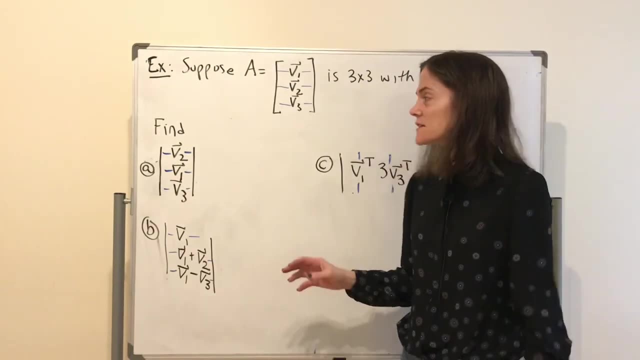 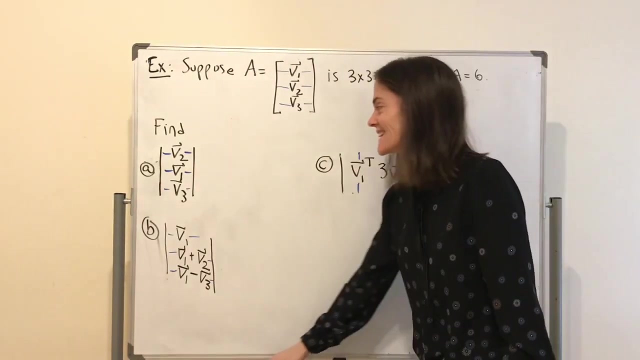 OK, So these are each vectors with three components in the rows- Very nice. And then we want to use these properties we have discussed so far to find the determinant of this, this and this. OK, Great, We're ready to do this. 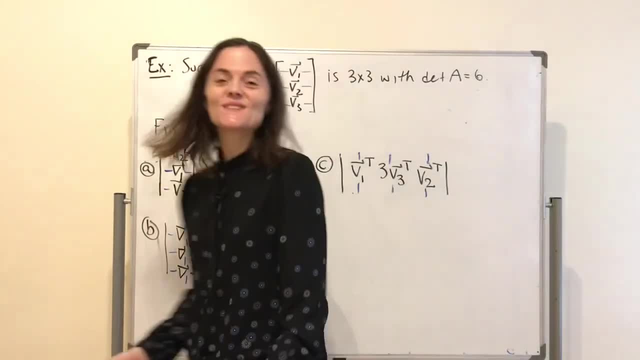 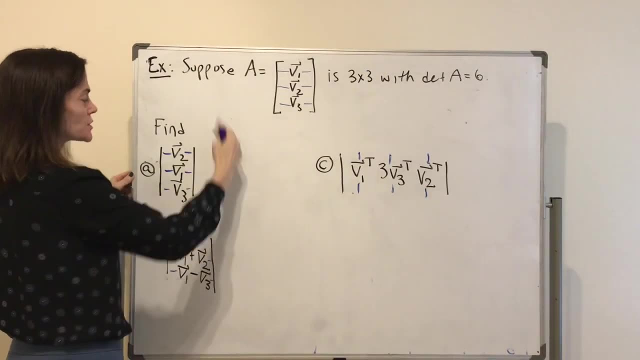 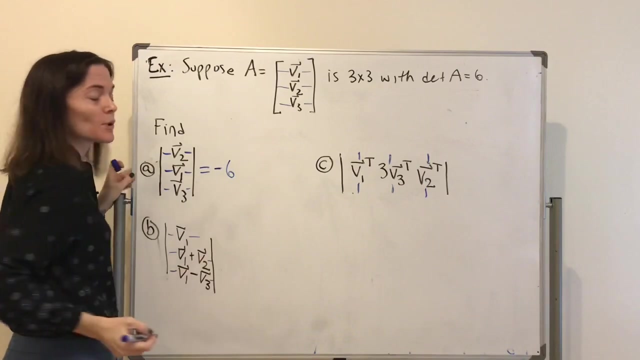 Well, Let's look at this first one. What's happened going from this matrix to here? Well, all I've done is interchange row 1 and row 2.. So this determinant is minus 6.. Multiplies by minus 1.. 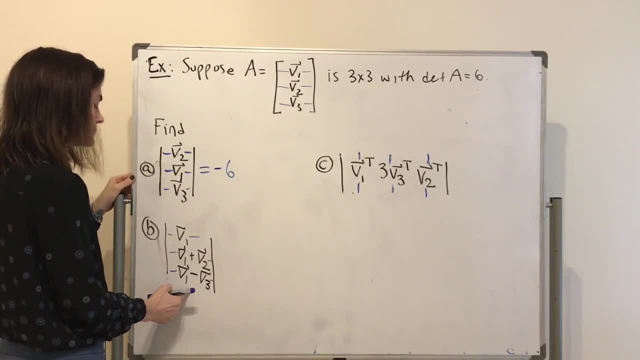 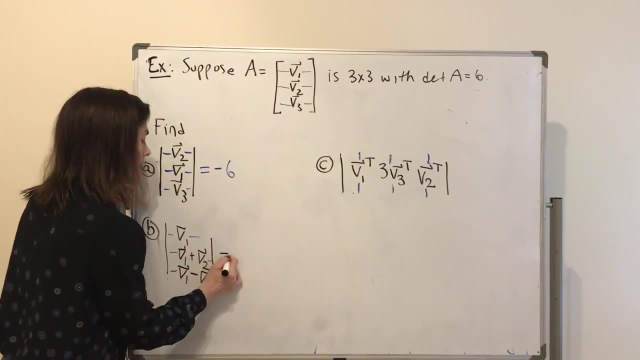 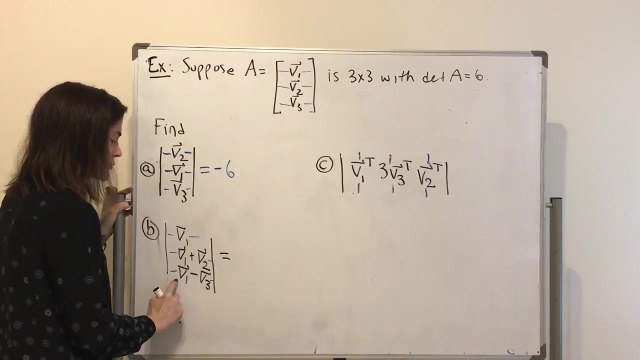 OK, What about this one? Well, let's do a few steps here. The first thing I can do to think about this is: I can take negative row 1, add it to row 2, and add it to row 3.. 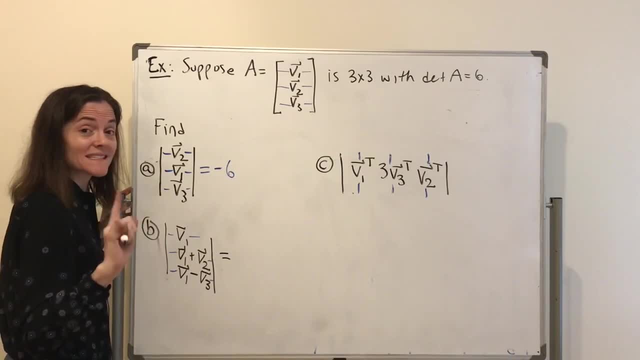 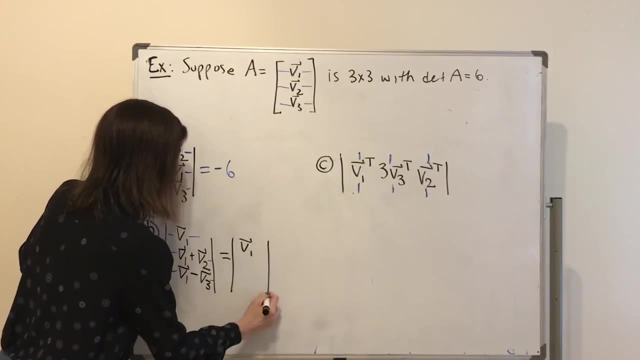 And this taking a multiple of one row and adding it to another does not effect the determinant. So this is equal to this determinant, Which has V1.. It has V2. And it has minus V3.. Oh, 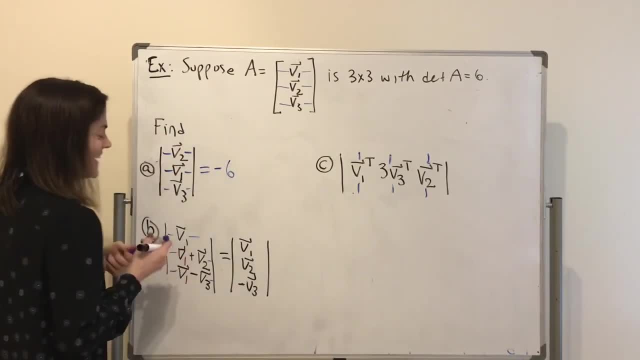 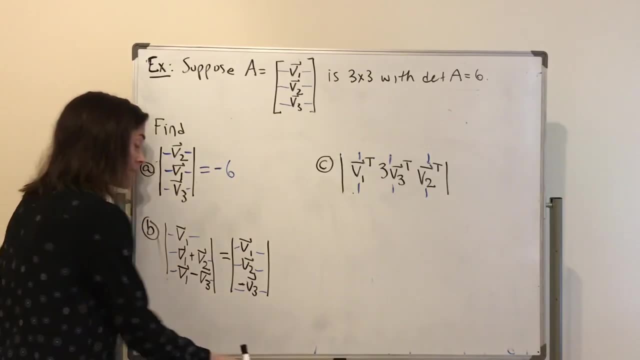 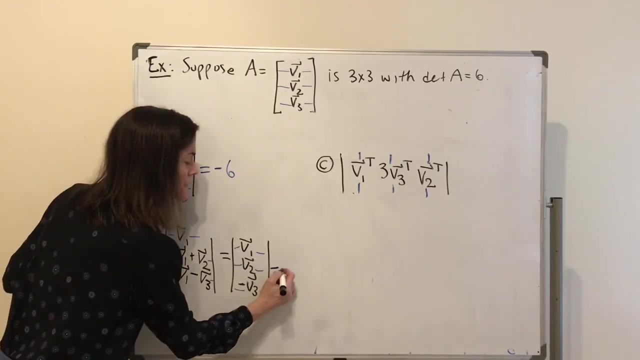 Oh, This should be a minus. And then, and then i have my blue things that illustrate it. they are rows. okay, very nice, okay, well, see this. now. we use the fact that the determinant is linear in each row, or what i was saying, multilinear, so this is just minus one. we pull out the minus one times the determinant, so this: 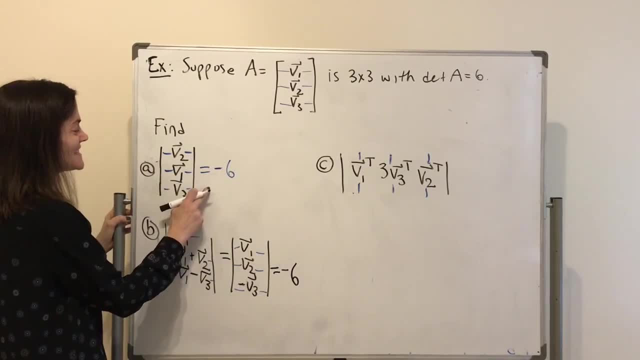 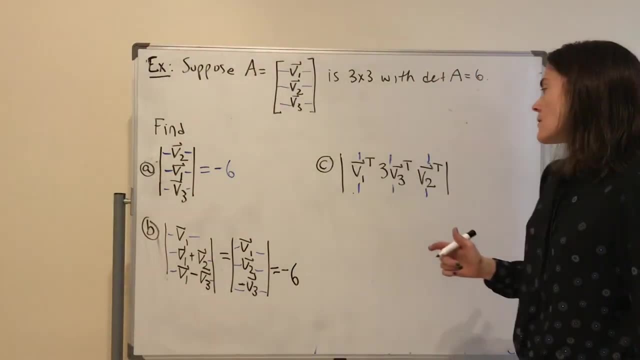 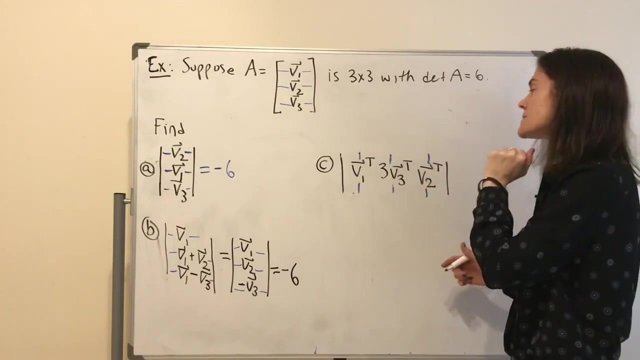 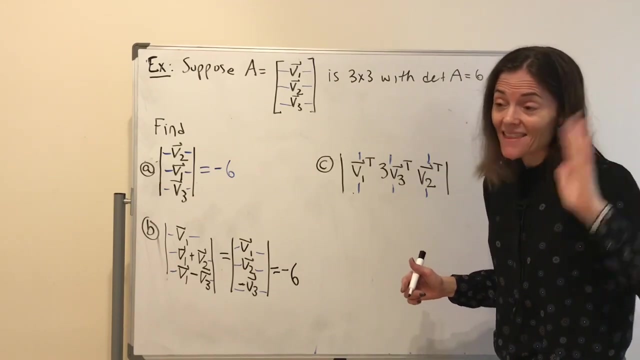 determinant is minus six. oh okay, it's the same one as the determinant here. so far, so good. now, okay. well, you see, these now have vectors as columns, and this is okay. we just talked about the fact that a matrix and its transpose have the same determinant and that we can work on columns. 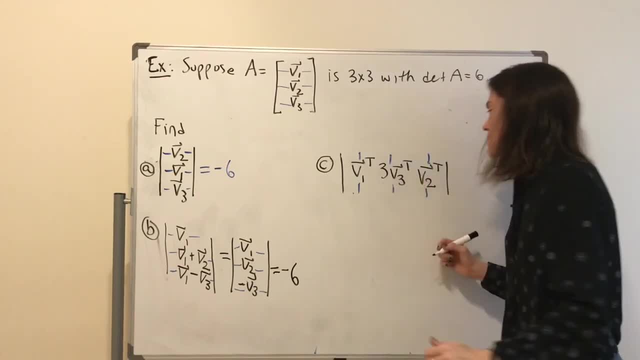 just as we could on rows, so this will be- let's do it in two steps. first of all, we have a multiple here, so this will be a single number, so this is a single number. so we have a multiple here and this will be a single number. so this will be a single number, so this will be a single number. 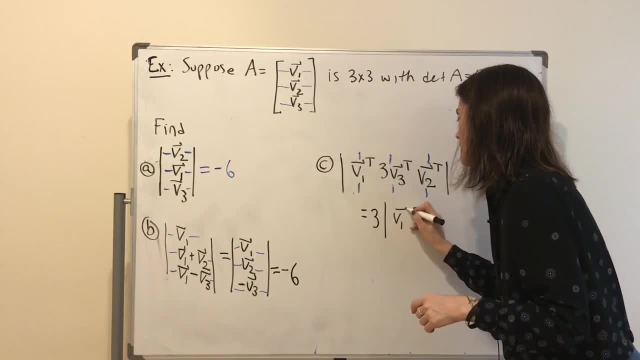 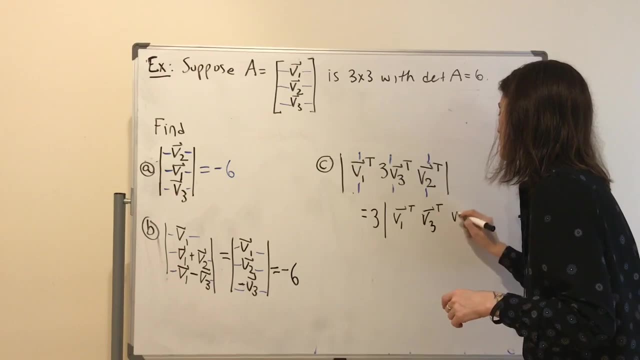 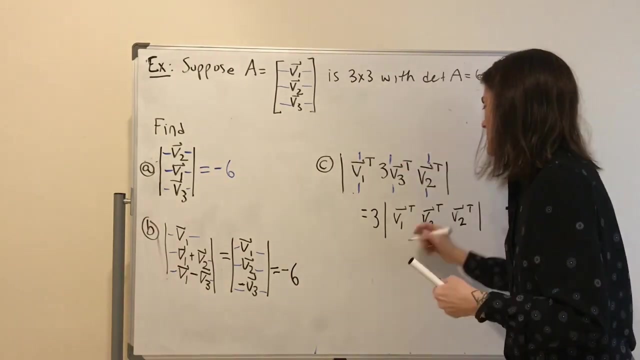 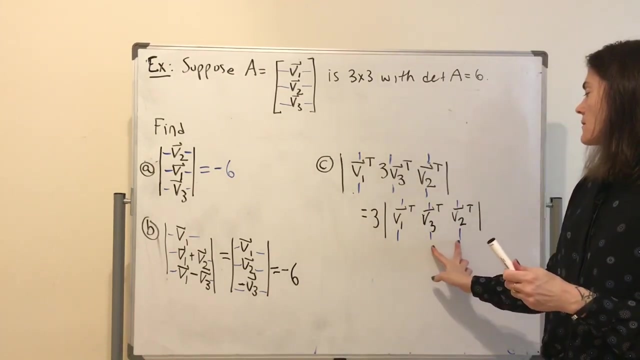 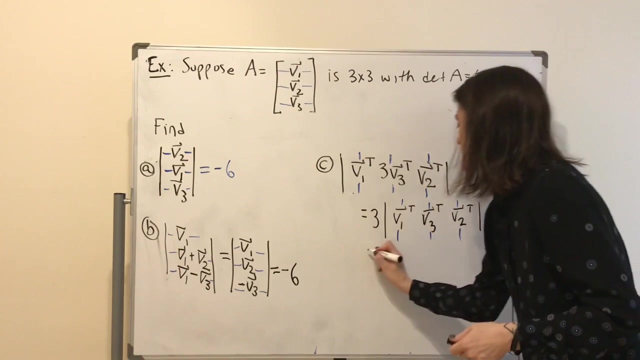 three times the determinant. here it's multilinear and the columns linear, in each column saying the same thing. okay, here are my columns and then interchange these two columns and you notice I will have exactly here the determinant of a transpose. so let me do this. this is minus 3 times this. 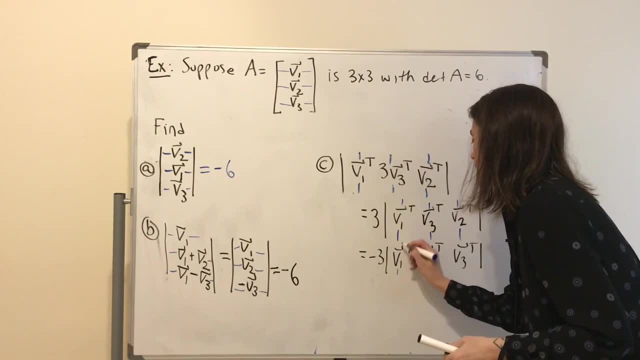 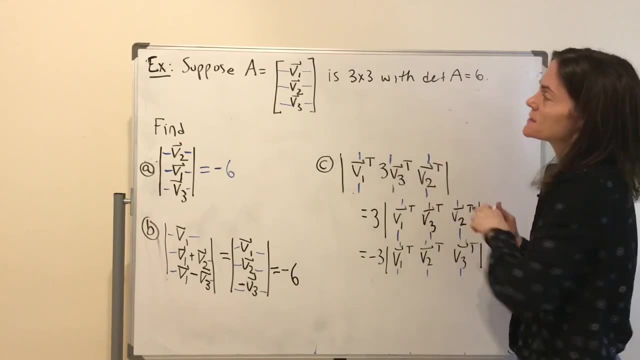 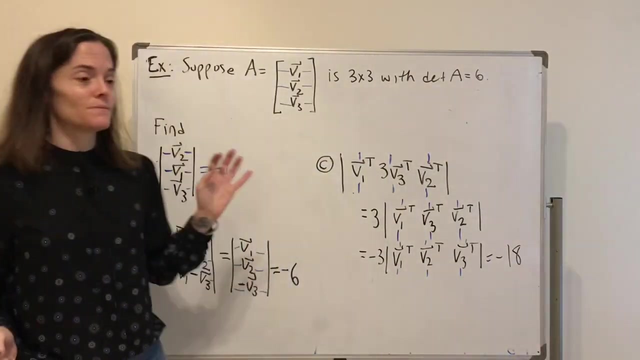 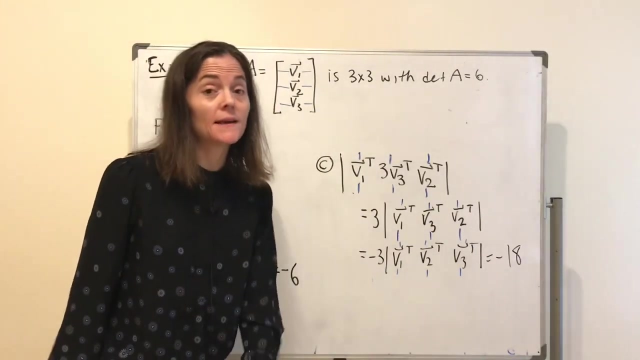 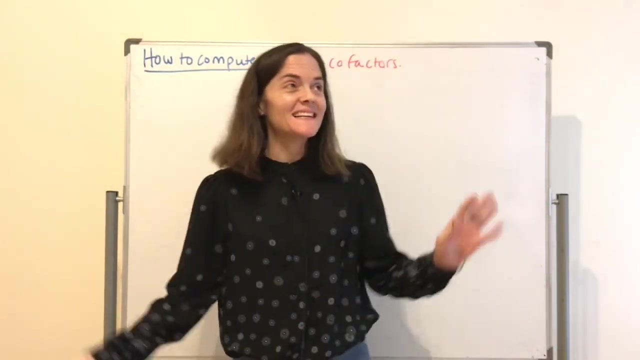 and okay, so this determinant is six, as they say marks determinant of a, so we get minus 18, and this is a nice exercise in this properties we have discussed so far, but now we want to move into. how do we compute a determinant for larger than a 2 by 2? well, now the question we've all been waiting for: how? 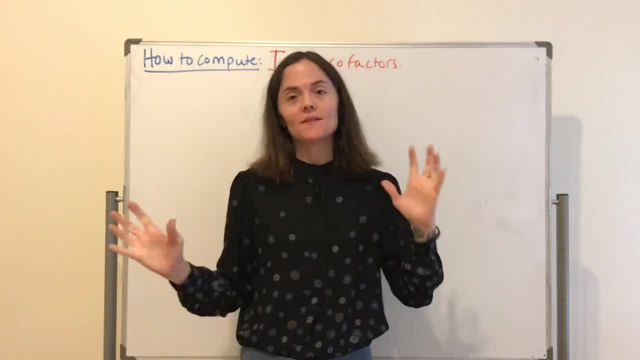 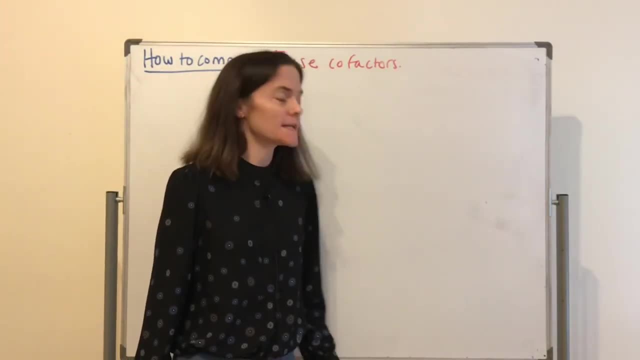 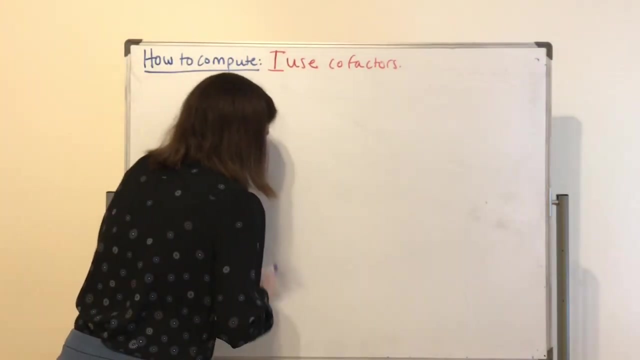 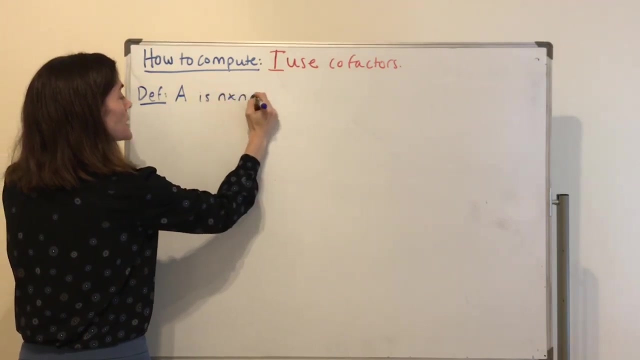 to compute a determinant of a larger matrix, and I will say I use cofactors. there's a few other ways that the book will mention, but we're going to discuss the cofactor approach. okay, but before I do let me begin with a definition. let's suppose a is n by n matrix and then a minor. 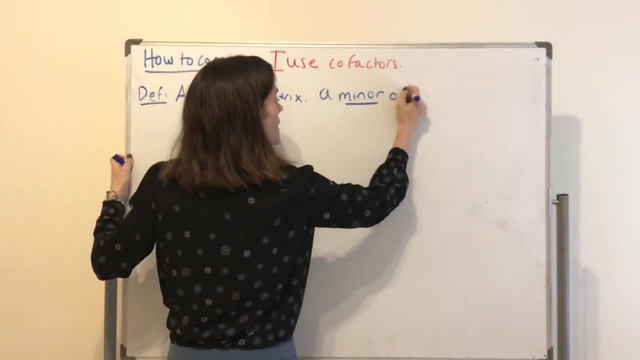 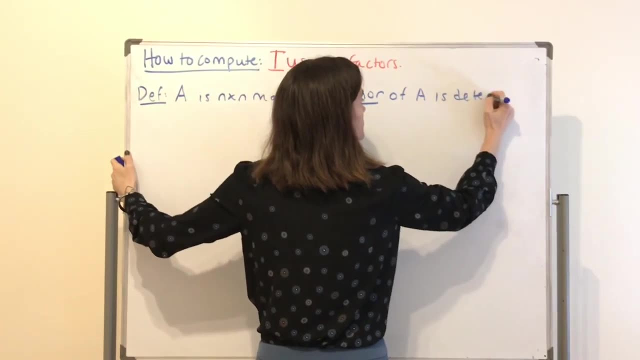 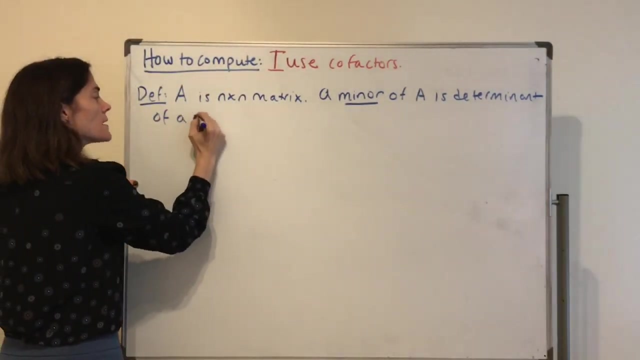 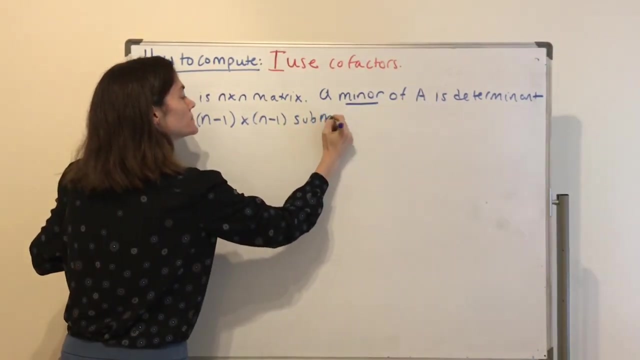 of a is a determinant of a n minus 1 by n minus 1 subnatrix, then I will call a N minus 1 by 11, which gives me j minus b. So what I've just done is I've shown zusammen, one by one, two by two, Mutter's Repeat with blah blah, blah In our English: 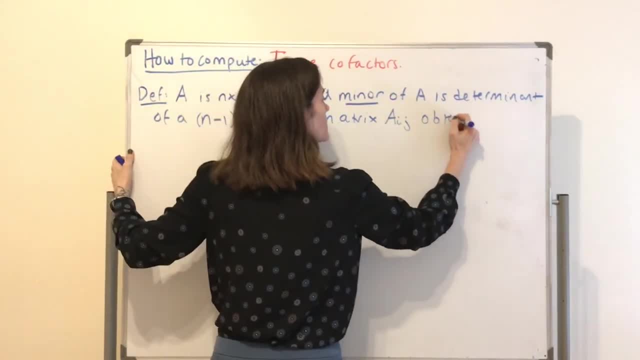 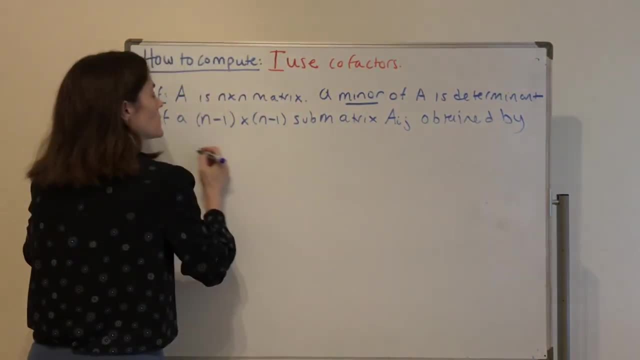 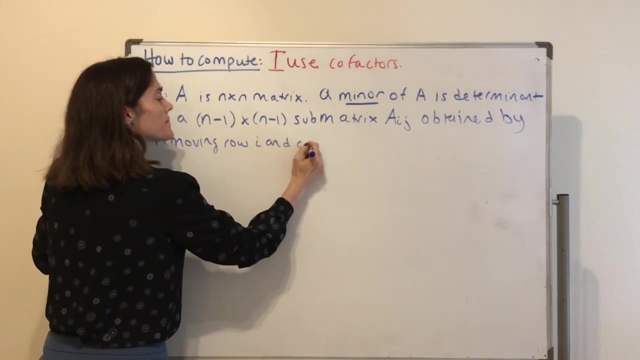 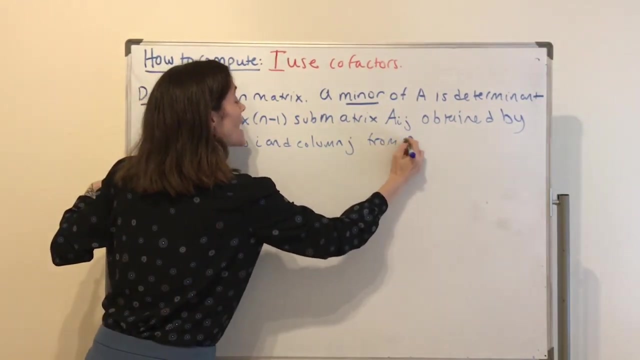 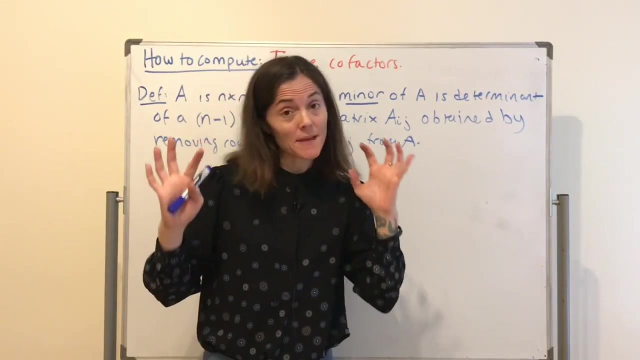 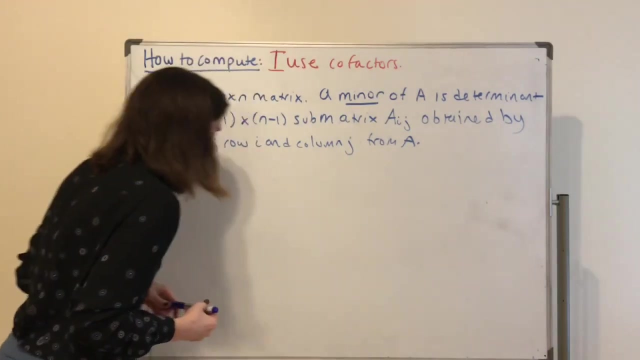 IJ, and this is obtained by removing row I and column J from A. So you have matrix A, You cross off row I, cross off column J. this gives you an N-1 by N-1 submatrix and its determinant is called a minor of A. 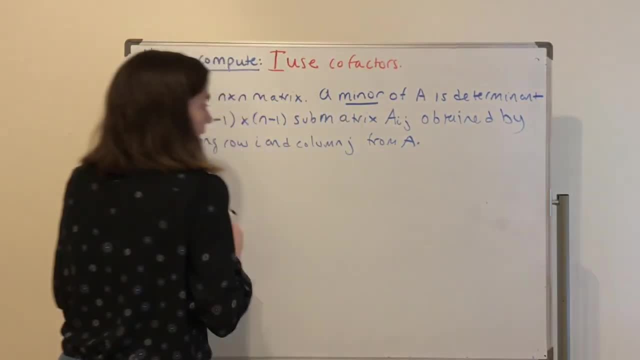 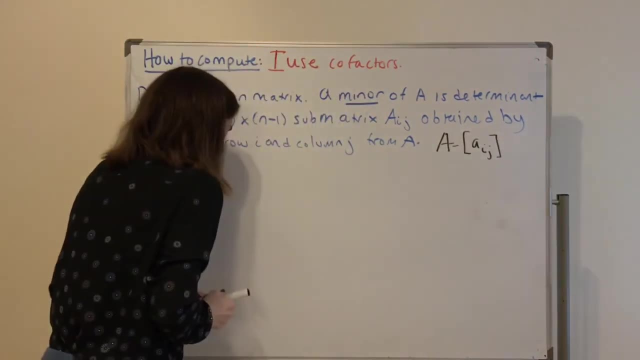 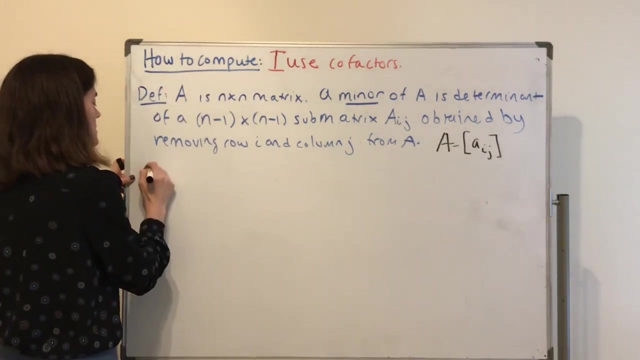 Now let's say the matrix A has IJ entry like this, Then we may write a formula for the determinant that has some minors in it. So we We may write: the determinant of A equals, it'll be A11, the determinant of A11, minus. 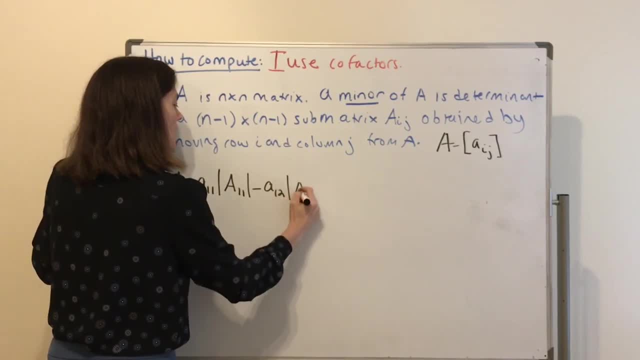 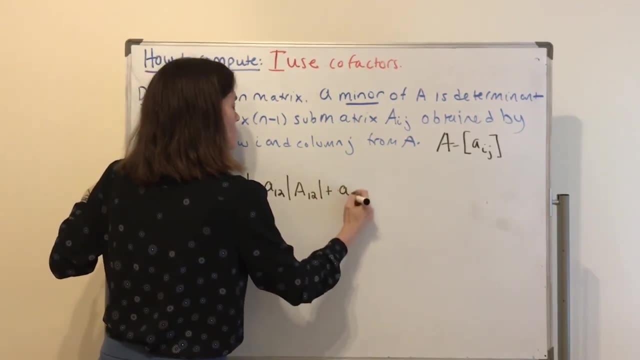 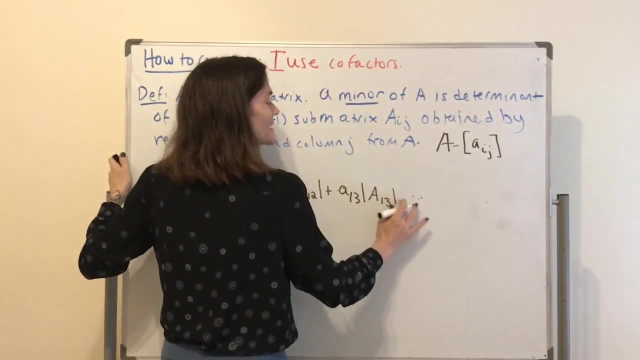 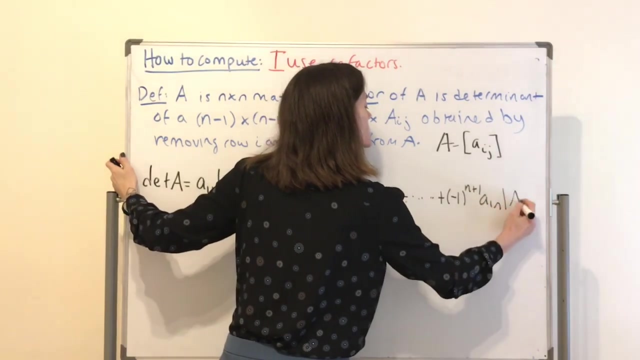 A12,, determinant of A12, plus. okay, I'll write- oops, I'll write one more before I do a dot dot dot- determinant capital A13.. And then the next one will be a minus, But then the very last one is a minus, one to the N, plus one A1N, and then this determinant. 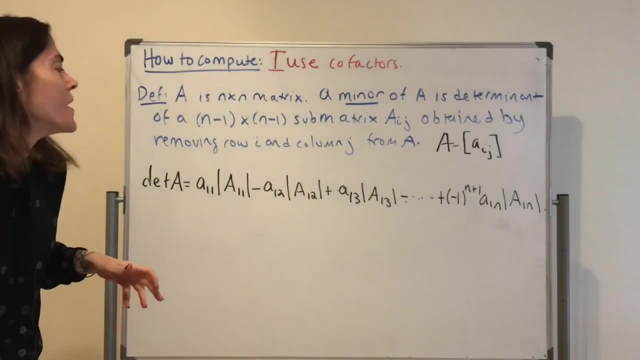 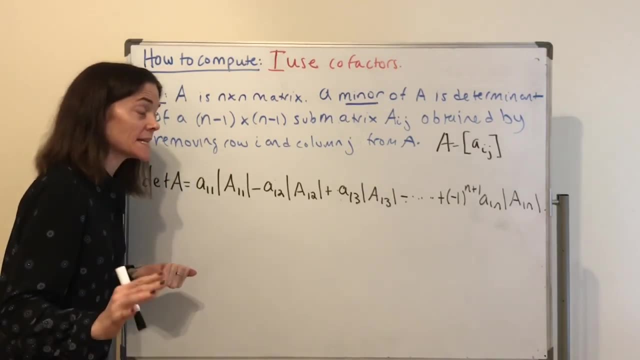 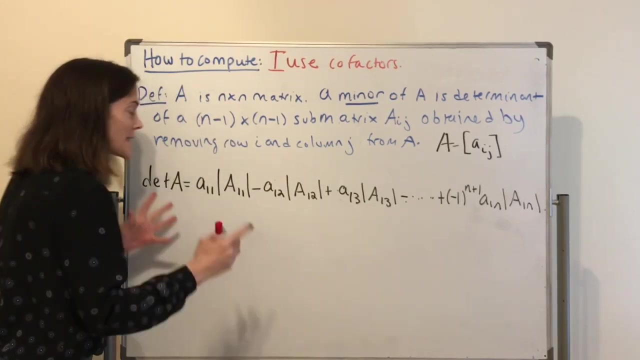 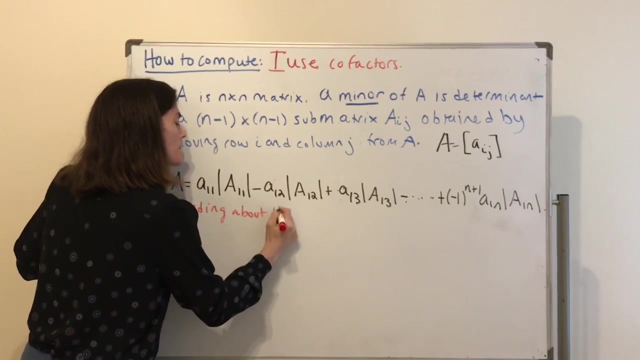 this minor Okay, Well, don't get scared, or something like this. It looks like a lot, but it's not too bad. So this is a special type of cofactor expansion. Again, this is expanding, So I'm gonna have to remember to put this: 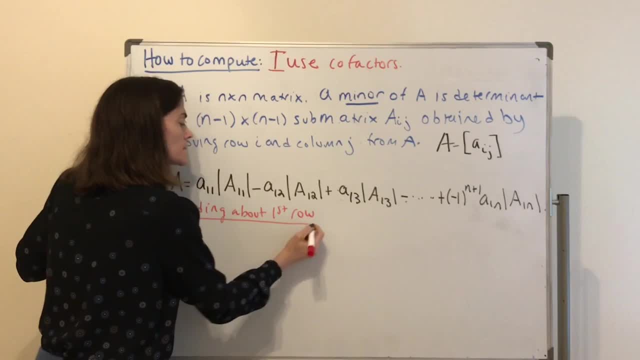 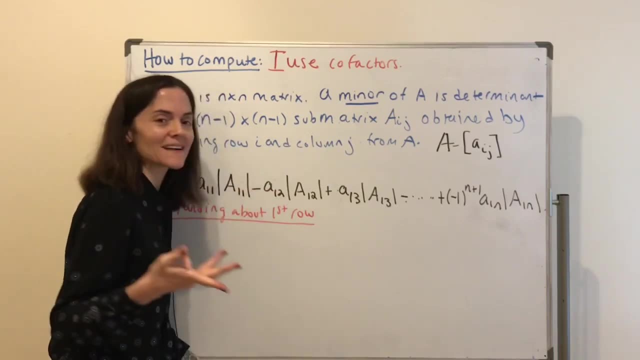 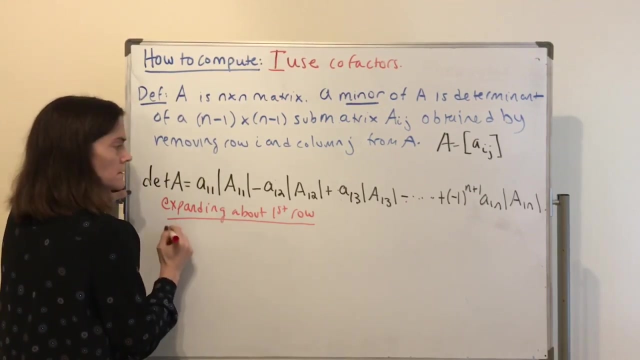 So we're gonna have to think about the first row. I will discuss momentarily that. this is not the only option for calculating the determinant this way. But what is the whole cofactor part here? Well, if you define C, maybe I'll do it here. C IJ is minus one to the I plus J times this. 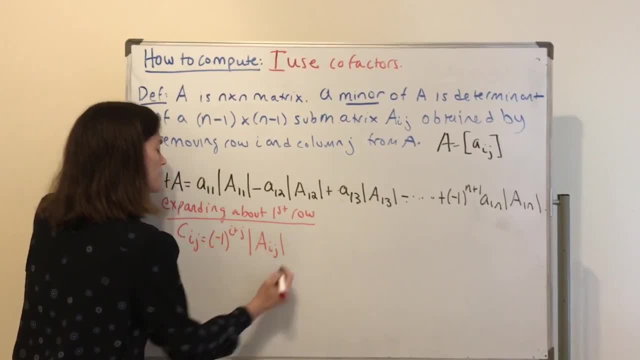 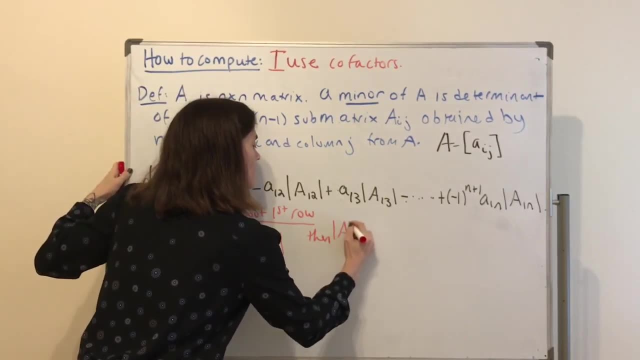 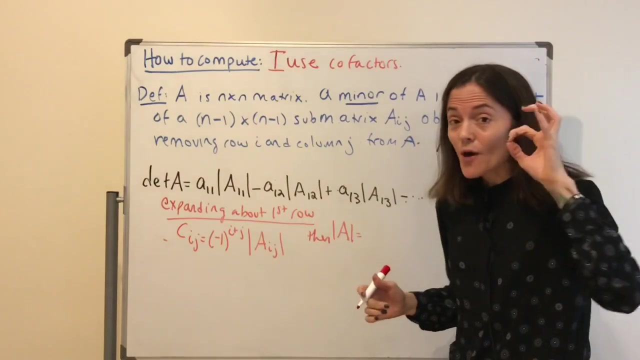 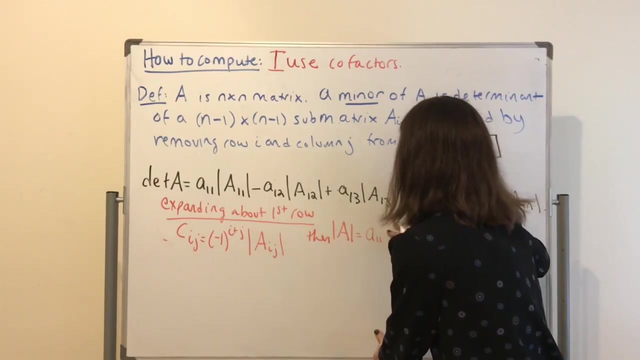 determinant And then the same thing. then you can write the determinant of A in terms of a sum. This is called the cofactor. The Cij is a cofactor. Okay, you can just write it as A11 plus C, oh, not plus times C11 plus A12, C12,. 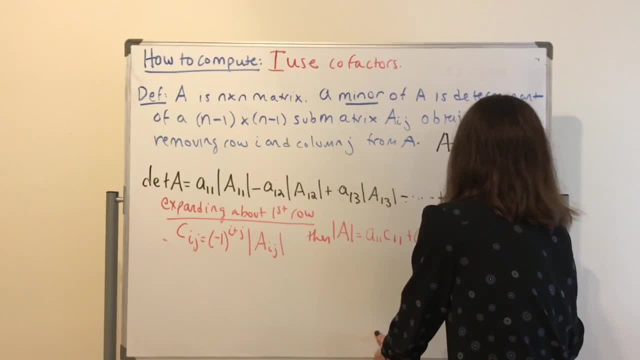 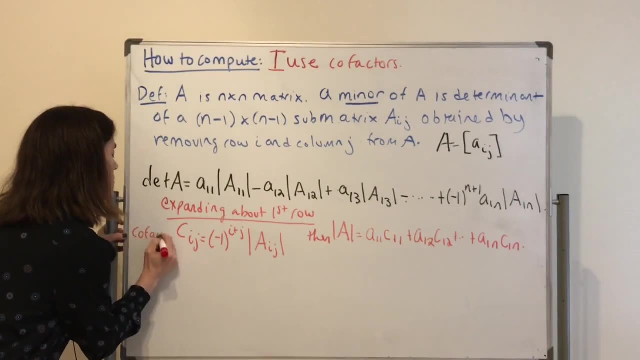 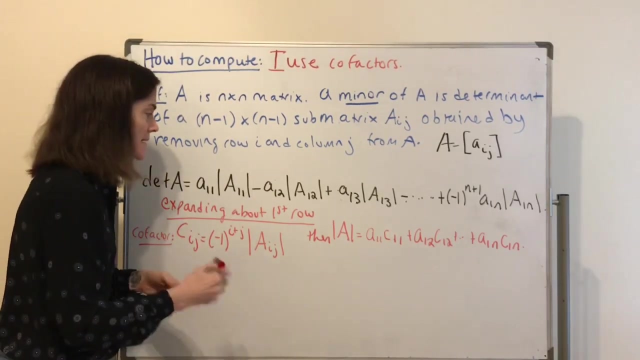 all the way out to A1N, C1N, like this: Okay, this is a cofactor, And this is just another way to write this exact same line here. Now let's look at this for a 3x3 matrix. 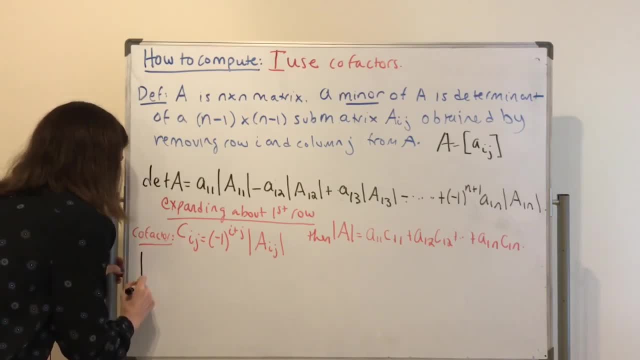 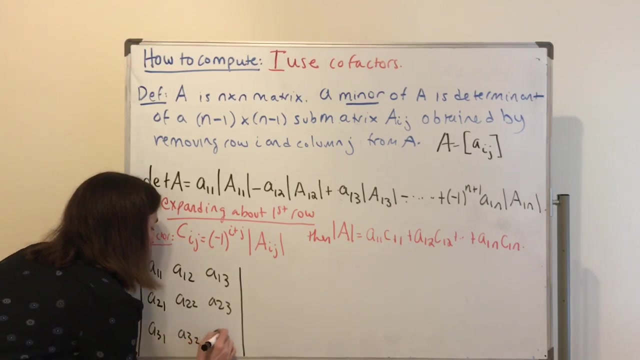 because this is where we can actually- it doesn't look like just so many indices- we can actually see these. We can actually see formulas. Okay, so if I have A11, A12, A13, A21, A22, A23, A31, A32, A33. 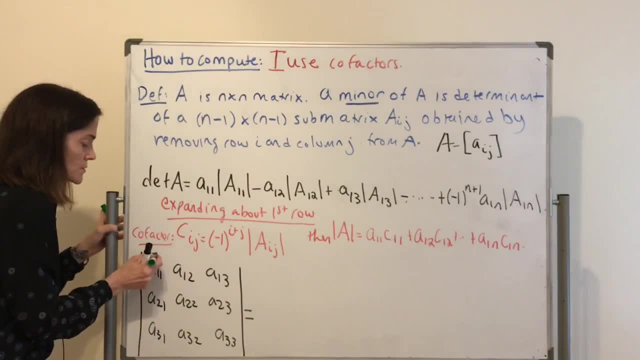 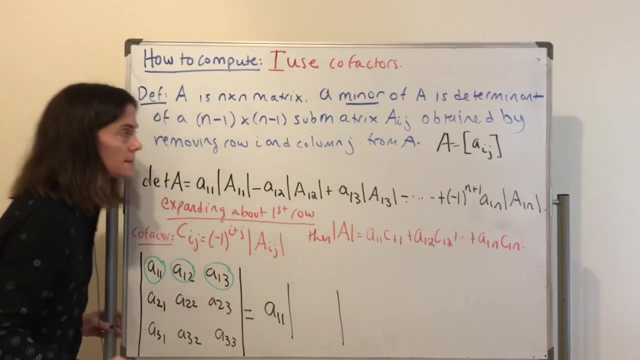 I'm expanding about the first row. Here's my first row. first row, first row. Okay, so this will be A11, and then we have this smaller determinant. okay, Here it's going to be a 2x2 minor. 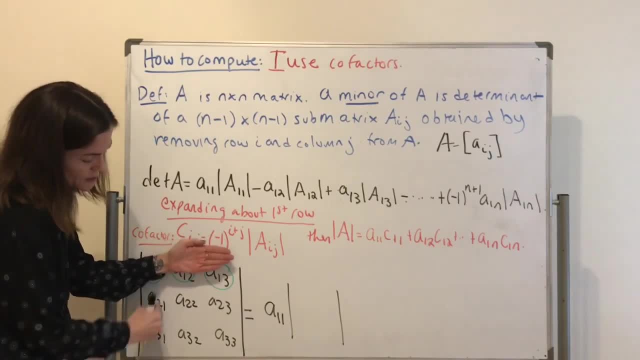 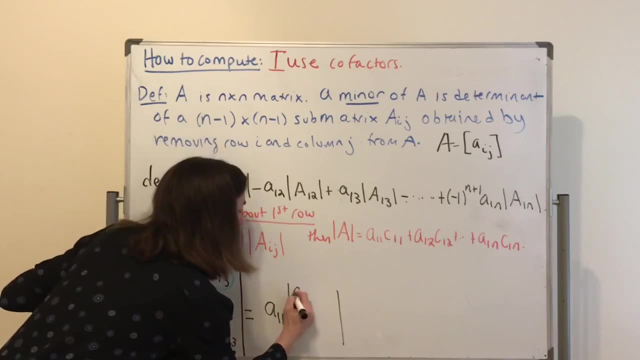 And look, you cross and you cross here. you cross these two off, Cross off this column, cross off this row and look you see, right, It's A22, A23, A32, A33.. And then it's going to be a minus A12.. 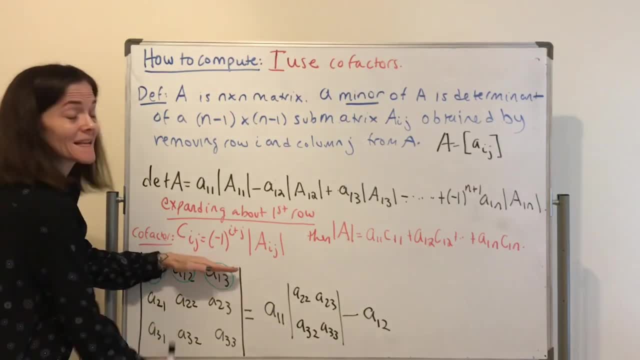 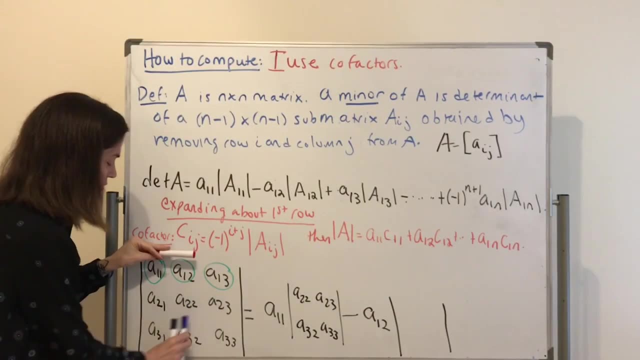 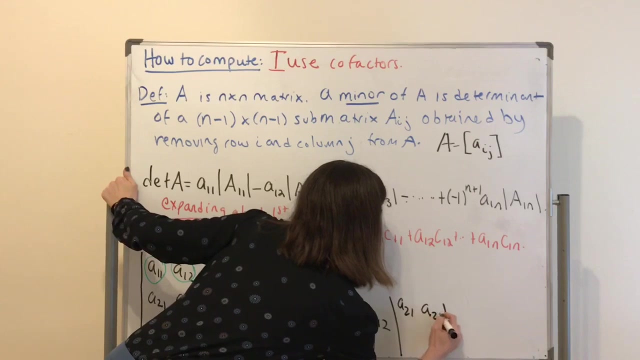 Okay, then we cross off the first row, second column, and we have another 2x2 determinant: A21, A23, A31, A33,. this is what it is: A21, A23, A31, A33.. 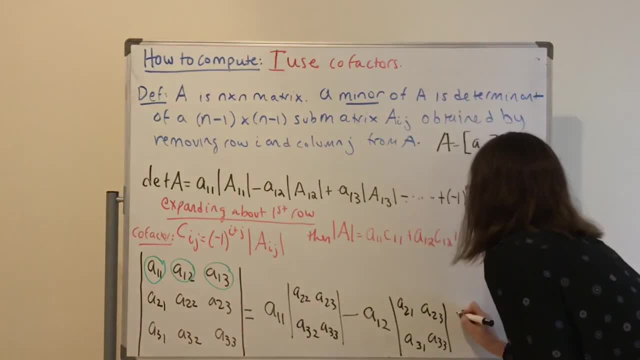 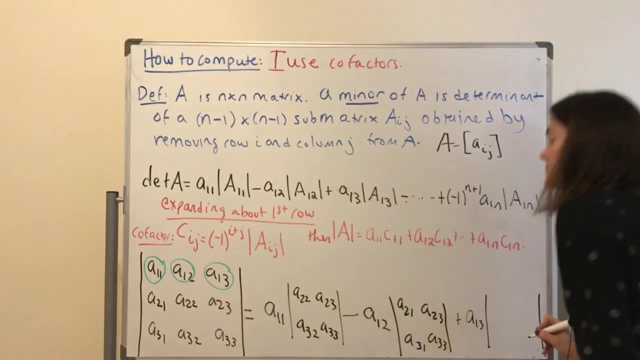 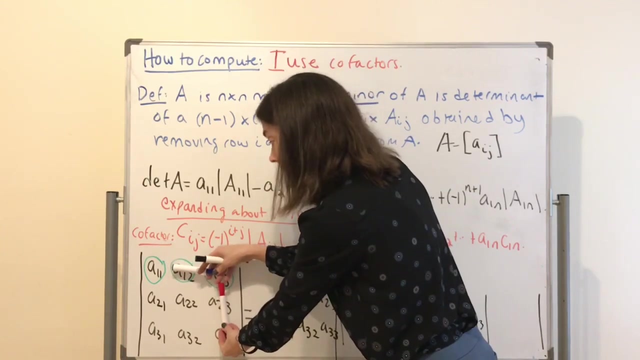 Okay, and then it's plus here A13, and we have one more 2x2 determinant where we cross off this row and this column and we see the 2x2 right there: A21,, A22,, A31, uh-oh yeah, we're okay. 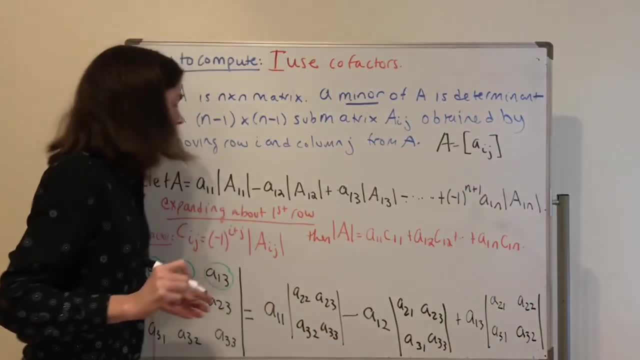 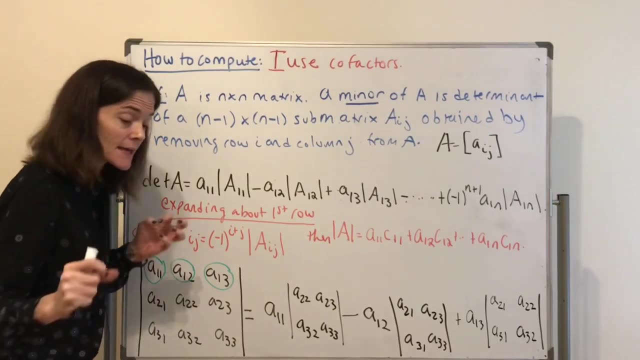 A32,. so this is the formula for a 3x3, but it's exactly this. But you notice, in order to compute an nxn determinant, you have to keep unraveling, because if I had a 4x4,, 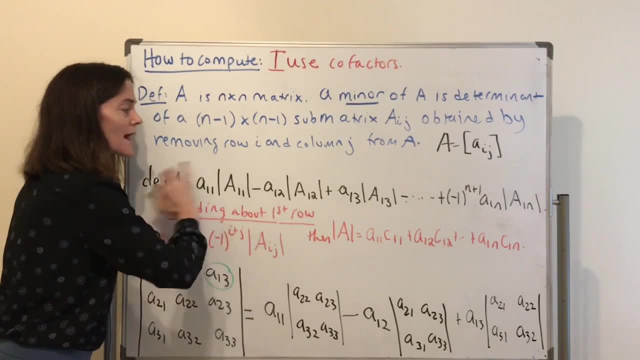 well, if I expanded about the first row, as this formula does, I would march along the row and each one I would have an A11.. This would be a 3x3 determinant. then minus A12, a 3x3 determinant. 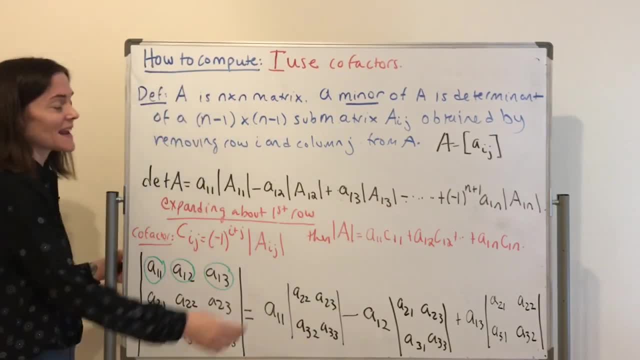 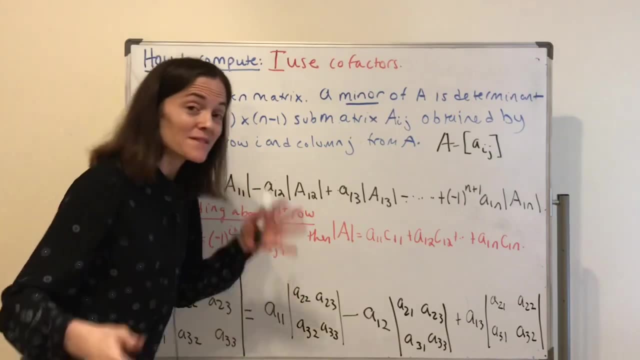 plus A13. A 3x3 determinant. and then I'd have a minus A14, a 3x3 determinant, But then to compute each one of those it would be a whole thing like this: a 3x3 determinant. 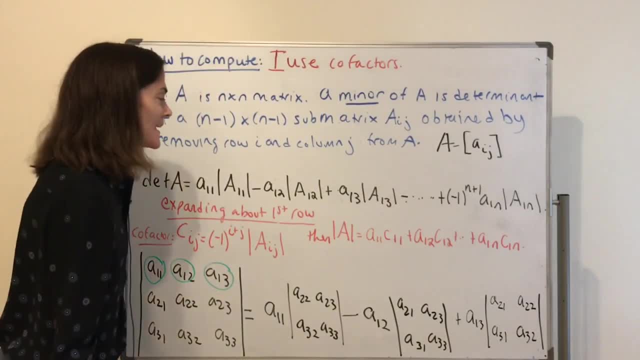 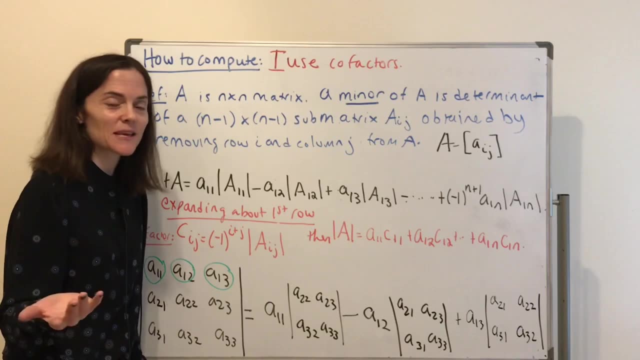 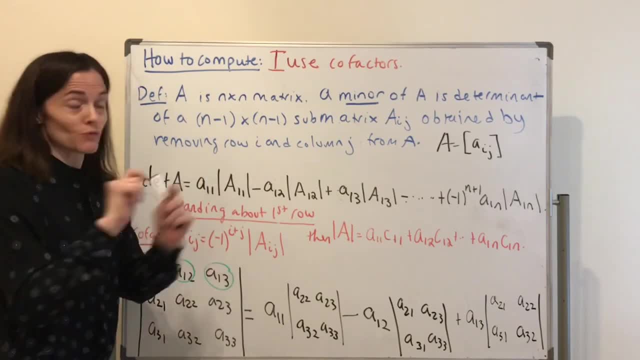 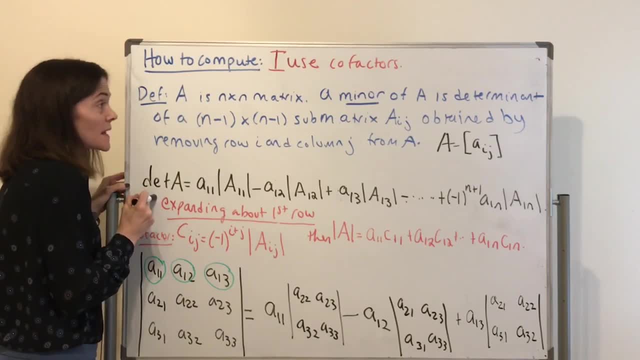 now you're gonna make. if you move it cooked at the end, you gotta double step on your instrument on this row and then startências like this in place of them. You can also do what I did in red. is you want to do the azimuth? Fif也可以 de l abuse. 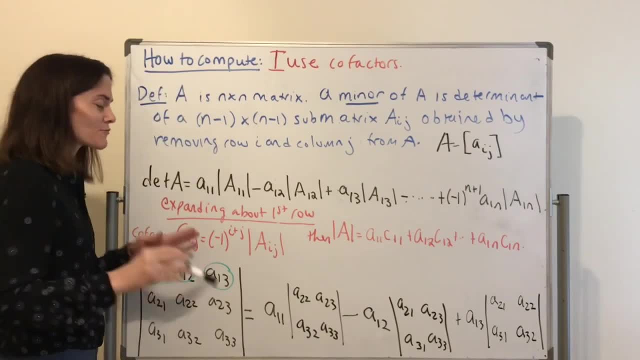 or the etherileen you wanna do with. that would work either way, but you can let that, or either one. you know the general curve or whatever can be done. So you wanna go around the mother. I will tell you where the mother can be. 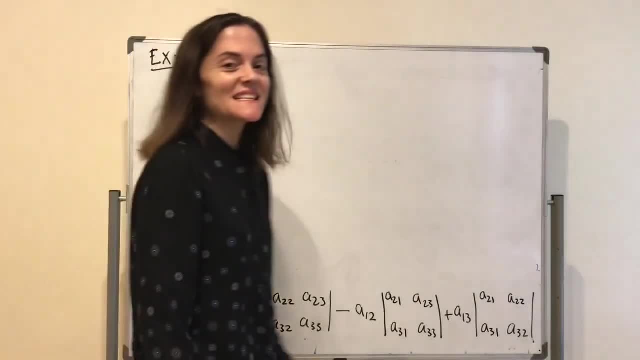 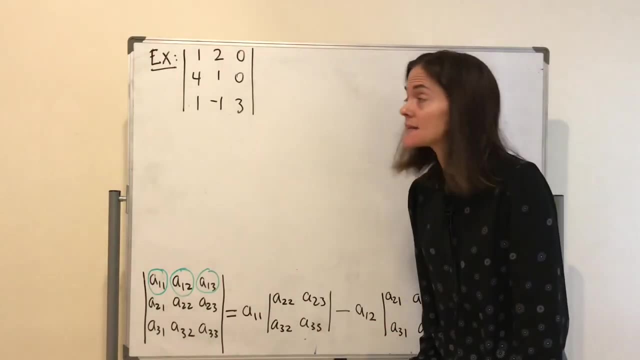 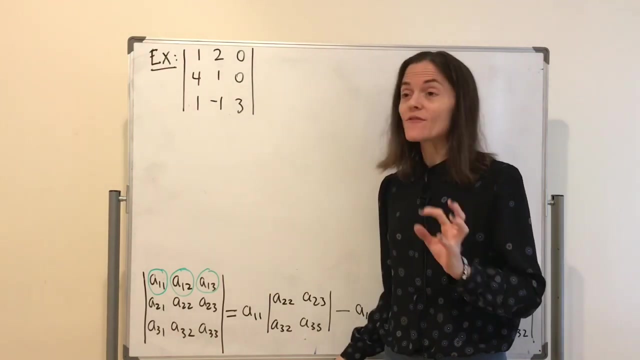 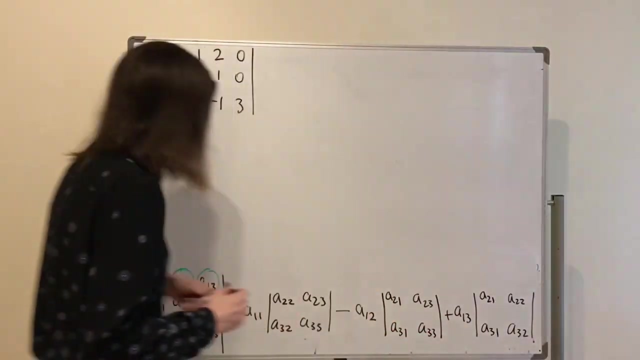 or the central curve start. even in this example, I will mention how we can approach it a little bit differently and we can be strategic as to what we expand about. so, expanding out the first row: okay, very nice. maybe I'll circle the entries of the row. 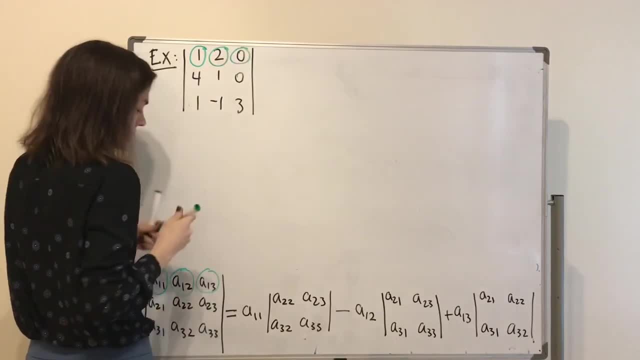 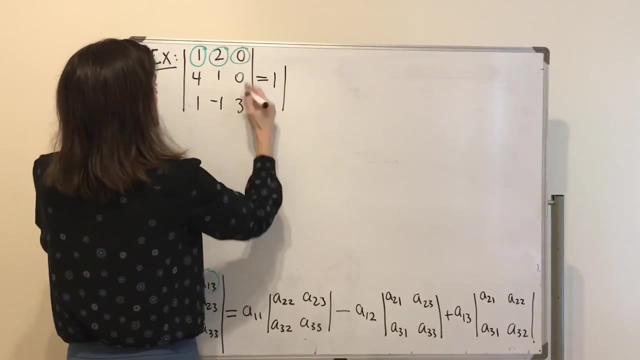 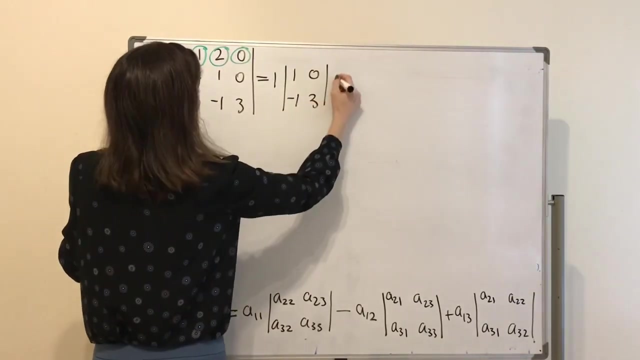 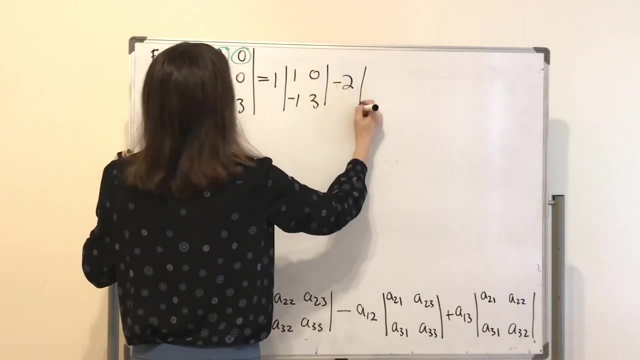 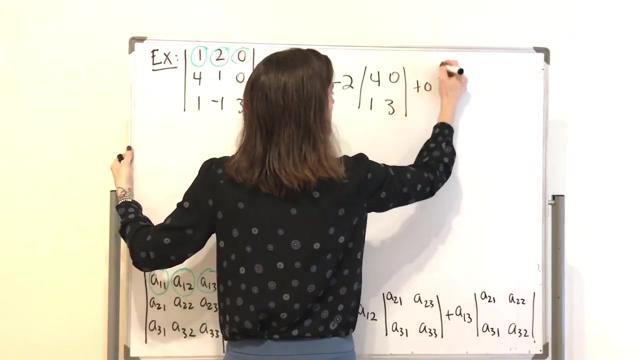 again. it's here, here and here. this would be one times. while you cross off the column in the row, we get one zero minus one, three minus two times you cross off the column, cross off the row. is this determinant? four zero one, three, and then here plus zero times. well, I don't even really need to fill it in zero times. 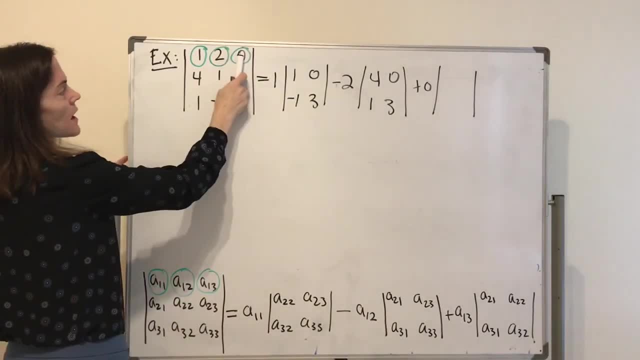 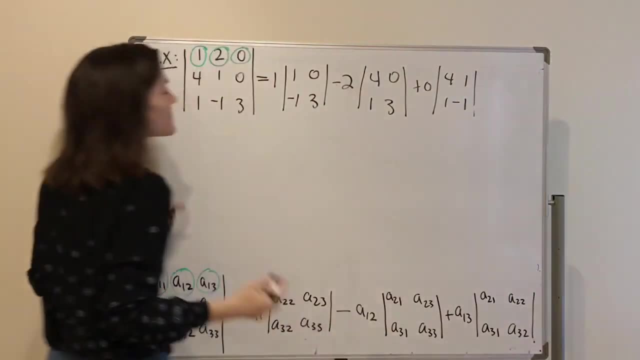 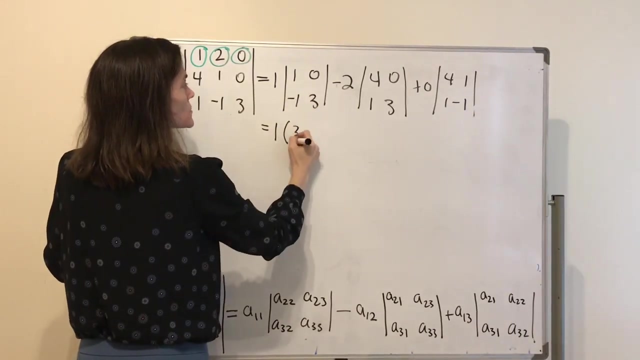 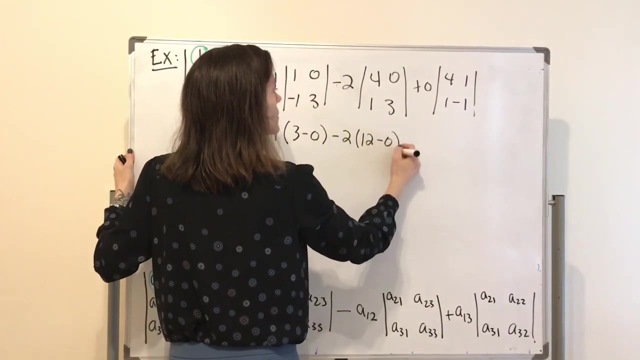 anything is zero, but I will, out of completeness. you cross off the column, cross off the row. we get four, one, one minus one. okay, and now we finish by calculating these determinants. so this is one, this is three minus zero, this is minus 2, 12 minus zero. and then I won't even worry. 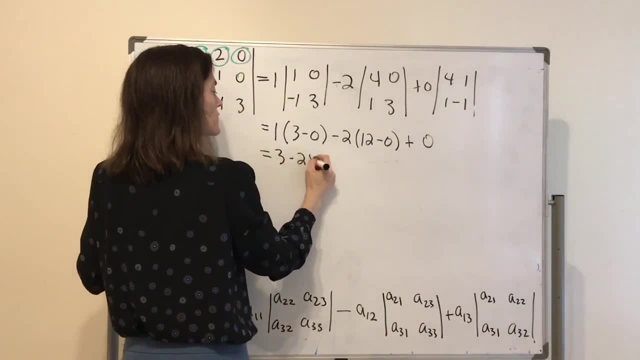 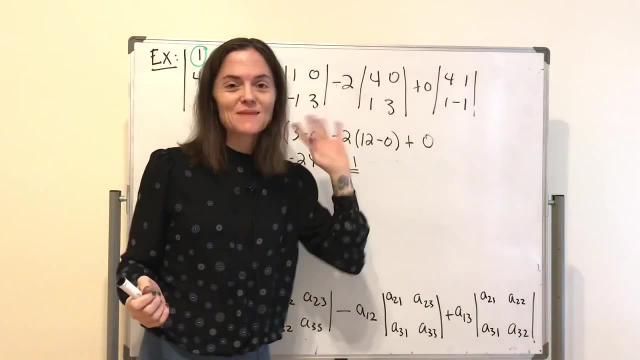 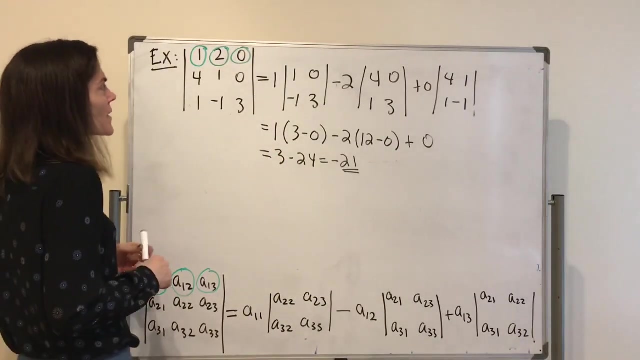 further and we get three minus 24 negative 21. okay, this determinant is negative 21. it means, in fact. it means, in fact, this matrix here is invertible because we got something other than zero, just as a side comment. okay, but what else could we have done here? this wasn't too bad. 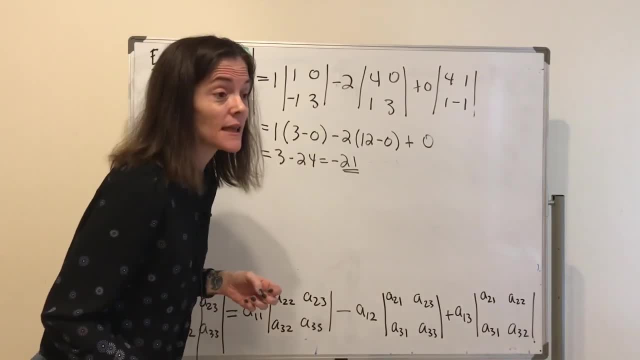 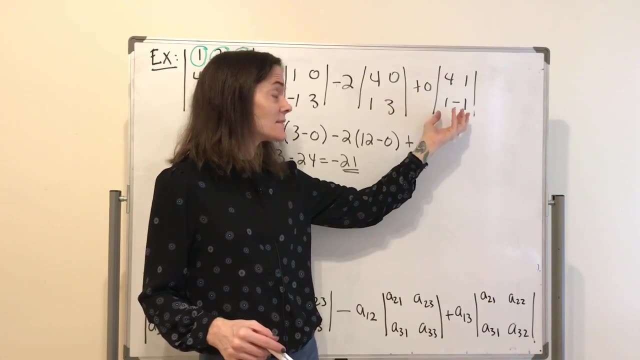 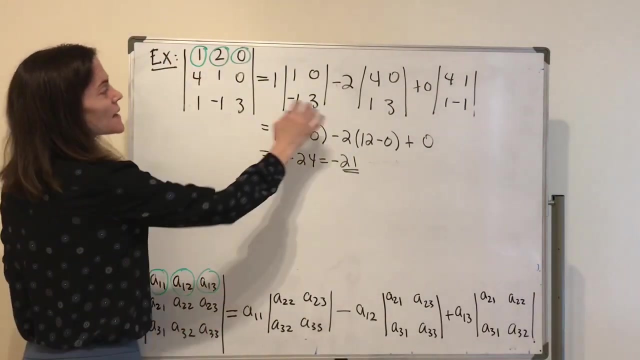 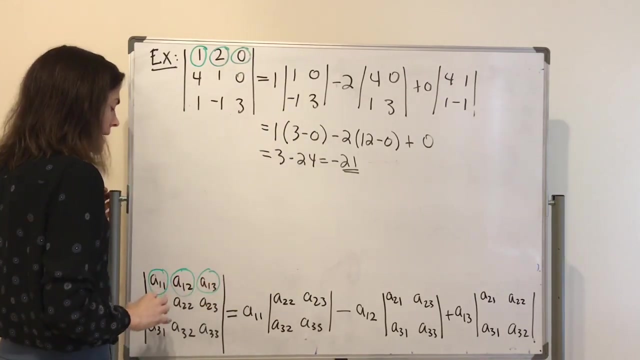 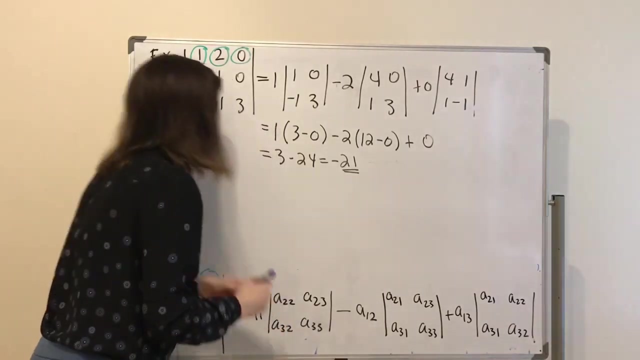 and you noticed that my life was easier because I had a zero times one of the cofactors, right, okay, so if I had had more zeros here, it would have been even simpler. and you notice i have two zeros and this column. now there's nothing special about the first row and this expansion. you canv, you can expand a. 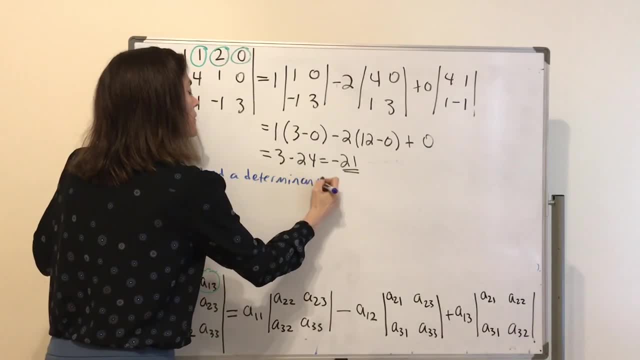 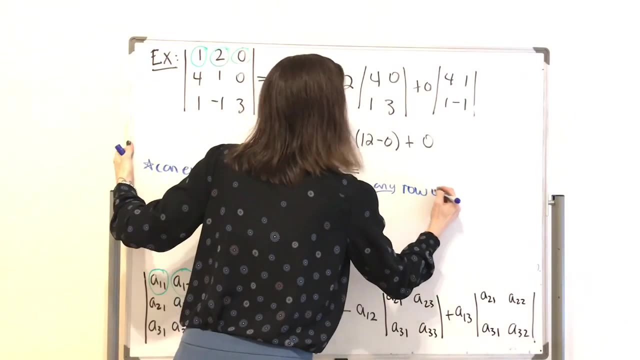 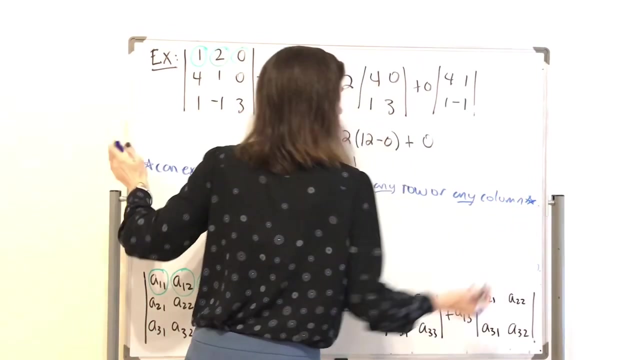 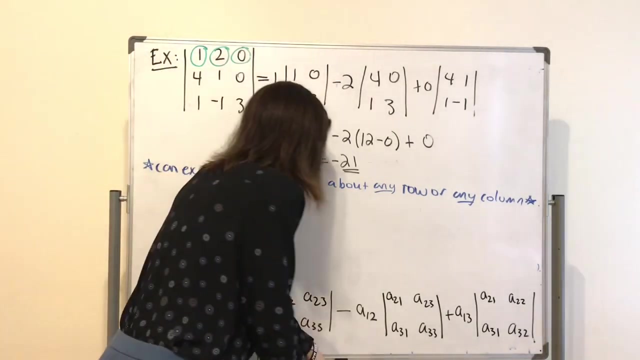 determinant about inieman, or you can expand the determinant婠 extent or any row would do good column okay, so let's just I will expand this one about column 3 because of all the zeros, but before I do, let me just show you what would this look like, maybe? 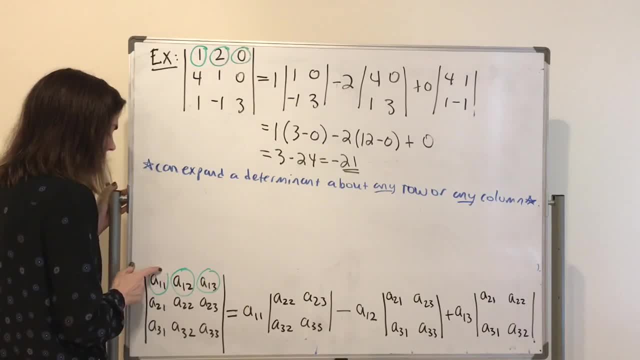 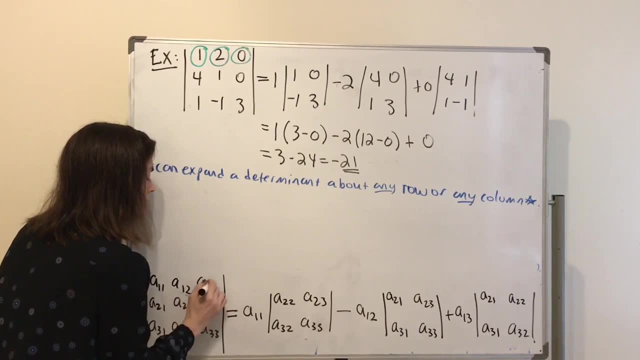 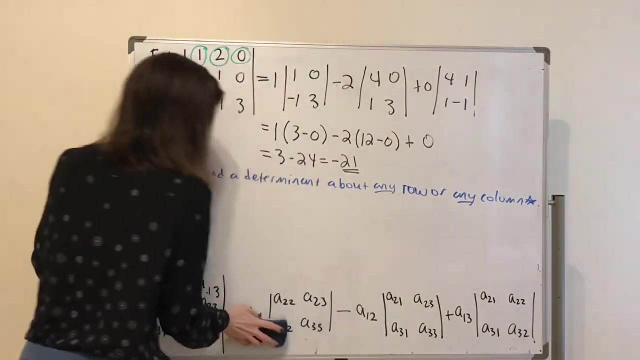 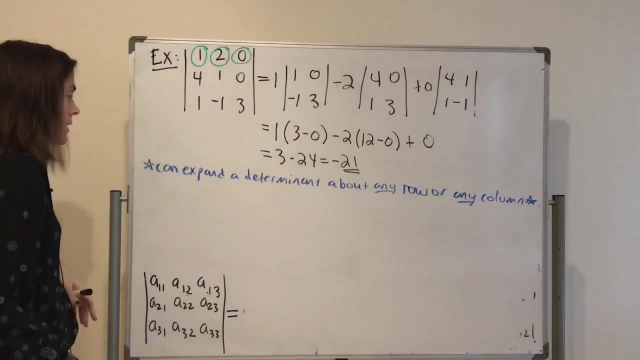 I won't put the general formula, but let's just do this exact same one here about a different row. it's a lot easier to just understand what you're doing than it is sometimes to wrap your brain around a general formula because of all the indices. so what do we do? if I wanted to expand about something else? well, if 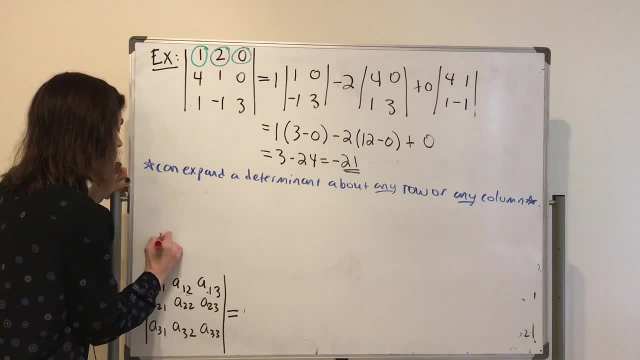 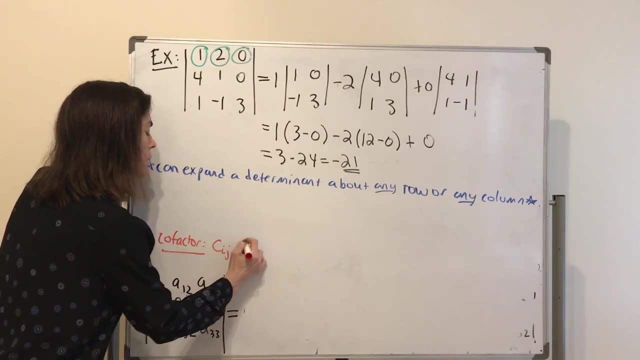 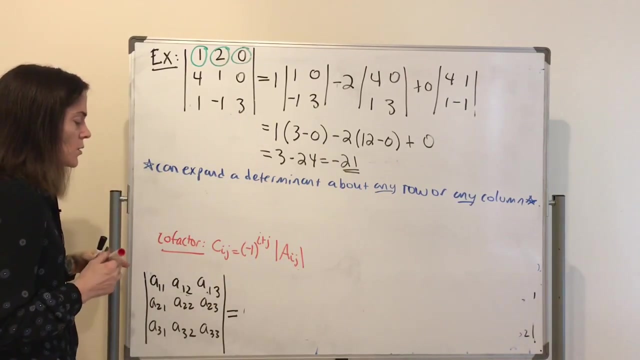 you remember, and maybe I should have left it on the board- this cofactor that comes up and the determinant is CI J, which is minus 1 to the I plus J times this minor. okay, so you can choose your favorite row or your favorite column for this matrix. 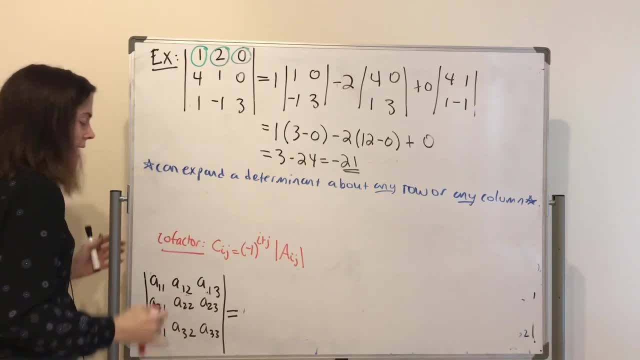 this is my favorite column and expand about that and it's going to be a sum of whatever times the corresponding cofactors, except the most important thing to keep in mind is this: minus 1 to whatever power, because that matters. so, for instance, I, here you start at the 1: 1 position is going to be minus 1 to the. 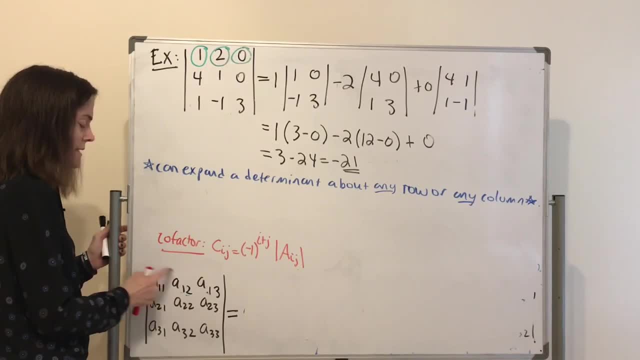 1 plus 1, that's 2, and so it goes plus minus, plus. and we see this here: plus minus, plus. okay, but if I, for instance, started in the second row, well, 2 plus 1 is 3. it's going to be negative. so this is going to be negative, positive. 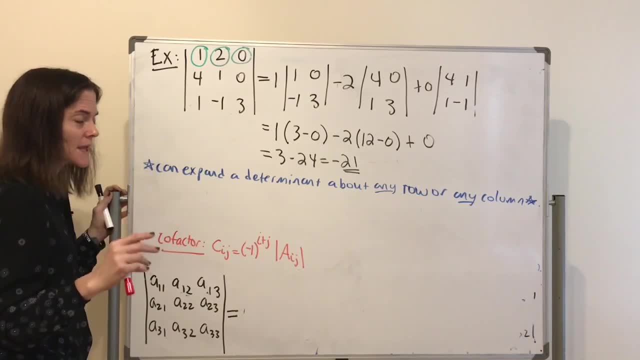 negative like this and the way that I remember it is not necessarily that it's I plus J. I just started the 1: 1 position plus and then I move, this will be minus. I move down 1, or if I went over 1, that would be minus, and then I just start. 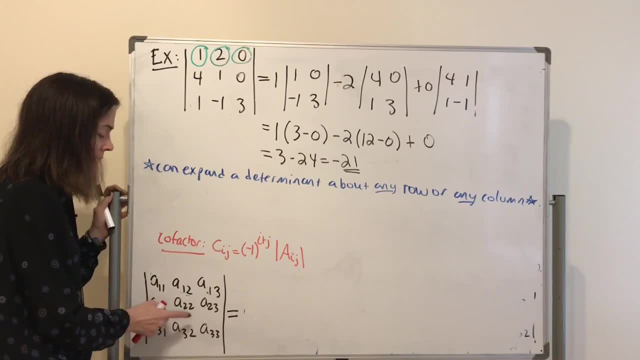 alternating. this is going to be minus plus minus, so maybe let's write that just as an exercise. what would this look like? expanding about the second row? then we'll do this example on the third column. so you see how it works with two different things. so if I wanted to expand now, I will expand on the second. 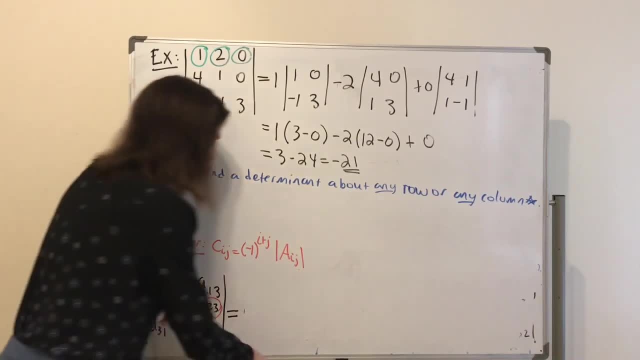 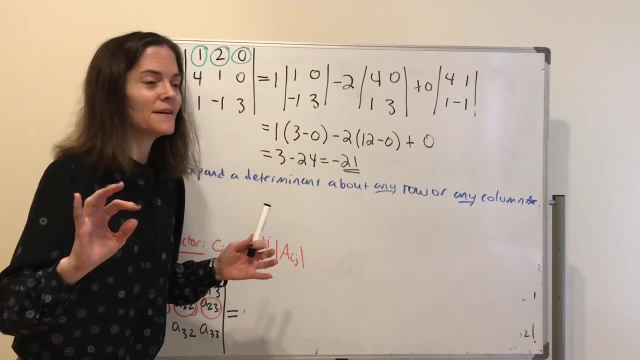 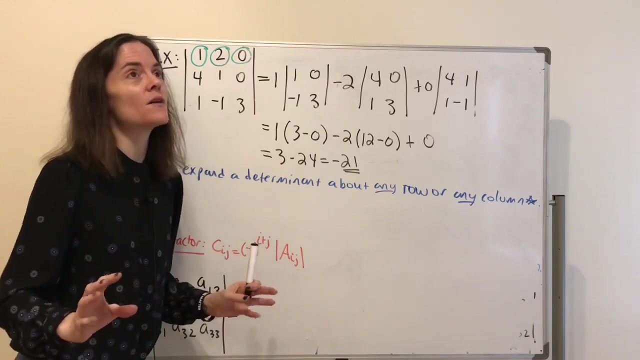 row. let's just write it out as an exercise because you can do. this is what's so nice, especially when you have a big matrix, because I could give you 100 by 100 and I won't, but I could. I just take a lot of paper to even print 100 by 100, but I could, with tons of zeros and you. 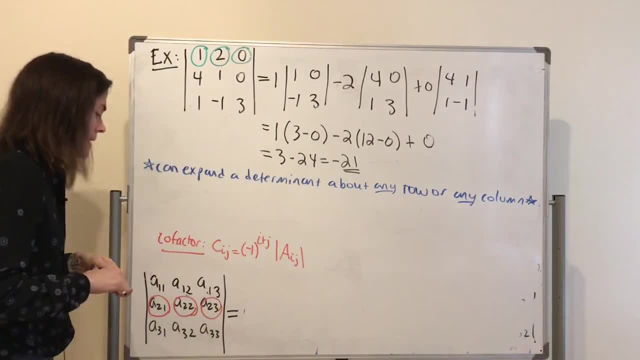 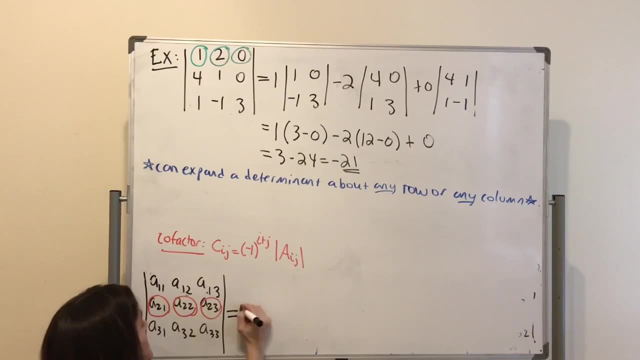 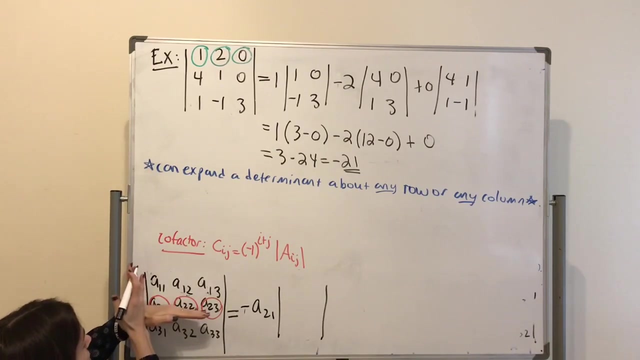 could have to determine it just like that. okay, okay. so what would this look like? well, here is: this is plus, this is minus, so this will be minus a 2- 1. and then we have this determinant where you cross off this row and this column and you see it is a 1- 2. 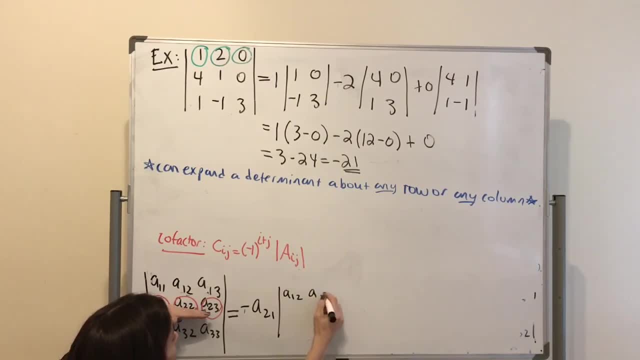 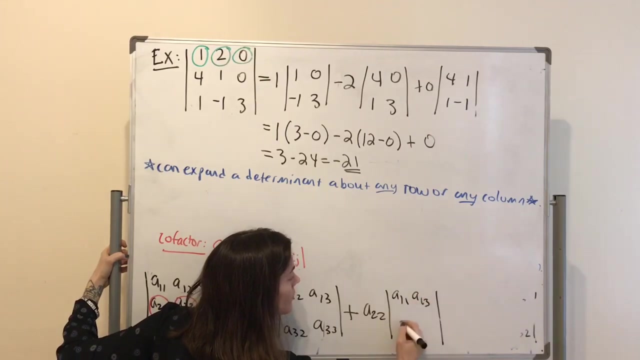 a 1, 3, and then a 3, 2, a 3, 3, and then you could write: okay, plus, because it went minus me, plus, minus, then it's gonna be plus, minus, like this: this one's plus. then here I cross off, cross off, i get a 1, 1, a 1, 3, a 3, 1, a, 3, 3, and then I have another. 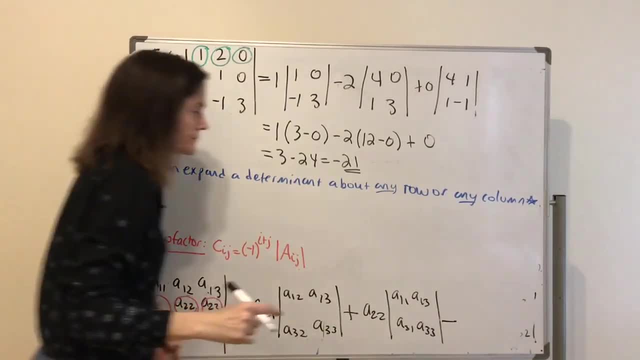 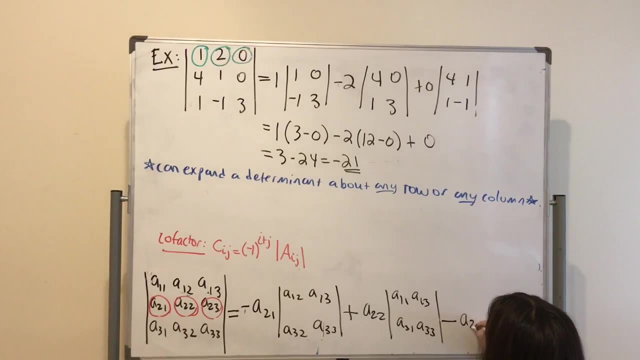 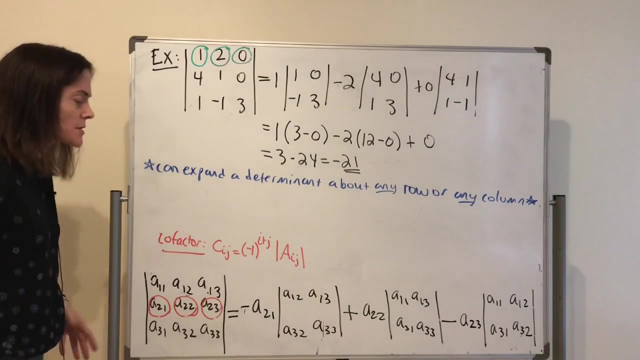 minus its 823, and you cross off the 2nd row, 3rd column�, third column. you see you get this two by two. Okay, so this would be another formula for the determinant of a three by three matrix. Now, if you multiplied it all out, you would see the exact. 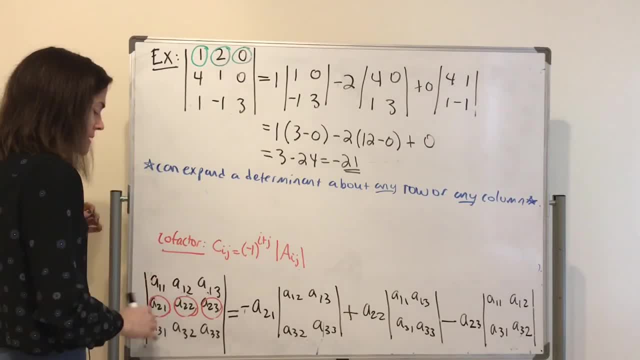 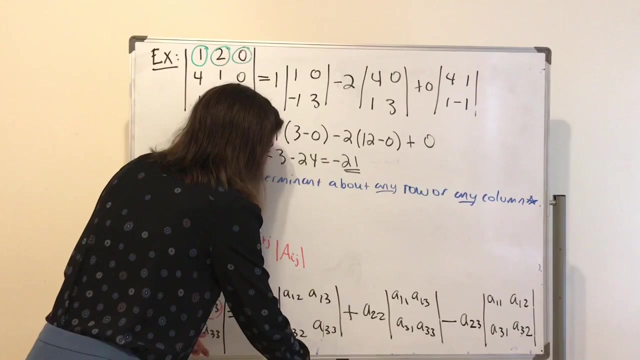 same thing as what I wrote before, But I just wanted to practice expanding by. in this case, I chose a different row because you could choose your favorite, depending on the matrix. Okay, now let's go back to this example. As I mentioned, when you see lots of zeros in a row, 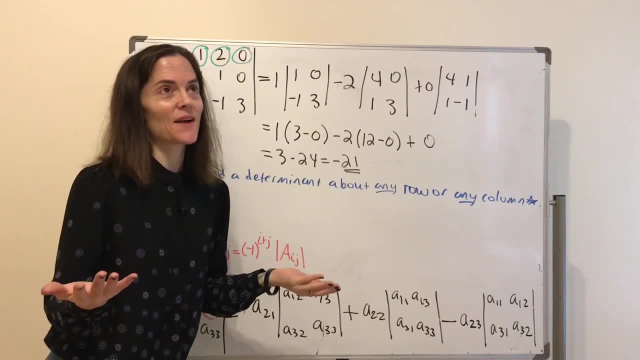 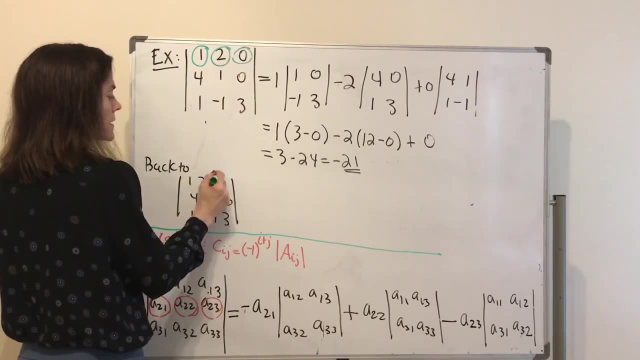 or lots of zeros in a column. this is the easiest way to calculate the determinant. Pick that one, expand about that one because you have less steps. This time I do it a little bit more strategically. And what do I get? Well, this is plus minus, plus. So I'm going to start. 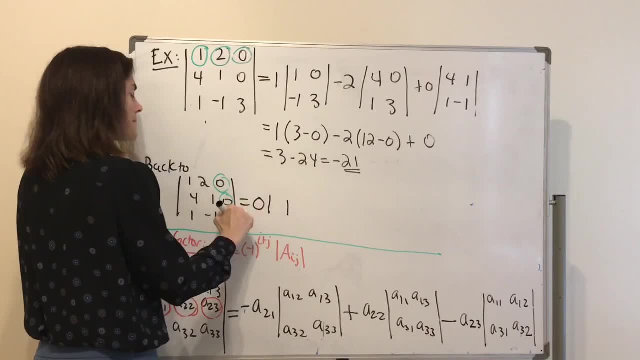 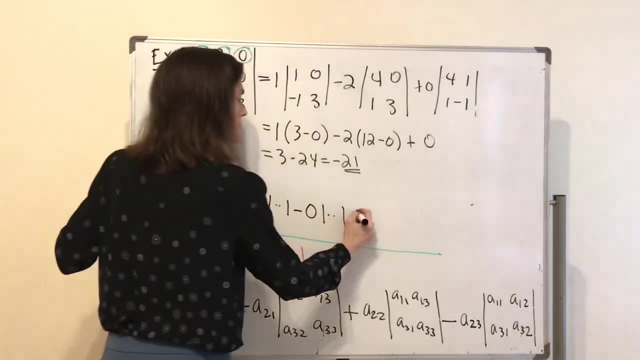 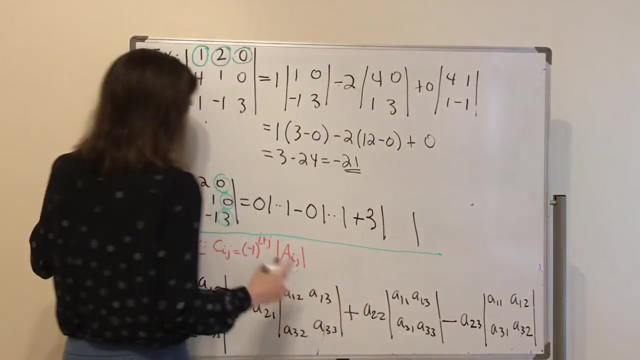 with a plus. I'm gonna have zero times something minus zero times something. I'll just put dots because it doesn't matter. And then plus, right, it alternates plus, minus, plus. then I have three. this one matters. I have the determinant of you cross off this row and this column. we see 1241.. 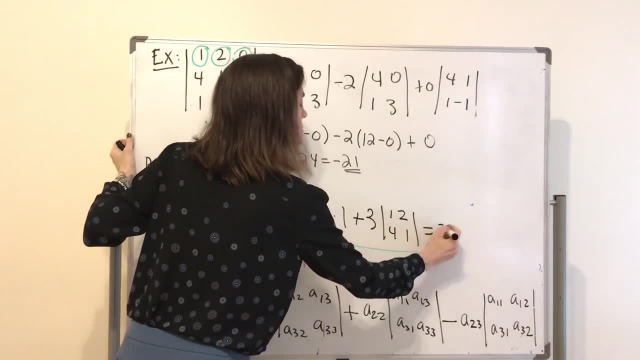 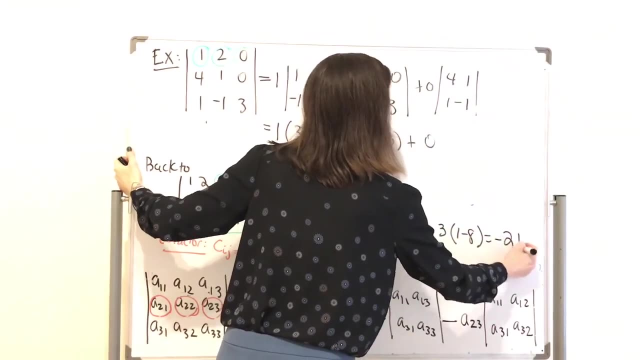 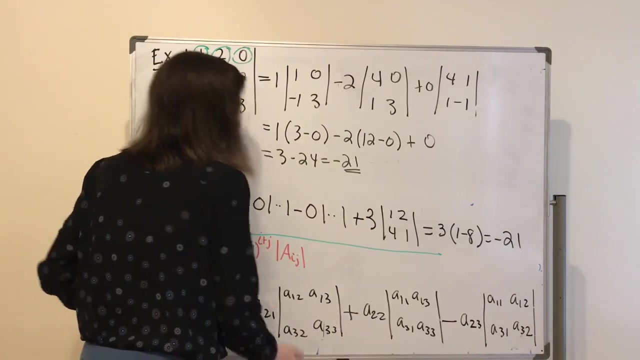 1241.. This is three times one minus zero, Minus eight, three times minus seven, in fact. Well, if I got a different answer and say I did it wrong one of the times at least, but we get the same number as we should, It was just. 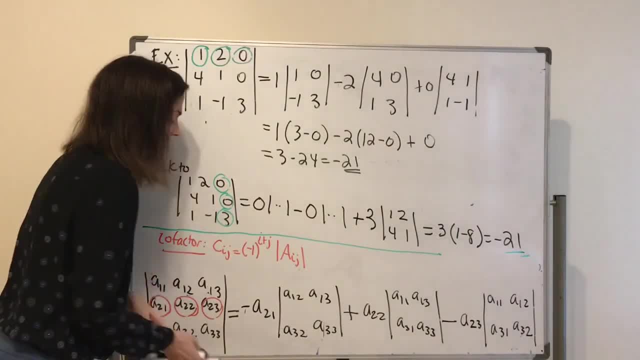 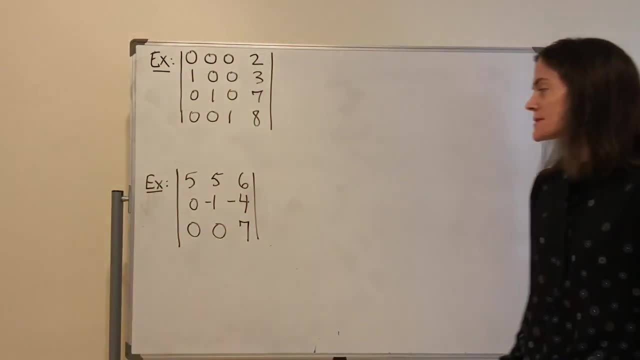 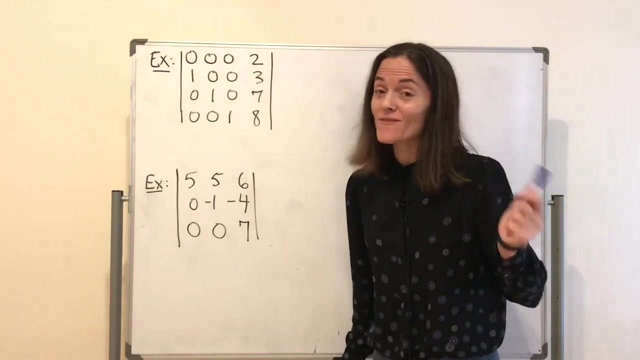 showing you a different way to expand and calculate the determinant of this matrix. Okay, let's do another one. Well, here are two more examples, And they're both fairly quick. if we're smart about how we expand- In fact this will be- even though it's four by four- this will be my fastest example of the day. 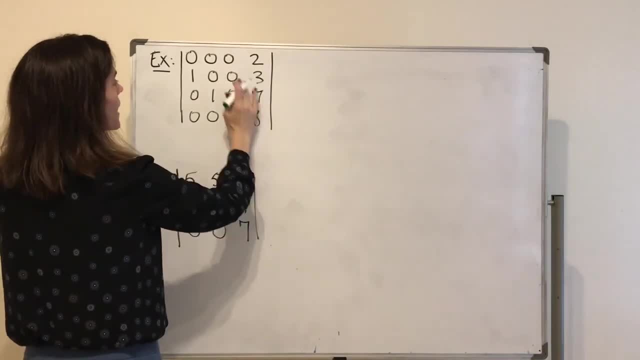 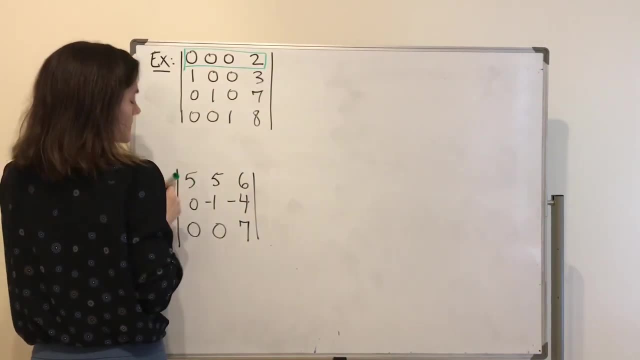 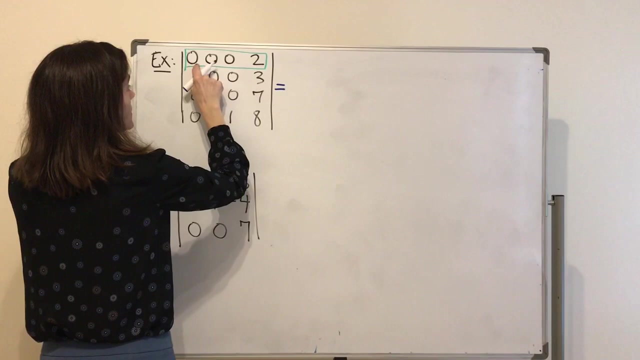 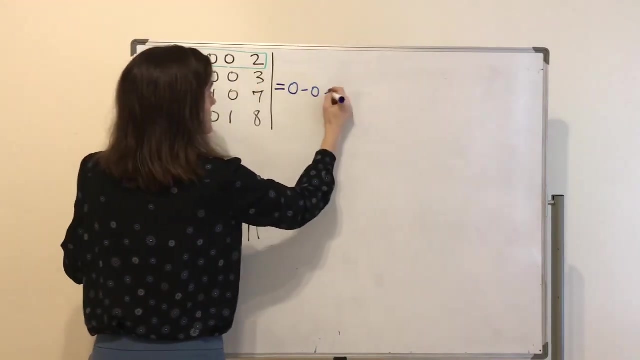 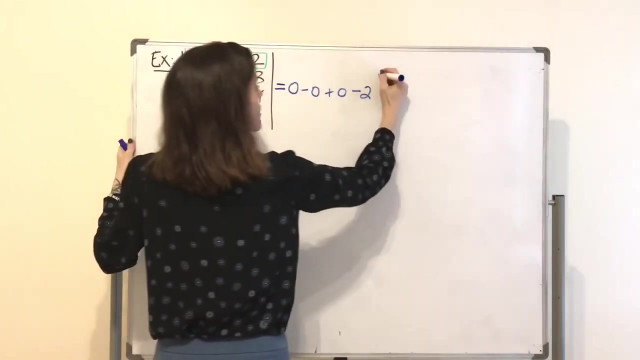 If I can cross off this column, then I see the identity here. So I'm going to expand here by the first row. And what do I get? Well, it starts off plus. So I get plus zero, minus, zero, plus, zero, minus, okay two. And then I cross off this column, cross off this row and I'm left with. 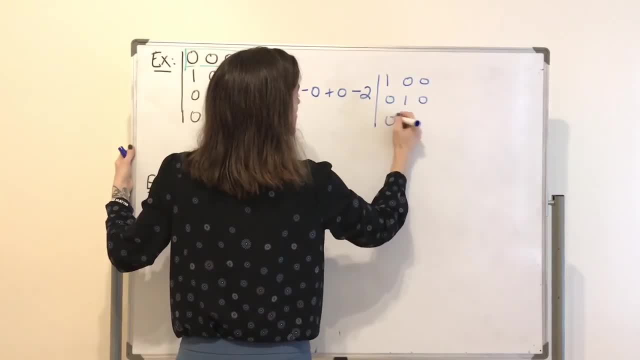 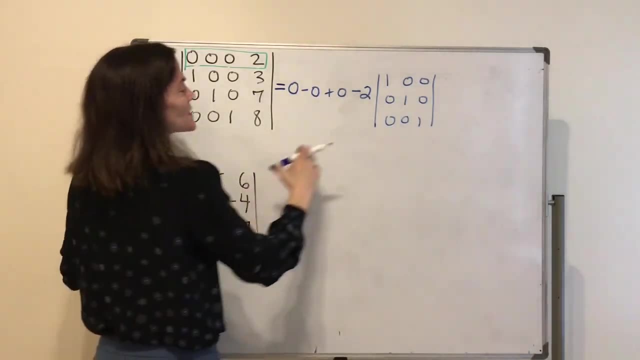 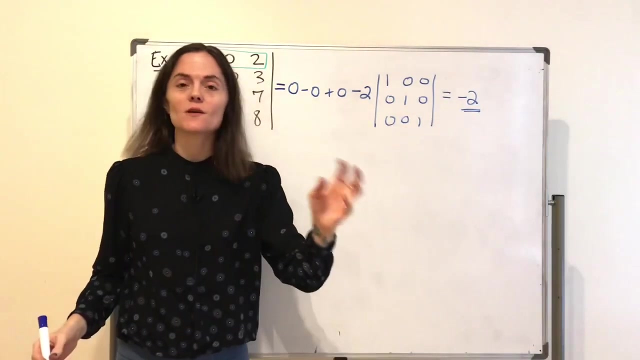 this three by three. But that is the identity And it has determinant one. So this is just minus two, Okay, but you notice, you have to pay attention. One reason I wrote these zeros was to figure out what the correct sign would be, Because you start here- it goes plus minus zero, minus two. So 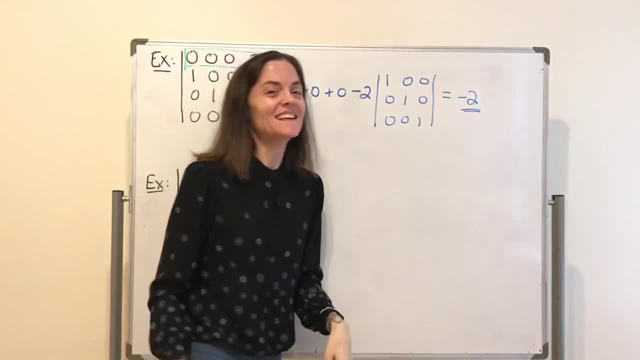 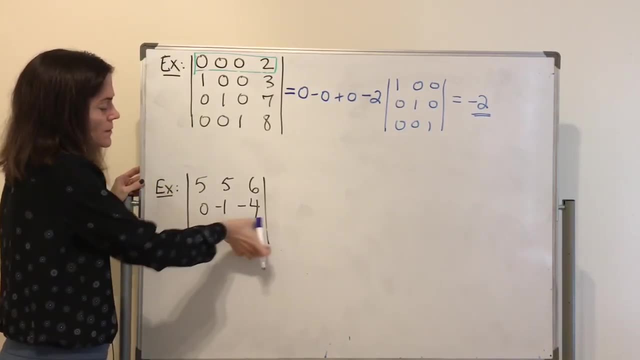 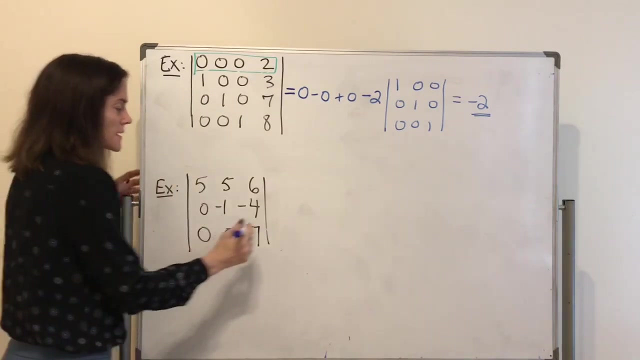 I get minus one minus four, plus minus plus minus, like this in the expansion. Now for this example: okay the old, I can either choose this column or or the bottom row, doesn't they both have two zeros and one nonzero entry? I will just pick this column, So I'm expanding on the first. 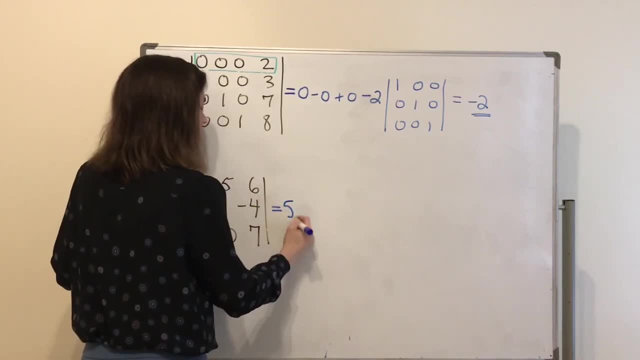 column. you see it's going to be a plus five. And then you cross off this row, cross off this column and I get minus one minus four, plus minus, plus, minus, minus, plus, minus, minus, plus, minus, minus. 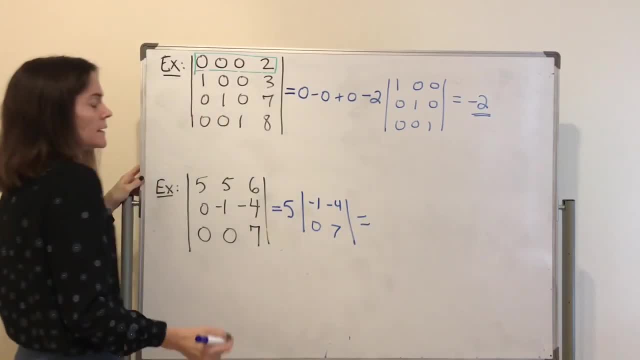 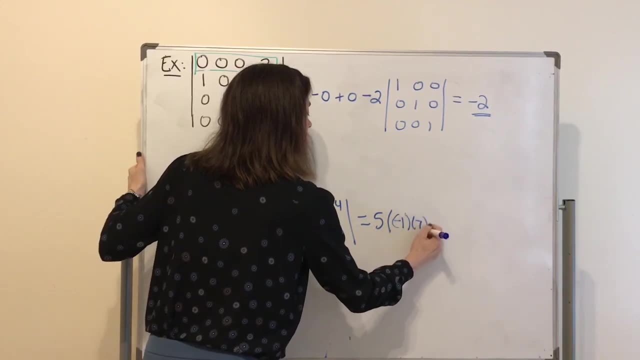 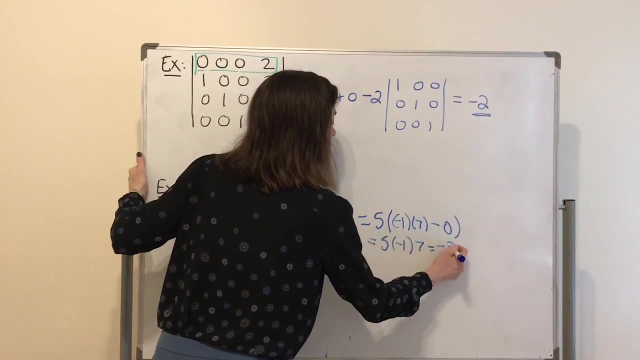 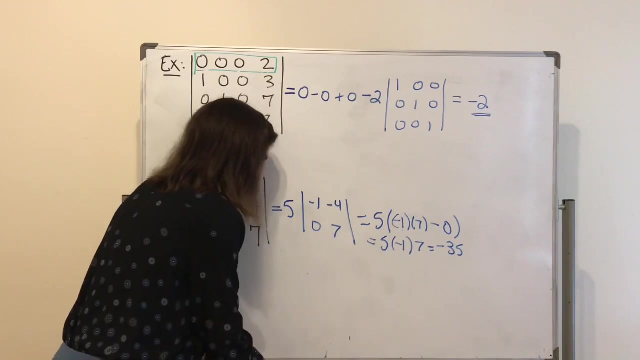 four zero seven. And now this determinant is just a two by two minus one times seven, minus zero, which in the end is just five times minus one times seven, is negative 35.. But the interesting thing here is, you notice, and this is, this is going to be the next property that I mentioned- 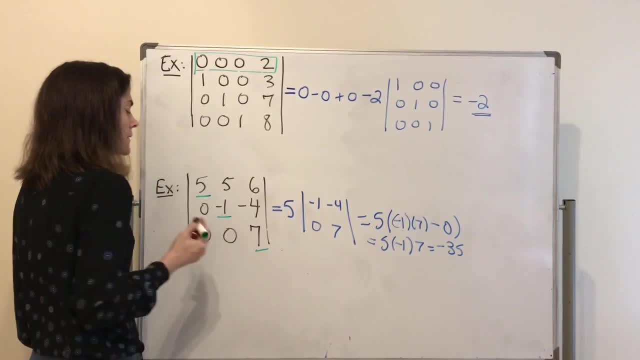 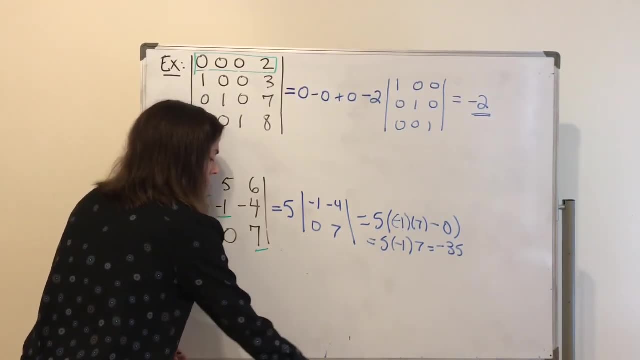 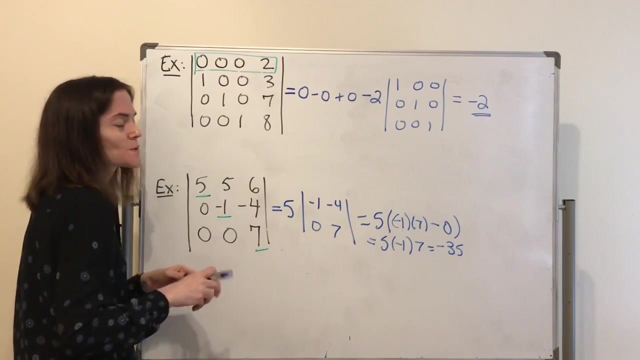 you notice? look, we got this just by multiplying what's on the diagonal. Now, just as an exercise, somebody else might want to expand upon this last row. Let's write it because we're still- well, this is not that many examples we've done, So it's still good to practice expanding about different rows. 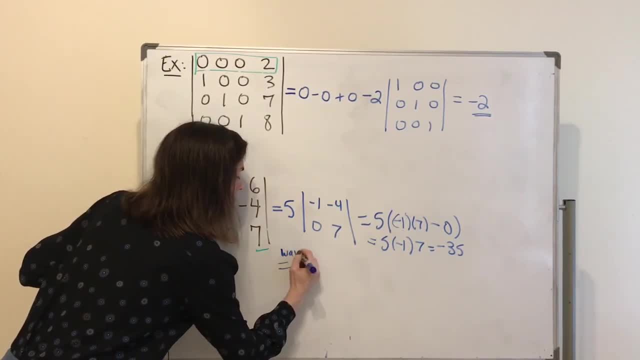 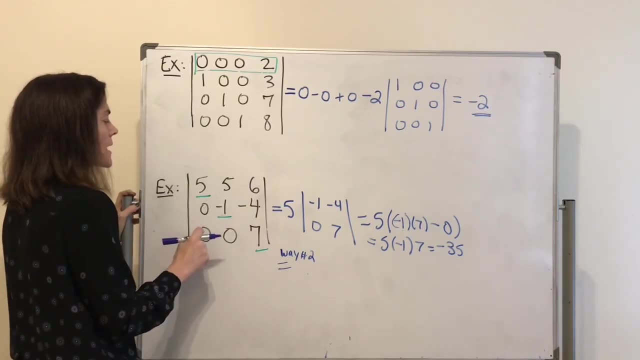 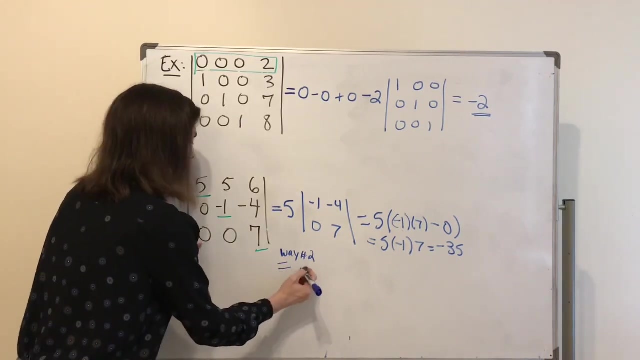 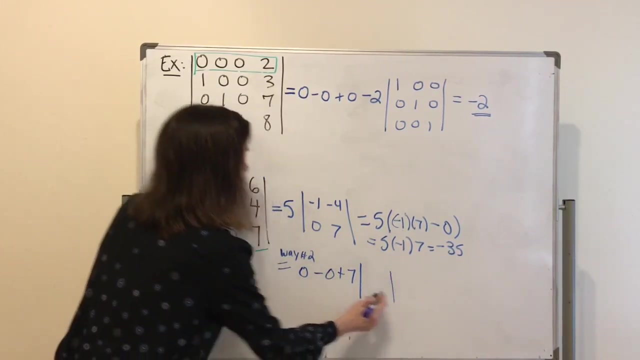 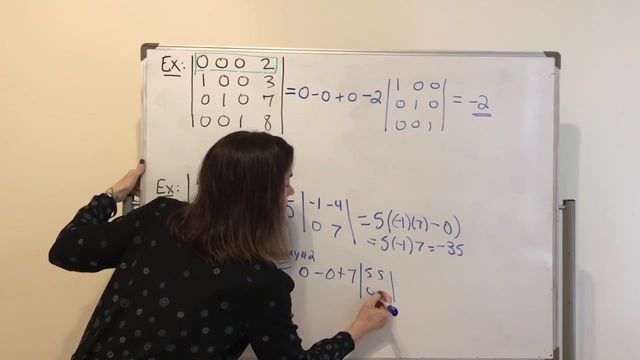 different columns, this way, number two, and then I will make my property comment that we see: Okay, so this is plus minus plus. okay, so this is going to be plus zero, minus zero, and then plus seven, And then we cross off this row, this column. we get five five zero minus one, five five zero. 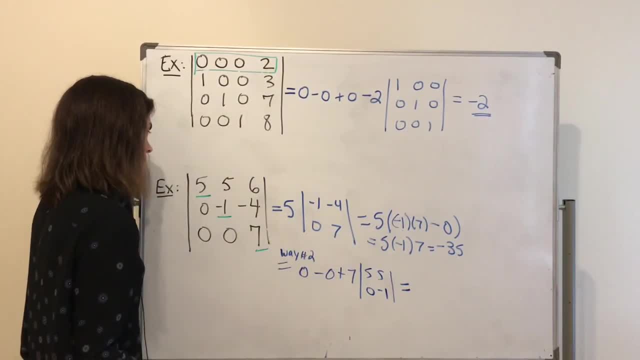 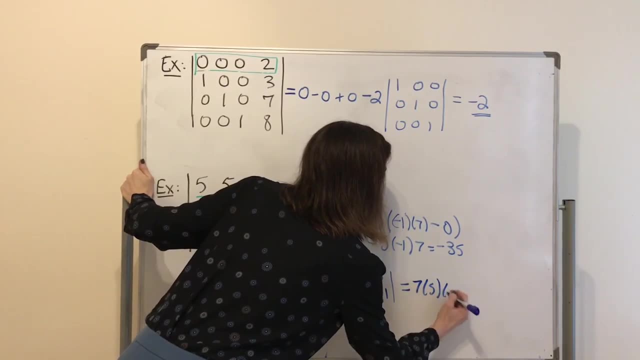 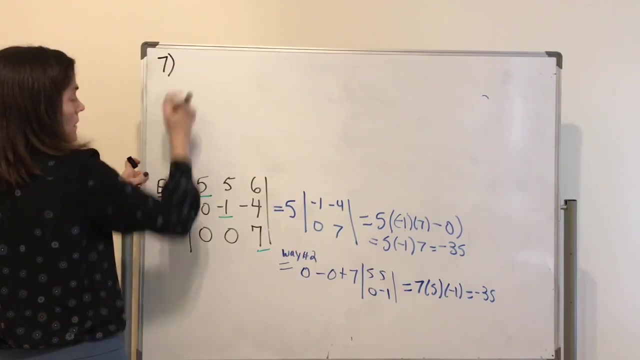 minus one. Okay, We get the same thing right. We get 7 times 5 minus 1, negative 35. But it's a different way of expanding. What we see from this example is property 7 about determinants. 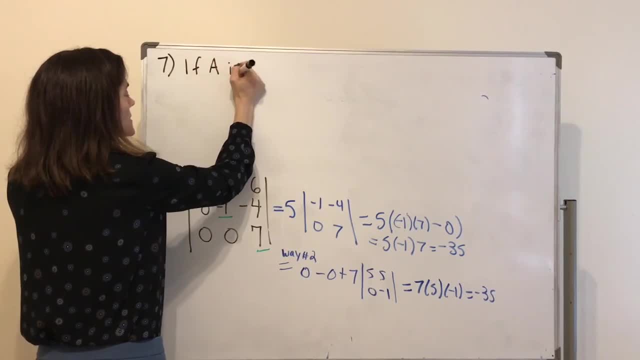 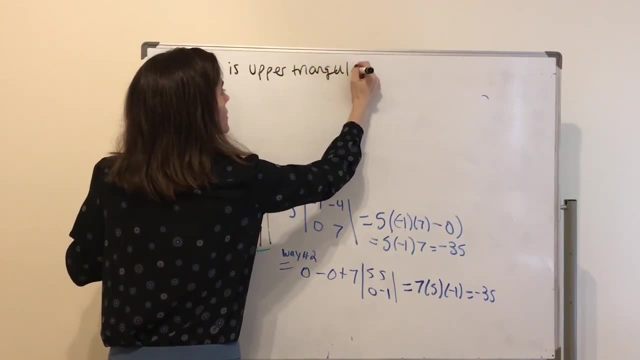 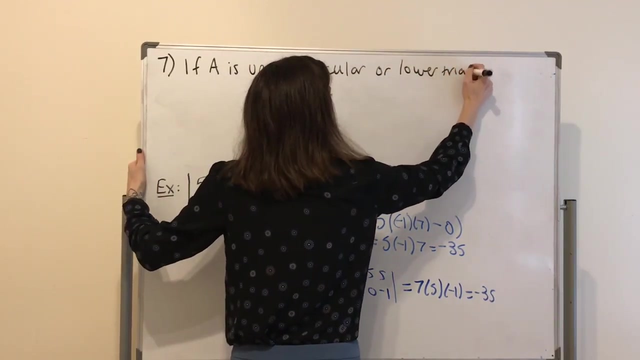 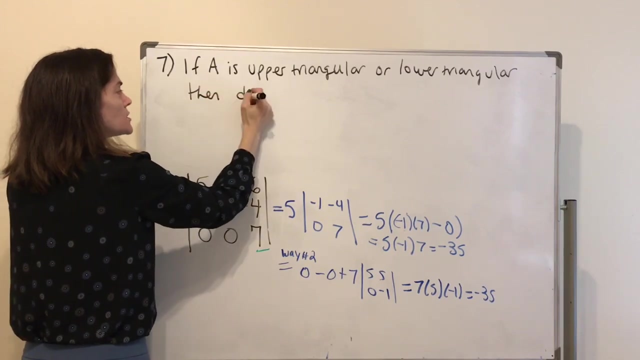 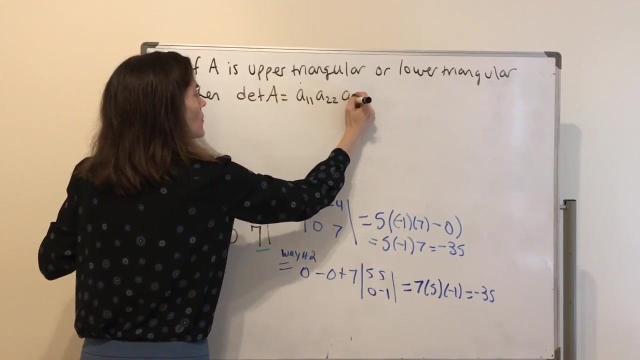 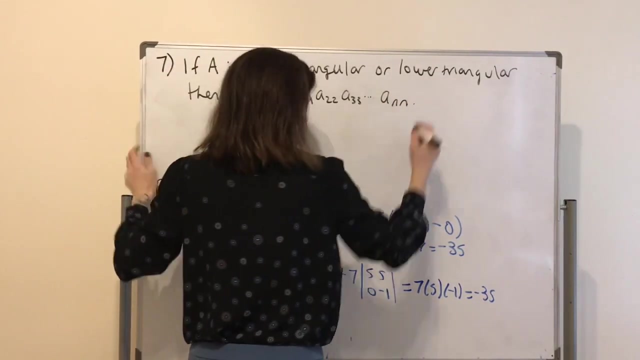 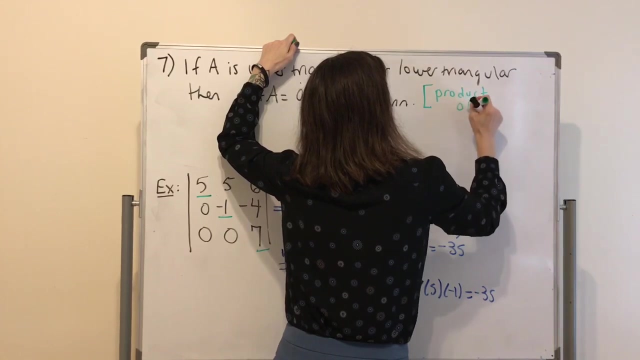 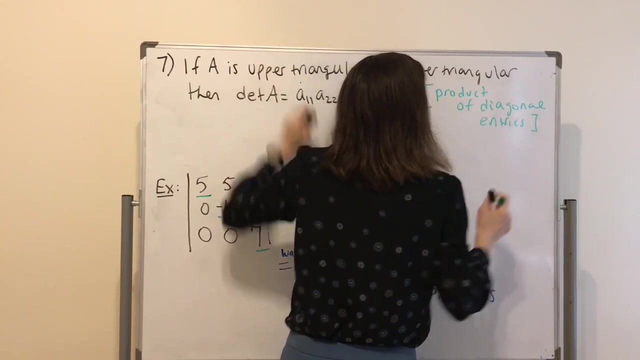 It says: if A is upper triangular, triangular, or also if it's lower triangular, then the determinant of A is this product, And maybe I'll write that in parentheses. It's a product of the diagonal entries And the nice thing about this is immediately we can make the observation. 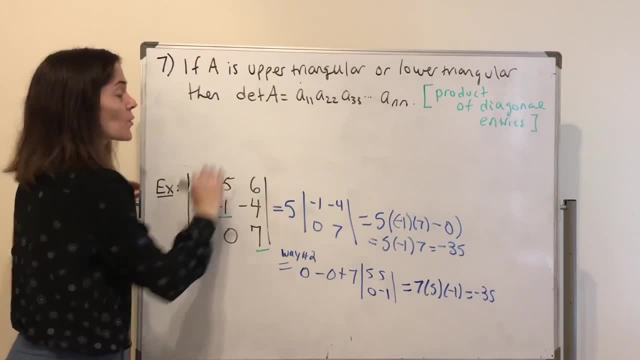 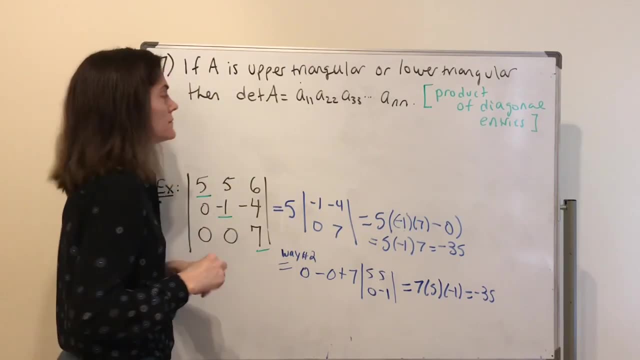 that if you have an upper triangular or a lower triangular matrix, you know right away when it's, for instance, invertible. Well, as long as the product of the diagonals, or equivalently, as long as every single diagonal entry is non-zero. 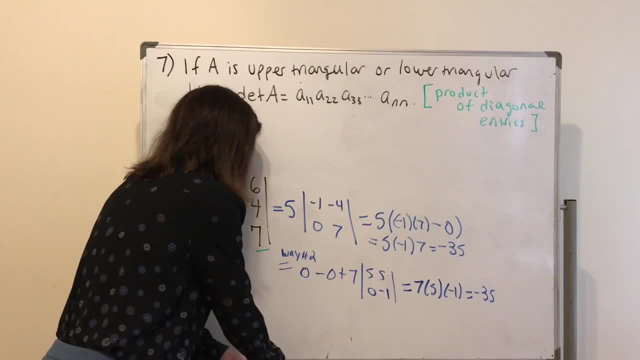 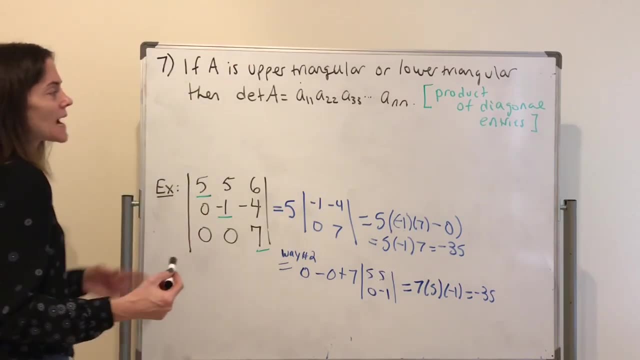 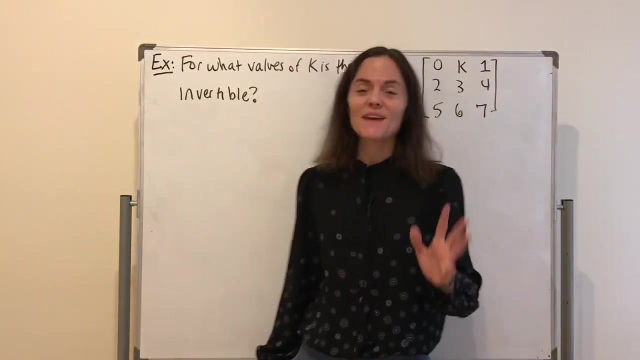 then the matrix will be invertible. You might have thought about this observation already in some of the previous work of this semester, but I wanted to make it now in light of our determinant calculations and comments, Continuing with our thoughts about a matrix is invertible. 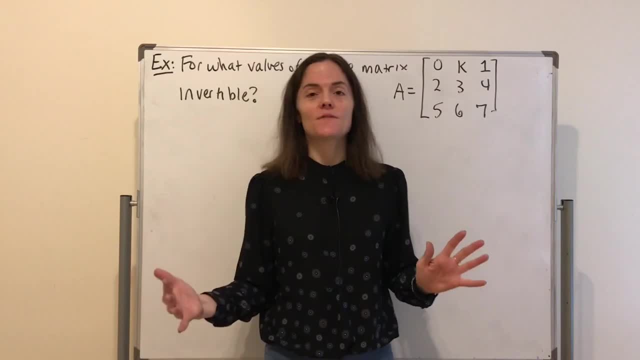 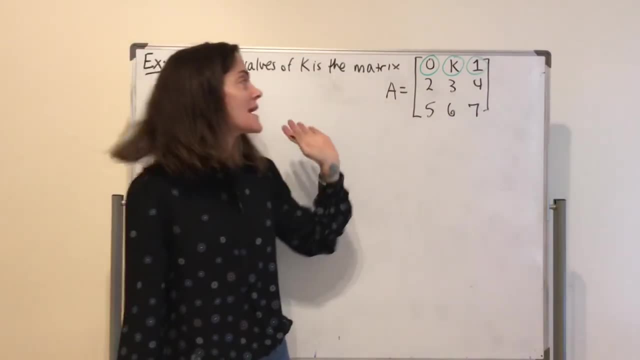 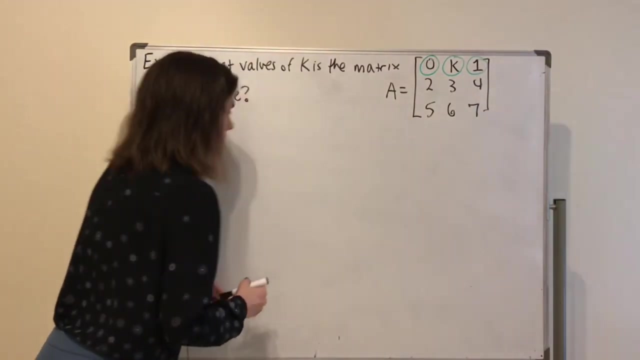 if, and only if, the determinant is non-zero. let's do a few in in that spirit. And here is one. This matrix has only one zero. I might as well expand about the first row. Here we go. So this determinant is zero times something minus k times. 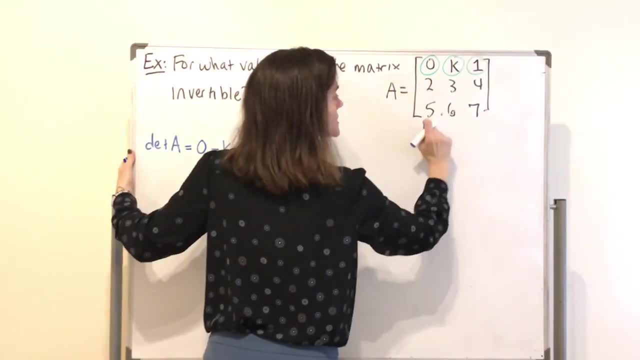 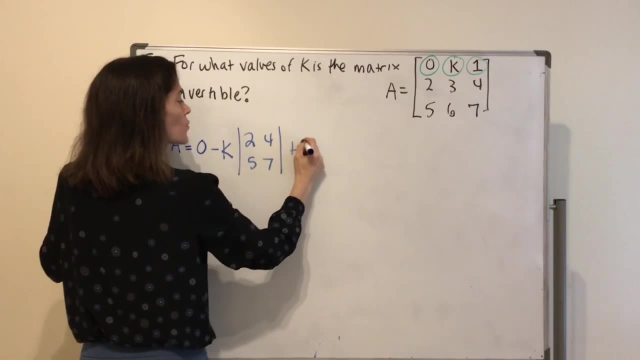 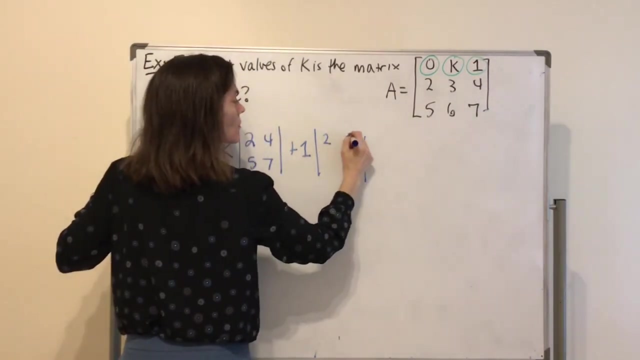 times while you cross off this row, cross off this column, we get 2,, 4,, 5,, 7.. And then, plus 1 times, I cross off the first row and the third column: 2,, 3,, 5,, 6.. Okay, This is. 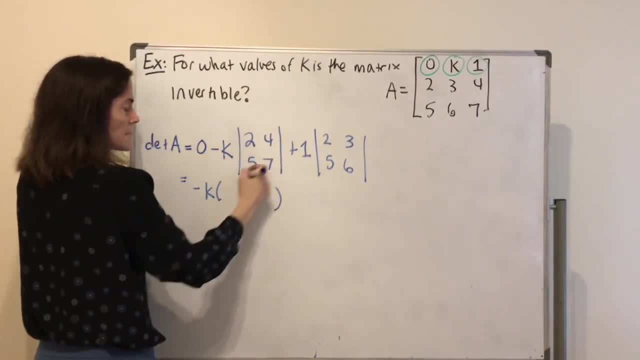 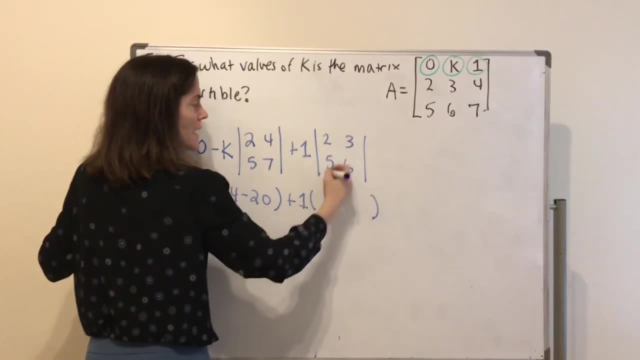 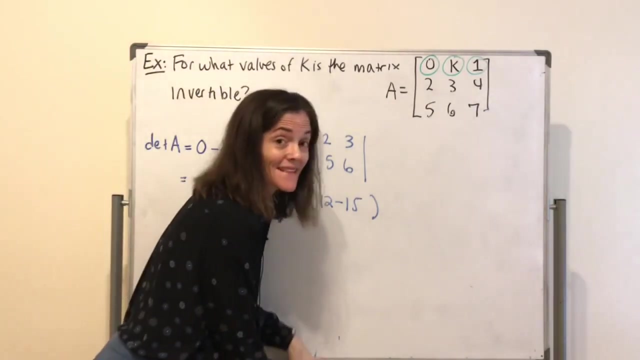 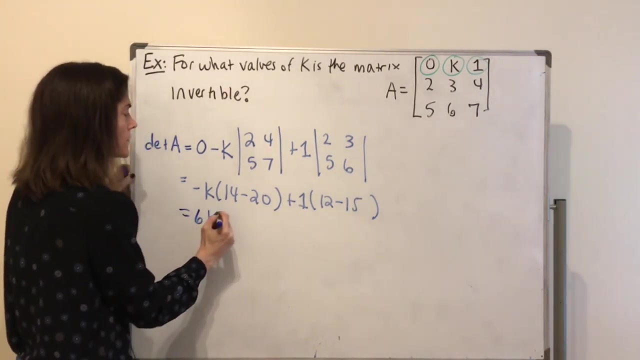 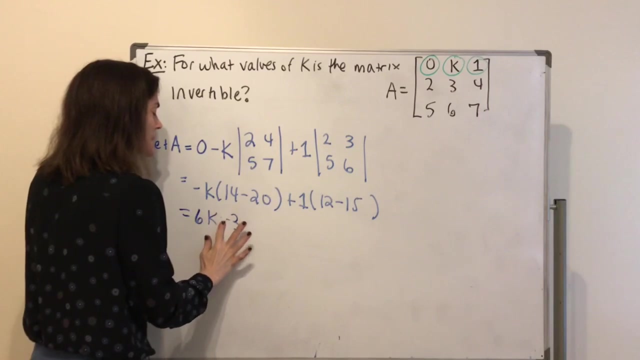 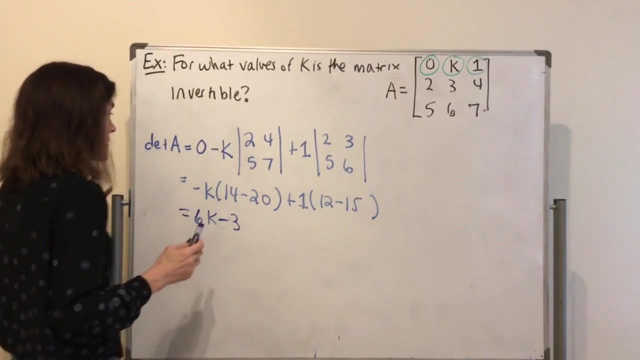 negative: k, 14 minus 20.. And then plus 1,, 12 minus 15.. Okay, The determinant of this matrix, we see, is 6k plus 3.. Okay, Minus 3.. Excuse me, 6k minus 3.. Very nice, And then, well, we know, the matrix is. 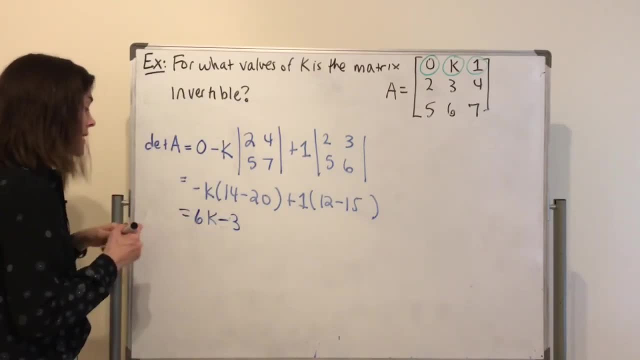 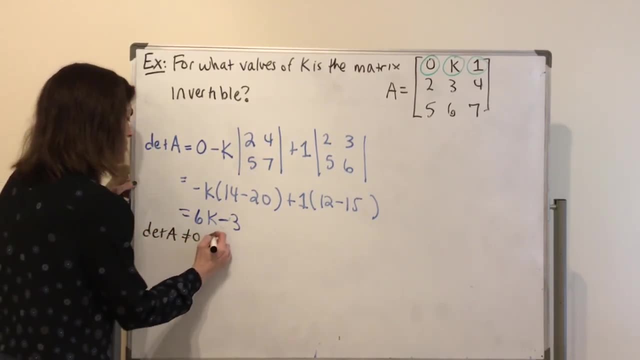 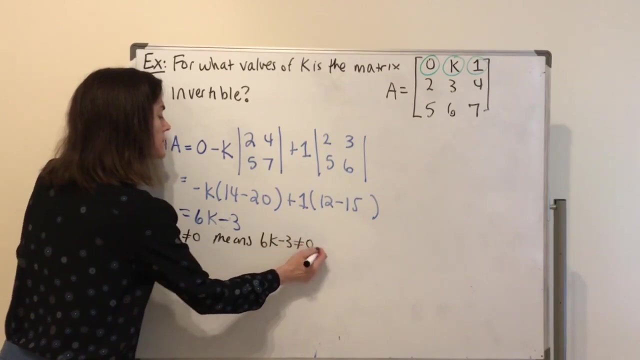 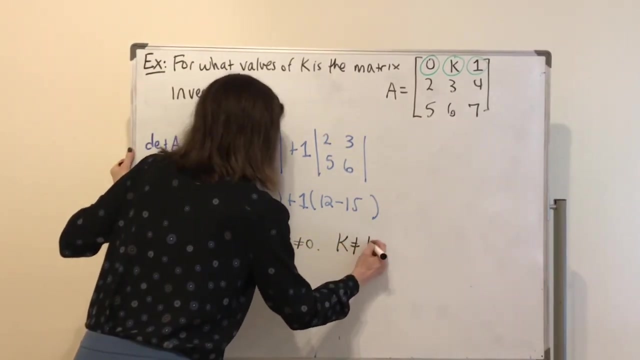 invertible, provided the determinant is not equal to 0. So the answer we need the determinant of A not equal to 0,. well, means 6k minus 3 not equal to 0. And so now we have our answer. so this will be invertible for all k, provided k is not equal to one half. 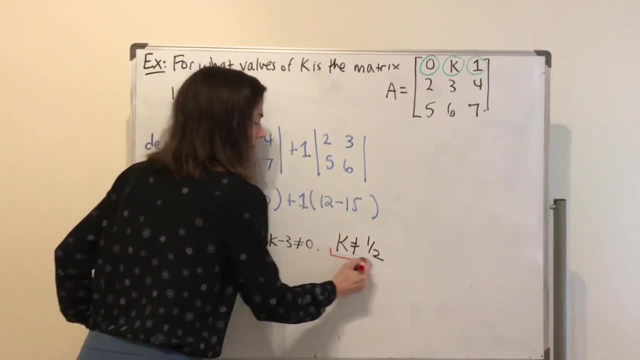 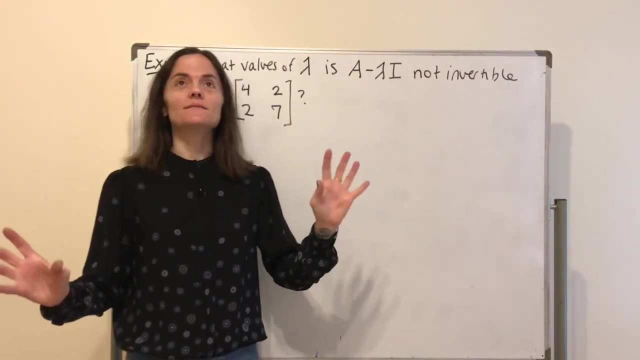 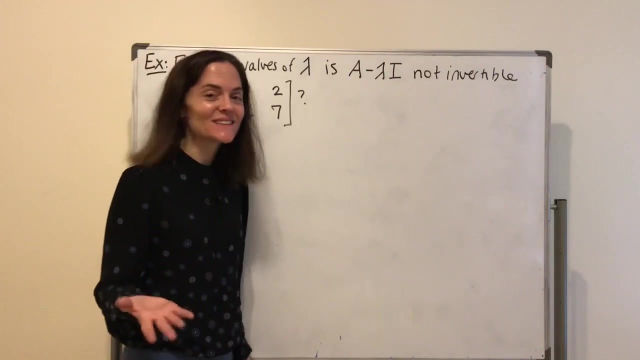 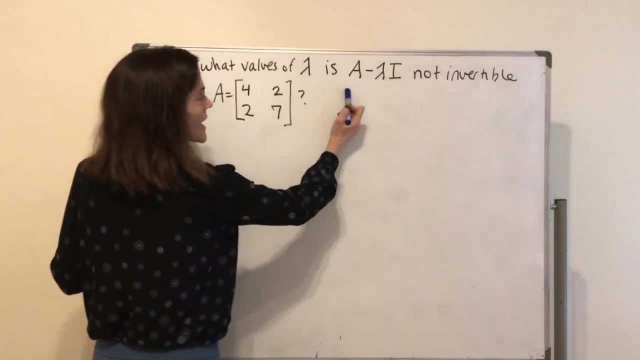 and this is our answer here. there's another question. well, and this one, i will say uh, as foreshadowing things to come, because we're going to be doing a lot of things like this very soon. okay, but this is what we will do today. what values of lambda is this matrix? a minus lambda times the identity, and this is a. 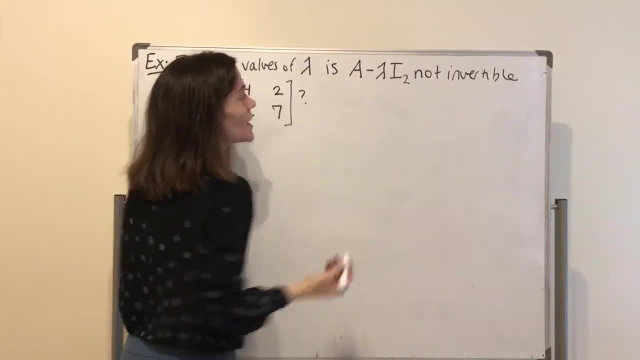 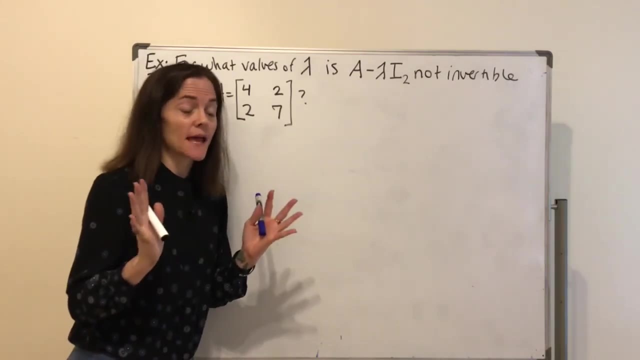 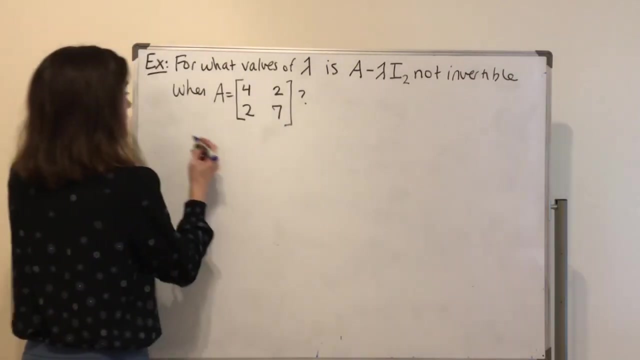 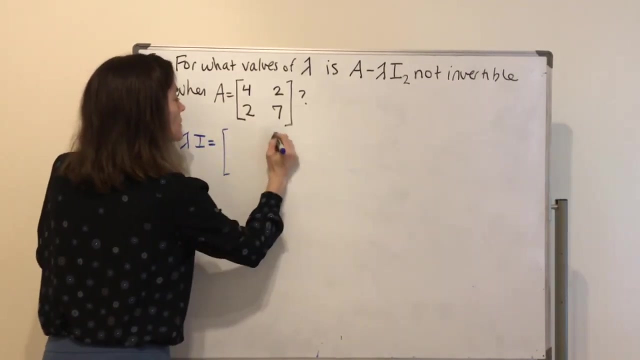 two by two. identity not invertible. well, we know. all we need to do is just calculate a minus lambda times the identity as a matrix and then figure out when the determinant of that matrix is zero. let's do this now. so a minus lambda i is equal to this matrix. maybe give a little bit more space here. this will be four. 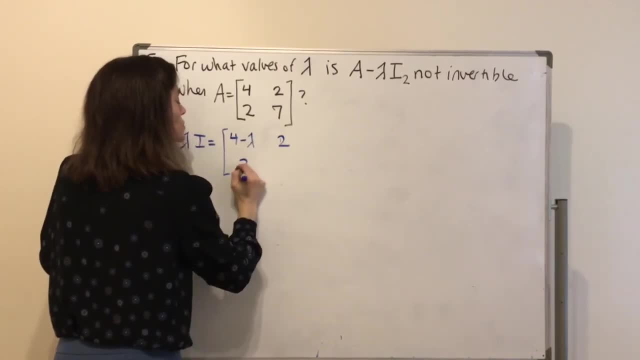 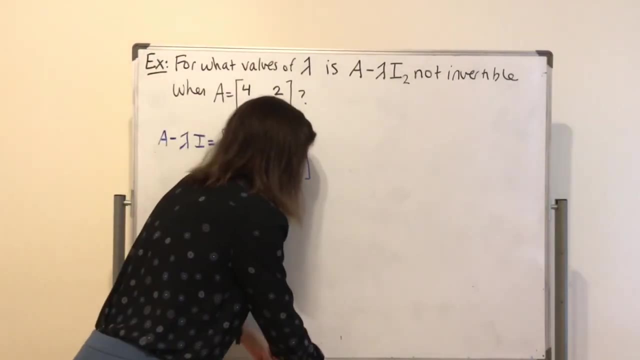 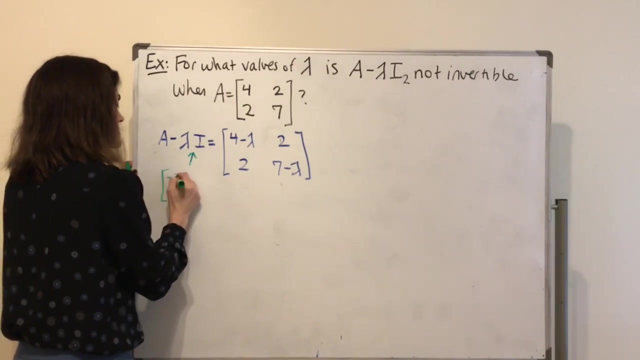 minus lambda. two, two, seven minus lambda. right, because, just as a side comment, if you didn't see that right away, what is this? this matrix, is this okay? how do you add two matrices? or how do you? yeah, okay, because i put pulled the minus in. how do? 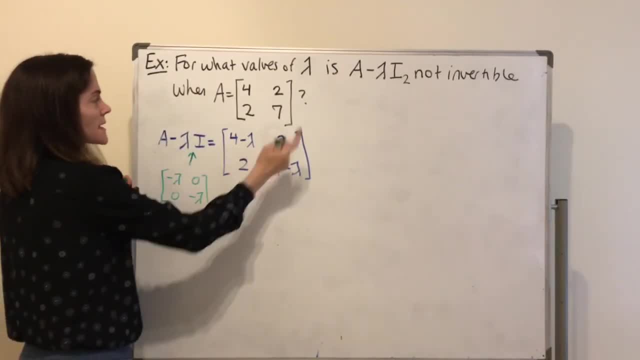 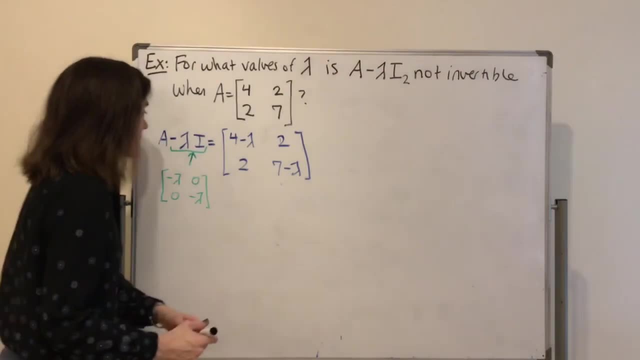 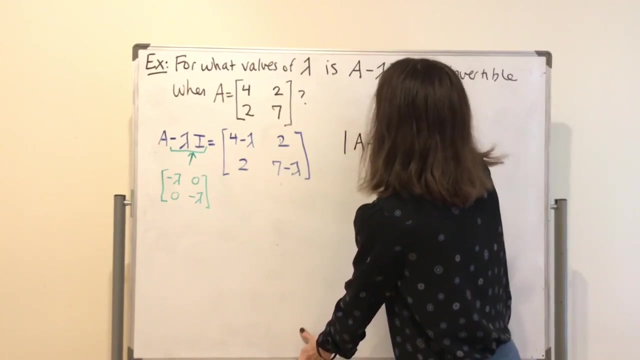 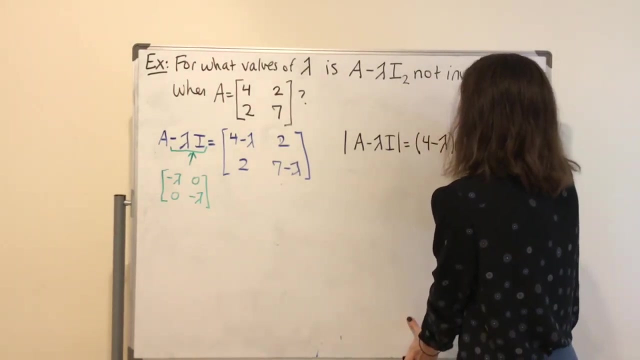 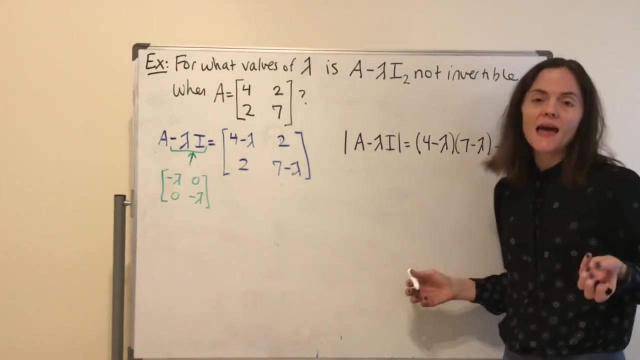 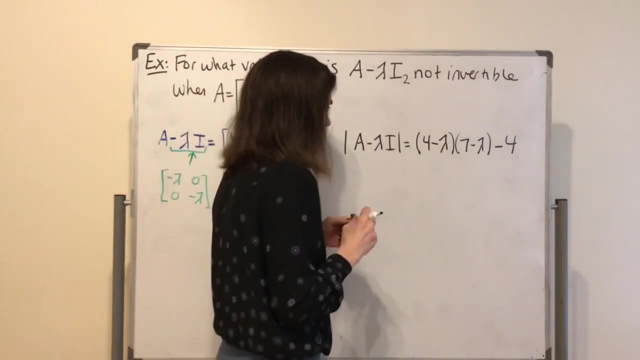 you add two matrices, component wise. so here this would be four minus lambda two, two, seven minus lambda. right like this. now what is the determinant here of a minus lambda i? this is our next step. so this determinant is: well, let's multiply four minus lambda, seven minus lambda minus four. but you see, i can't solve that. equal to zero, just looking at it. what i need to do is multiply everything out and then refactor. okay, so this is going to be a lambda. 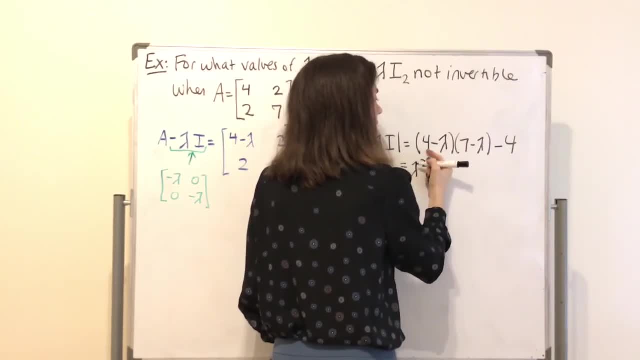 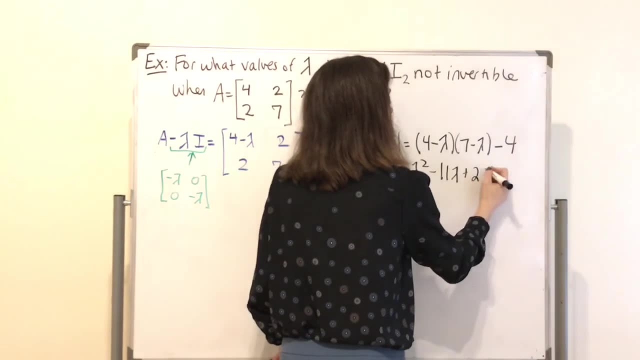 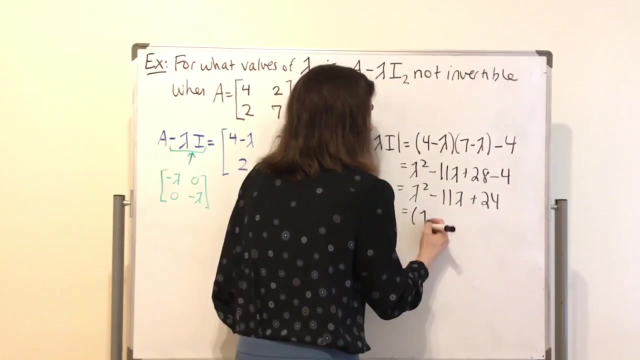 squared, we have minus seven and minus four, and then we have a plus twenty And then we have minus 4.. This is lambda squared minus 11, lambda plus 24.. I see 8 and 3.. Lambda minus 3 and lambda minus 8.. 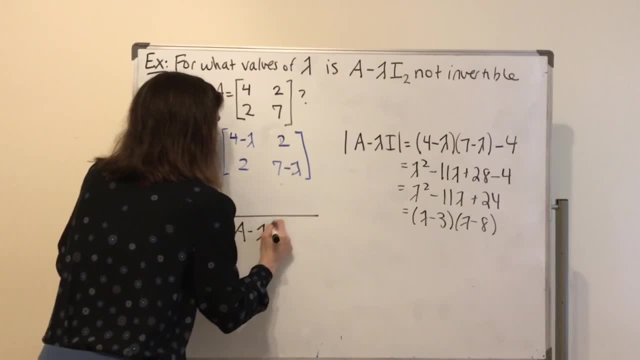 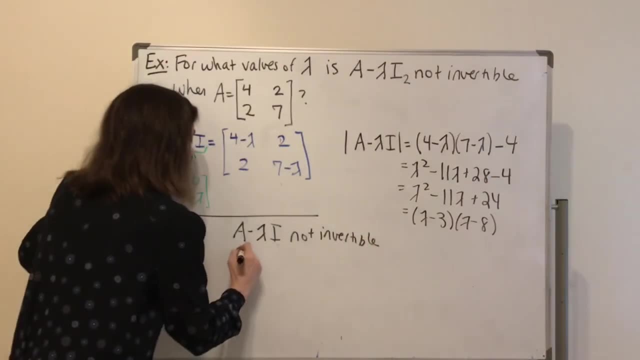 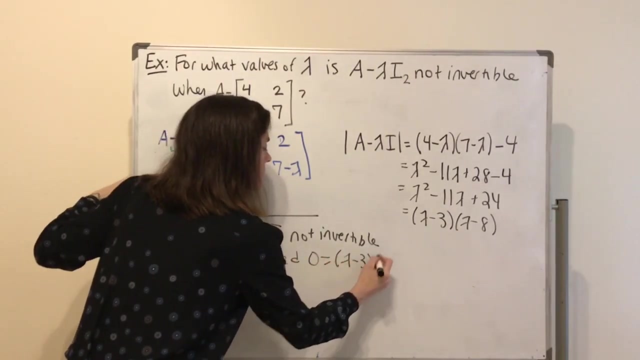 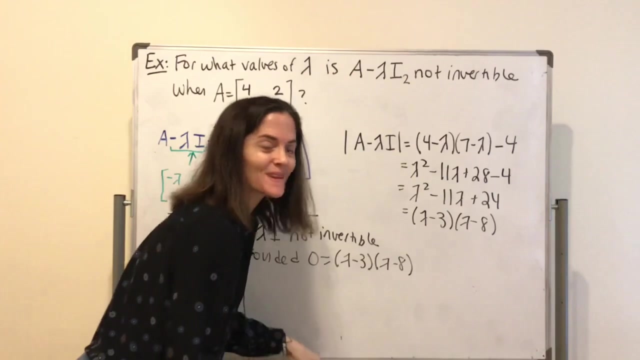 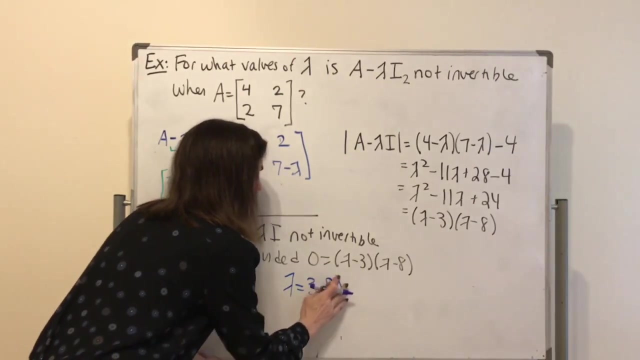 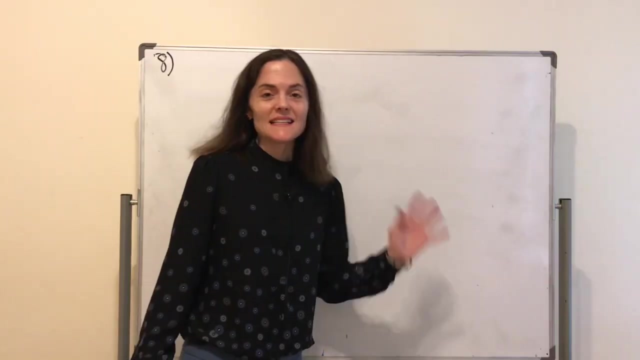 Move here A minus lambda. I is not invertible, provided 0 is this And there's only two answers or only two possible lambdas. They are 8 and 3.. So lambda equals 3 or 8.. Uh-oh, This is our answer. This is the last property I want to mention in this section. 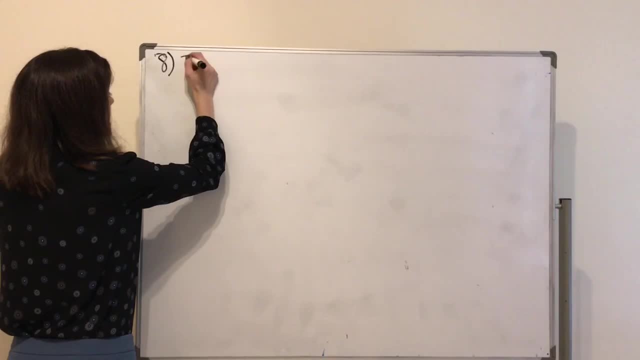 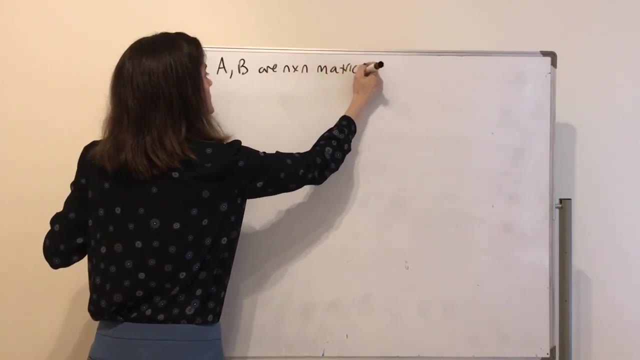 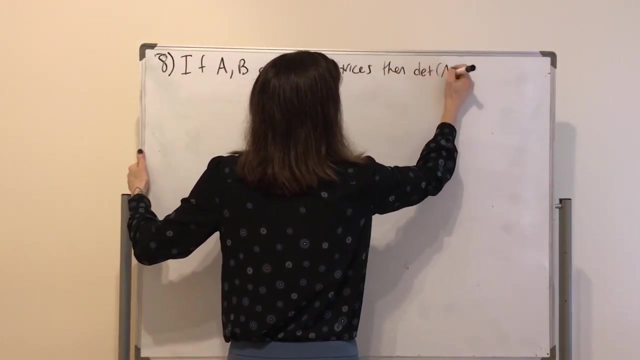 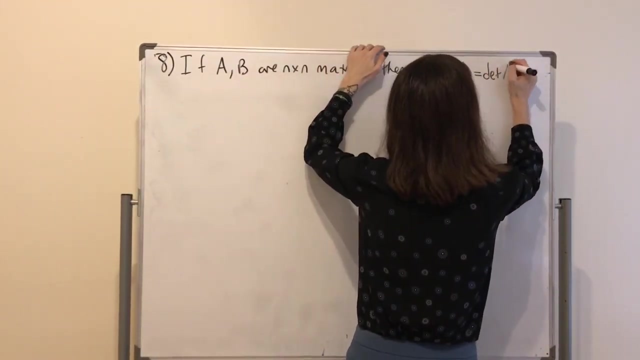 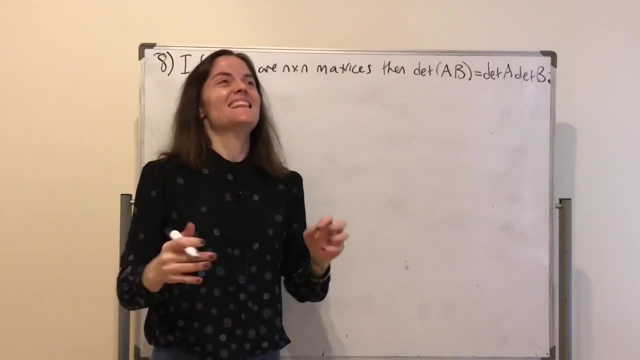 property number 8.. And it says that if A and B are n by n matrices, then the determinant of the property A times B is the determinant of A times determinant of B. So if you take a product, the determinant is multiply. Now, in particular, and this is an important part of this, 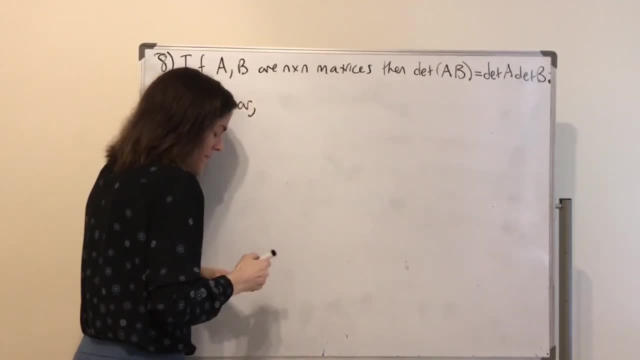 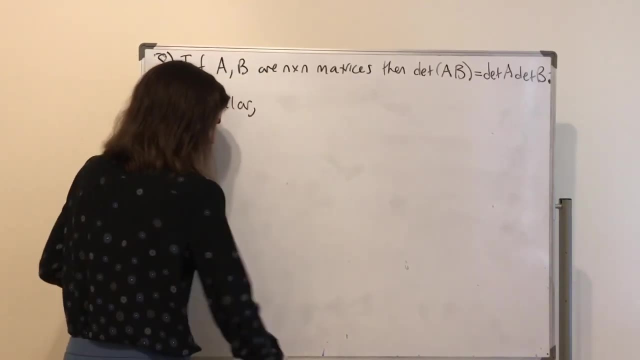 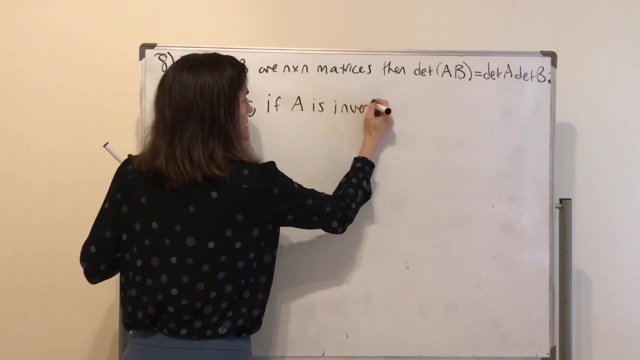 we have. well, let's think about this. Maybe I'll think about it in blue and then write the particular part in blue Black. Oh, I need an if, If A is invertible. Now let's think about this. 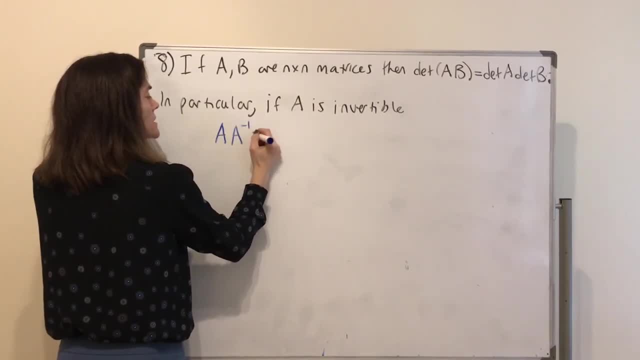 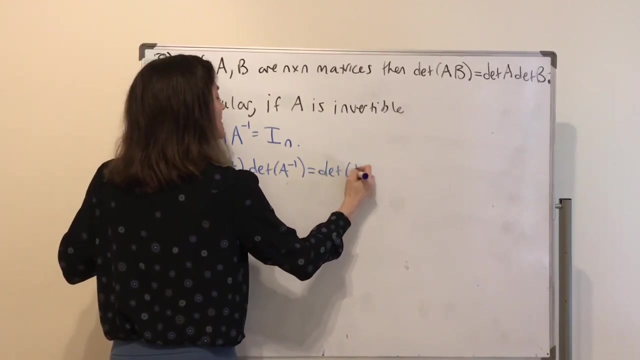 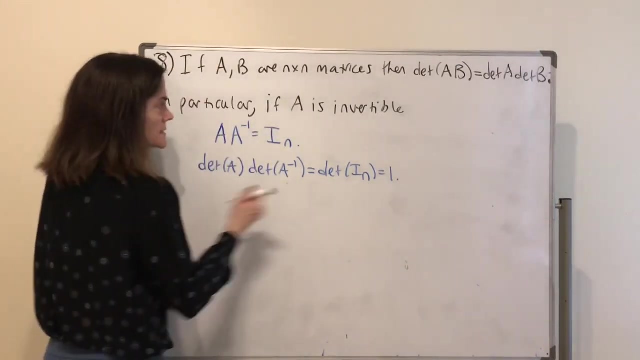 We know A A inverse is the identity. Okay, So the determinant of A determinant of A inverse equals the determinant of the identity, which is 1, right, So now, what's this in particular that I'm trying to say? if A is invertible, the determinant of A inverse is going to be 1 divided. 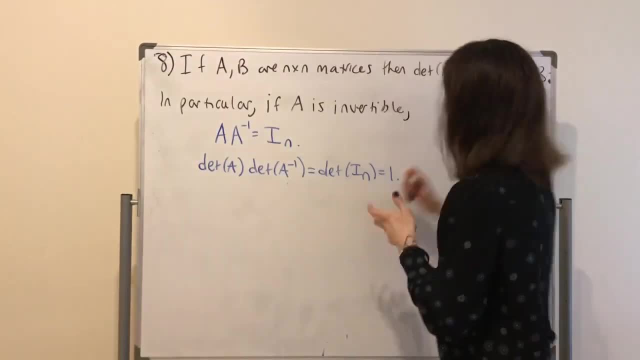 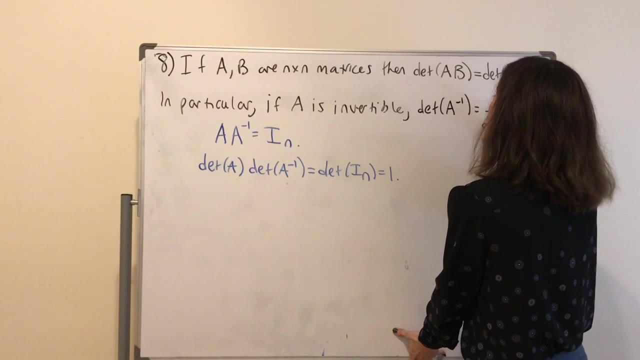 by the determinant of A. The determinant of A inverse is 1 over the determinant of A, Because they can always sum anything from one to the product, but they never tried to make a lot of OF the instrument. So A is invertible only when B is. this. A is 1 over the determinants of A ascendant. 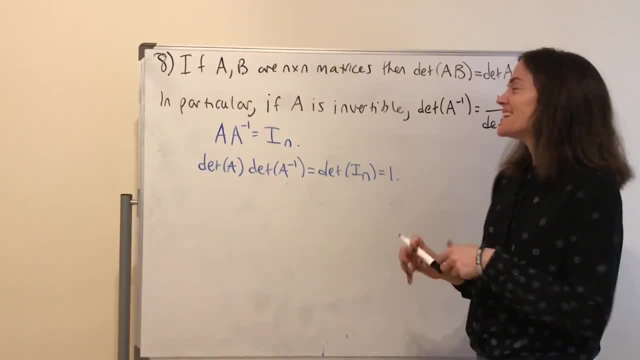 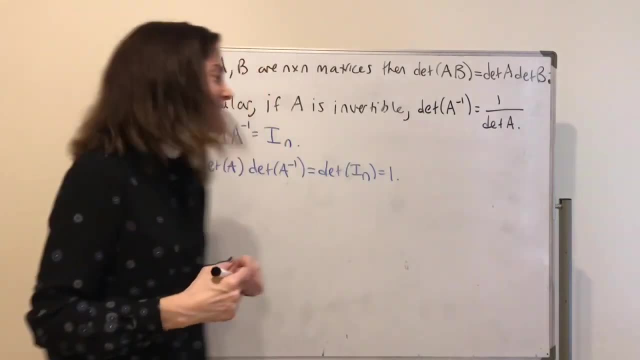 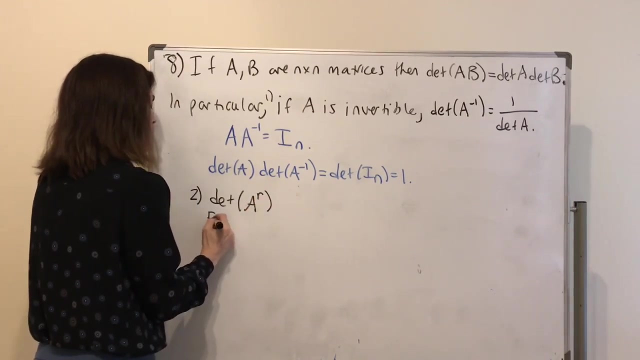 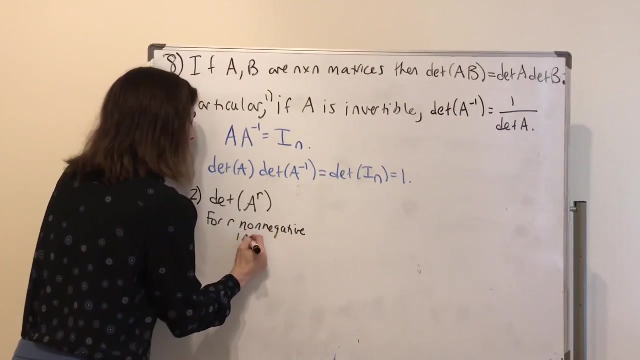 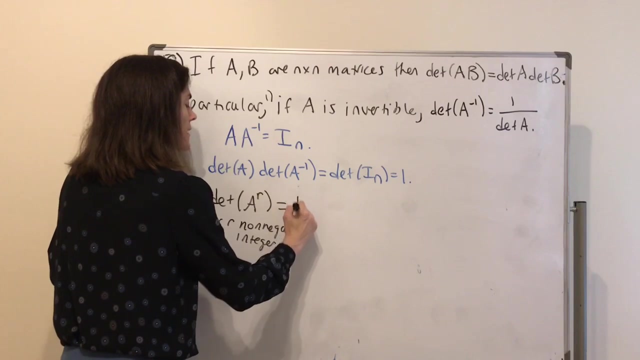 bye, bye, and see you next time, because they multiply to one. okay and also well. maybe this is in particular part two. if you take the determinant of a power, let's say for r non-negative integer, this would be well, think about it, it would be. i'll write it this way: determinant of a. 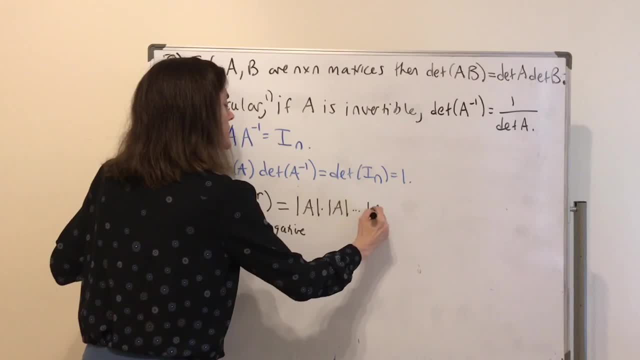 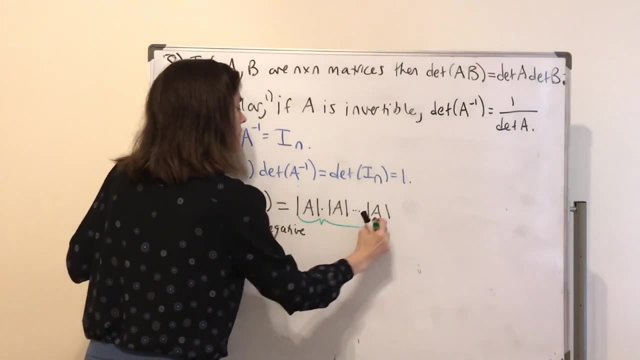 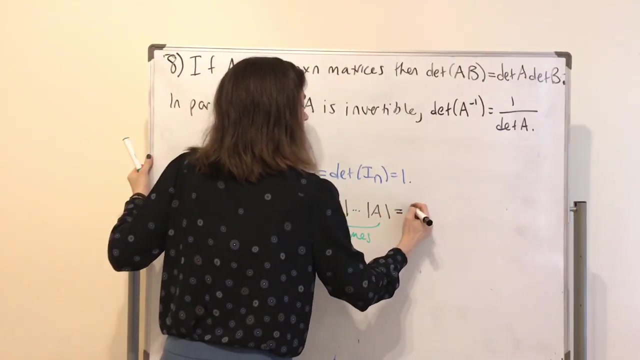 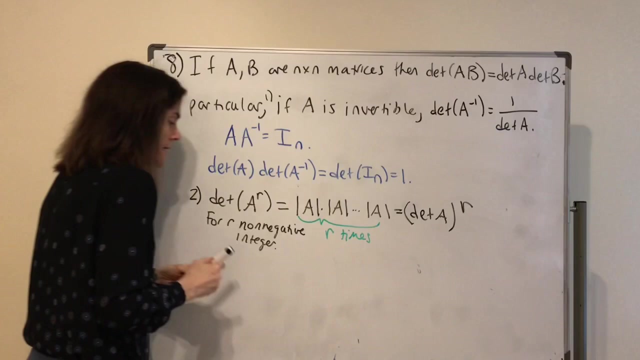 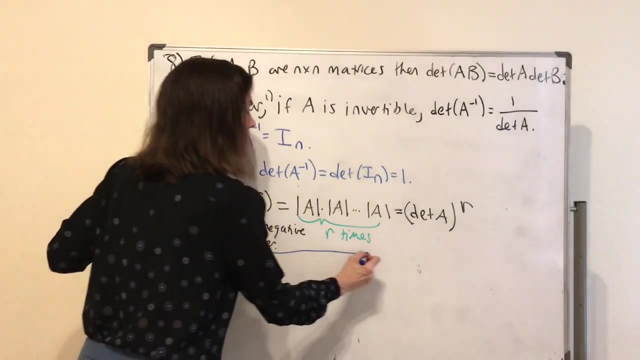 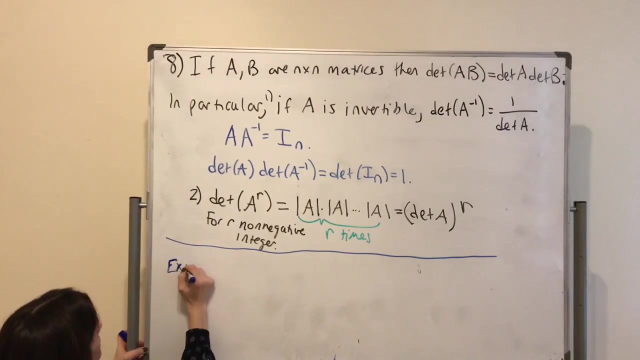 determinant of a, determinant of a r times using this, and so we get a. this is the determinant of a all raised to the r. now maybe a quick example. i'll put a line under this. we have room at the bottom for an example here. let's suppose a is the following matrix: two, five, eight, zero, four. 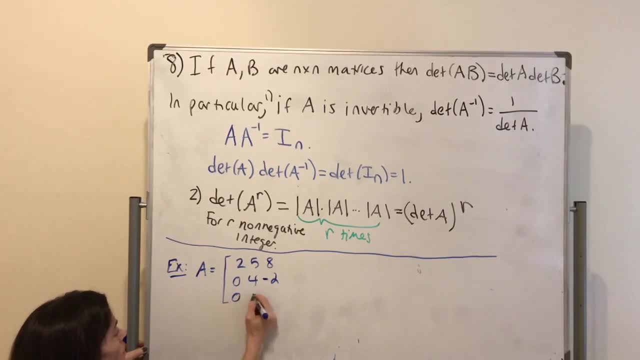 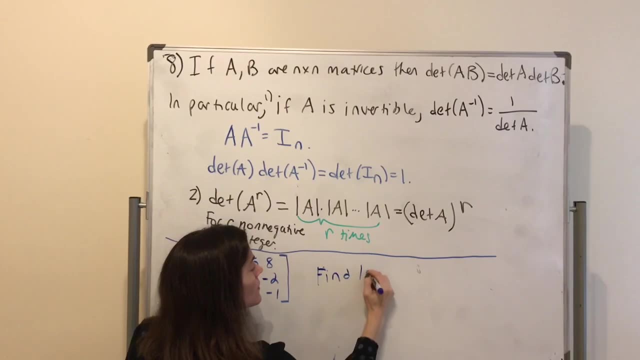 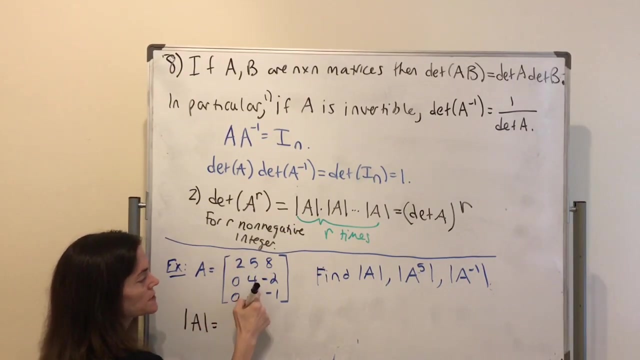 minus two, zero, zero minus one. let's find this. let's find the determinant of a to the fifth and let's find the determinant of a inverse. this is equal to four times two times minus one negative eight. and then- oh, i gave myself something hard to do. this is minus eight to the fifth. maybe i'll leave it like. 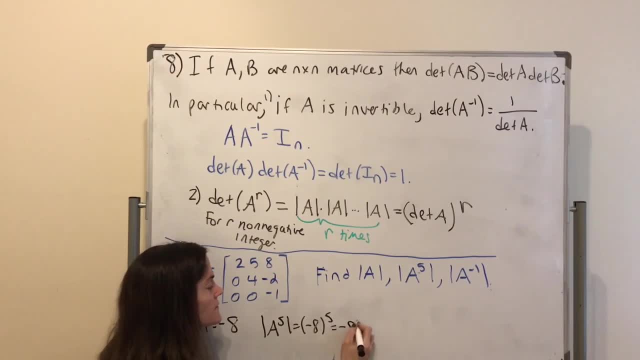 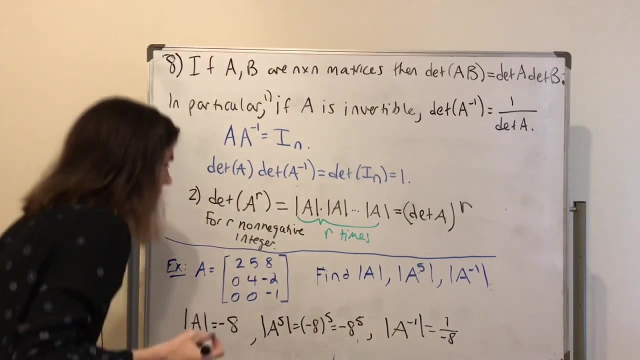 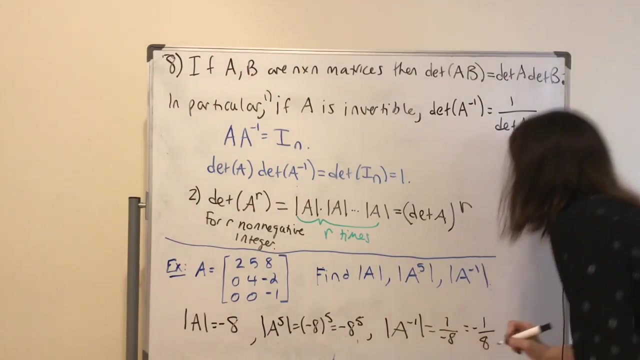 that what's negative, whatever eight to the fifth is. maybe i should have picked a smaller power. in any case, it's fine. and then the final answer: this is one over minus eight or negative one-eighth. okay, this is all, using this properties here. negative 1 over 8. the final thing. 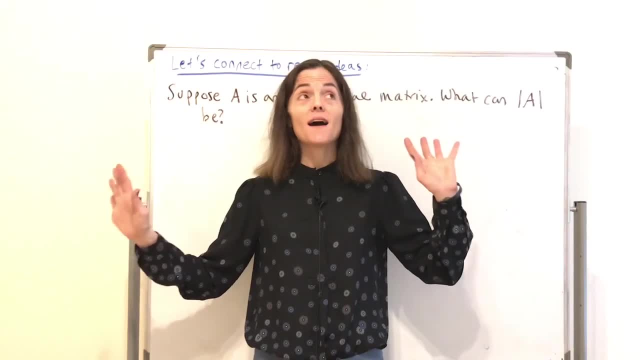 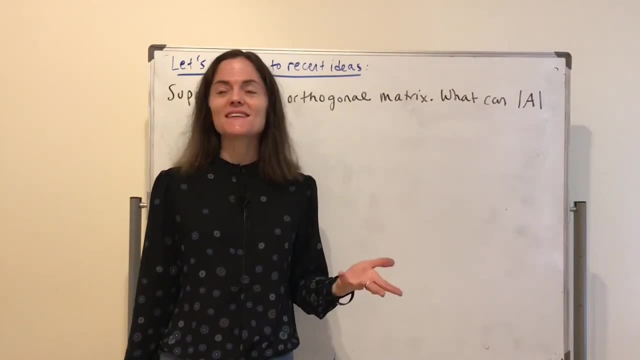 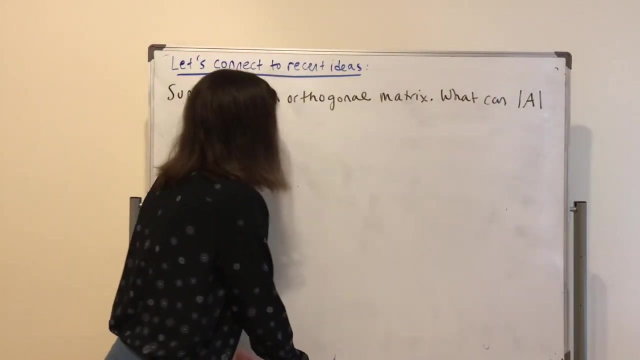 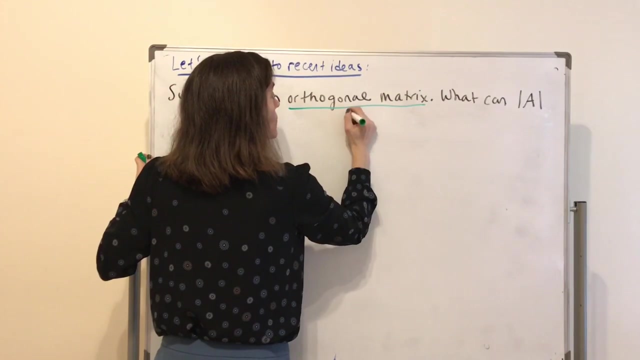 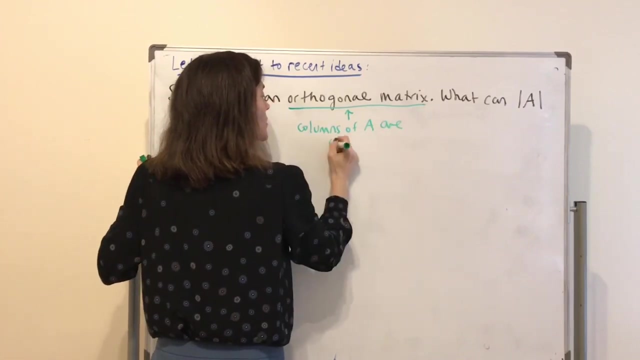 we will do today is connect with some recent ideas. okay, which is what happens when you have an orthogonal matrix, which we just spend a lot of time on ideas like this. well, let's remind ourselves what is an orthogonal matrix. first of all, orthogonal matrix: it says the columns of a are orthonormal and a is. 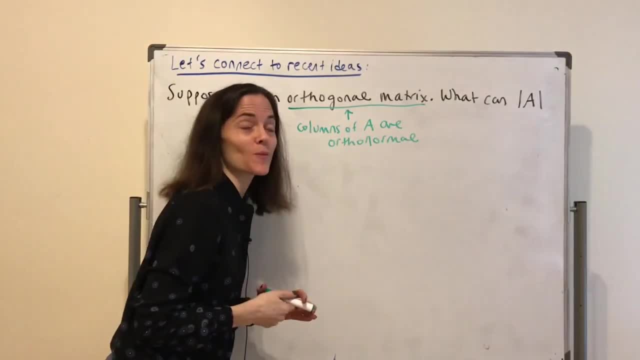 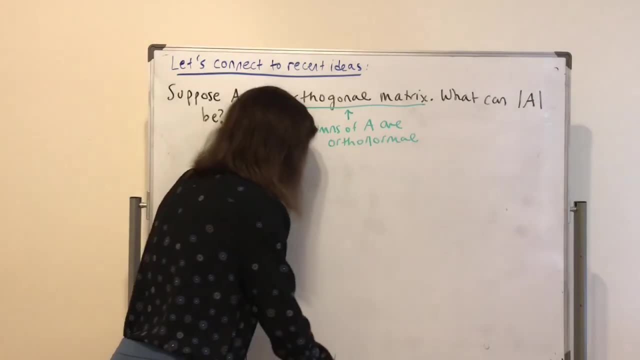 square, so in particular, the columns of a form, an orthonormal basis for our n right. okay, because it's square. well, but what I want to use to connect with an orthogonal matrix is: I want to connect with an orthogonal matrix. I want to connect with an orthogonal matrix is, in particular, let me figure: 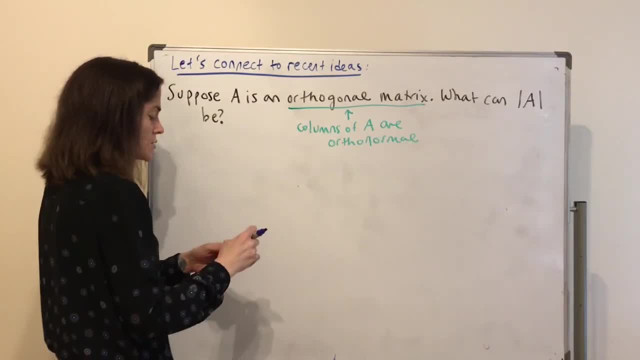 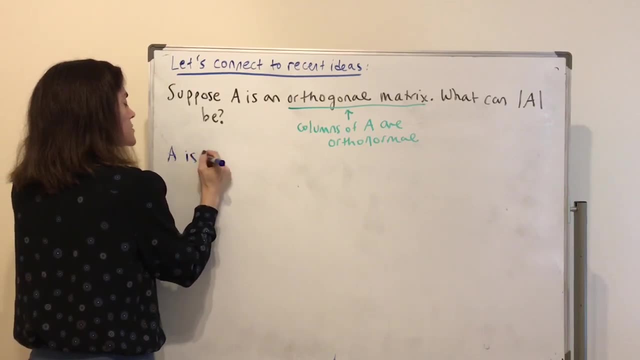 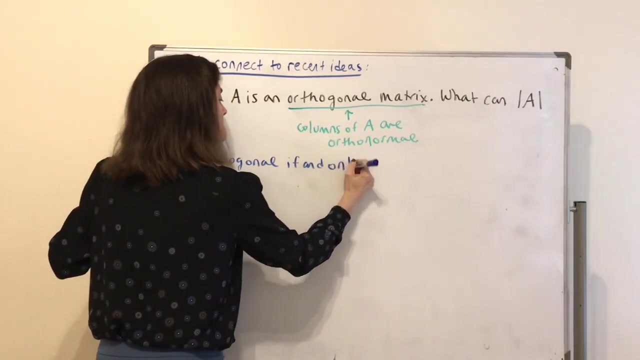 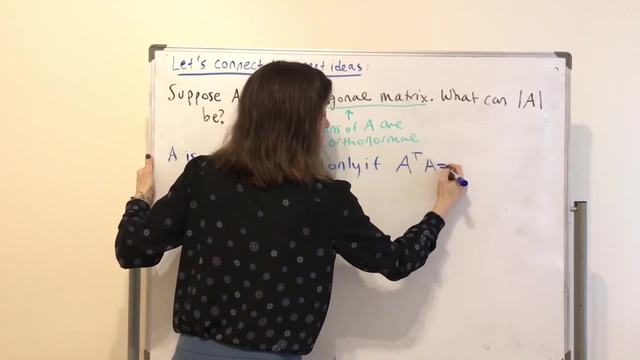 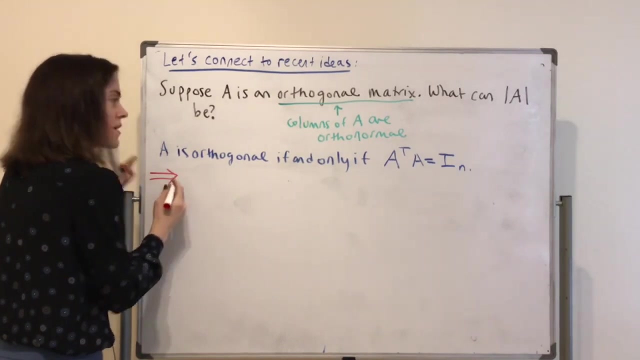 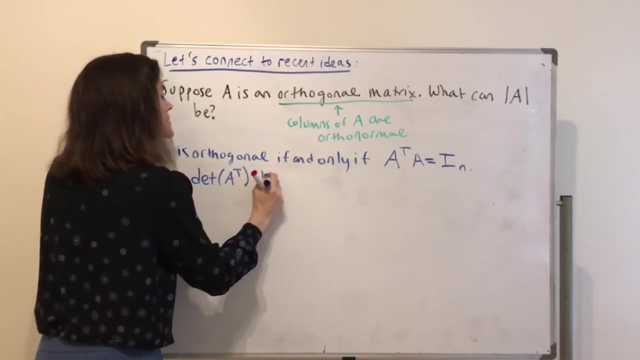 this out of what possible values can the determinant be for an orthogonal matrix? are to go back to this: if it, only if that we had. so we know A is orthogonal. one characterization was as follows: if, and only if, it was that a transpose A. from this we get that. well, the determinant of a transpose times, the determinant of a must be: 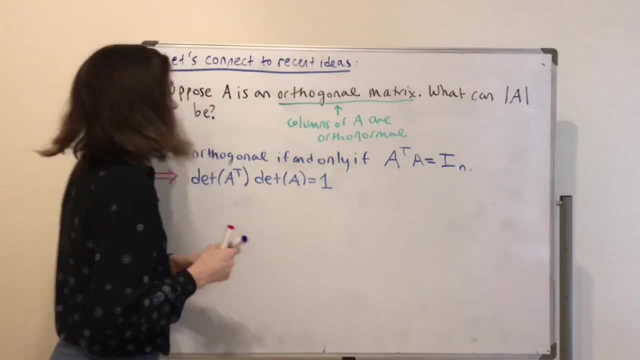 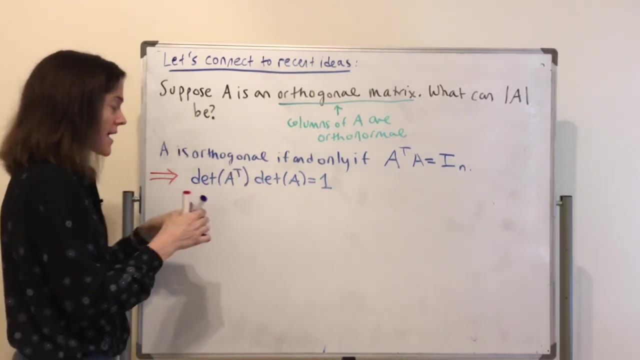 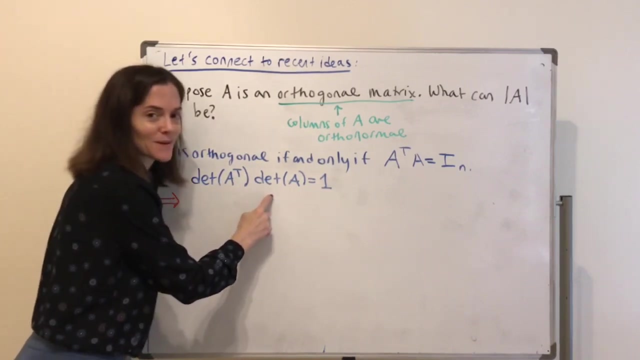 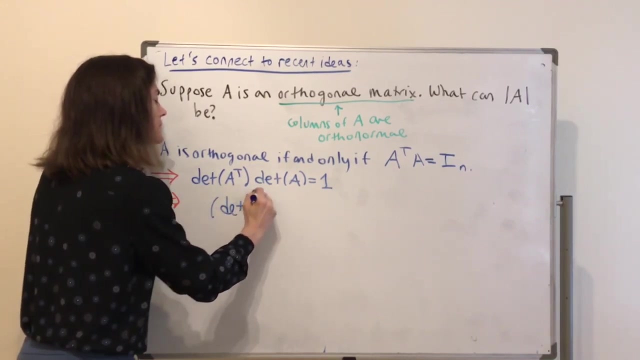 equal to 1, the determinant of the identity. and well, the determinant of a transpose equals the determinant of a for every matrix a, and if we use that here we see determinant of a times determinant of a must be 1, or another way to say that is the determinant of a squared must. 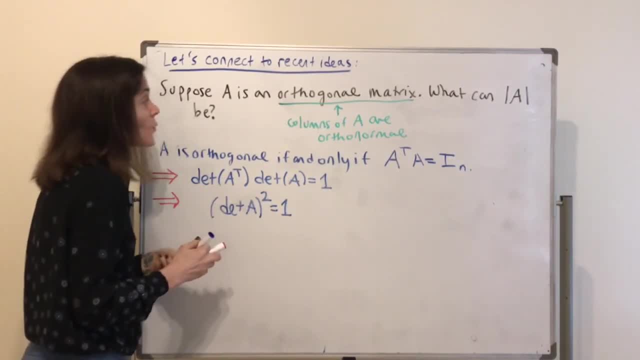 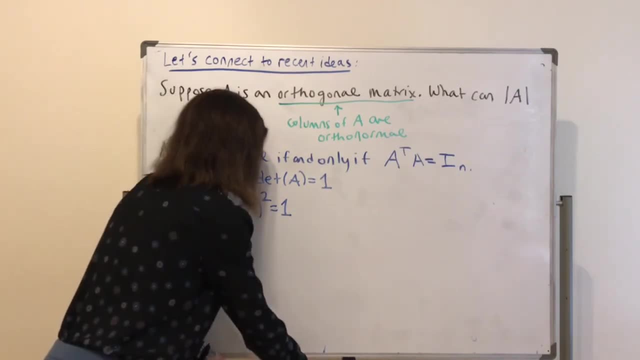 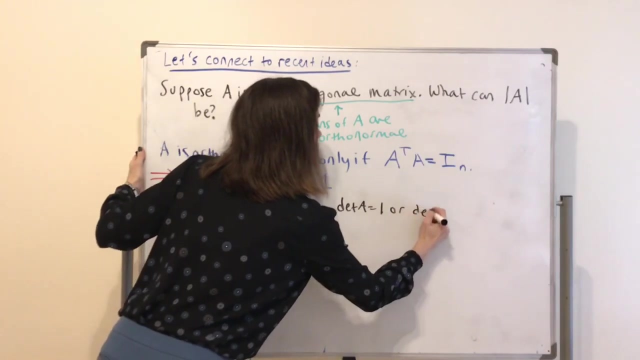 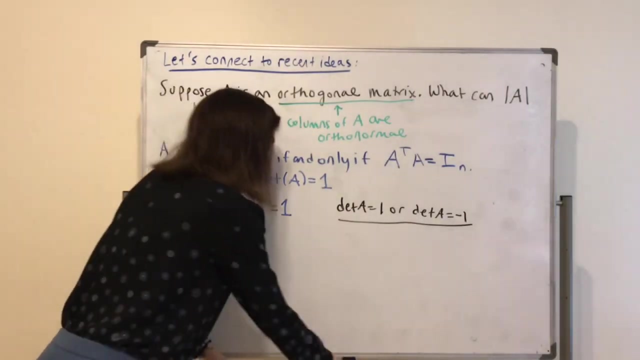 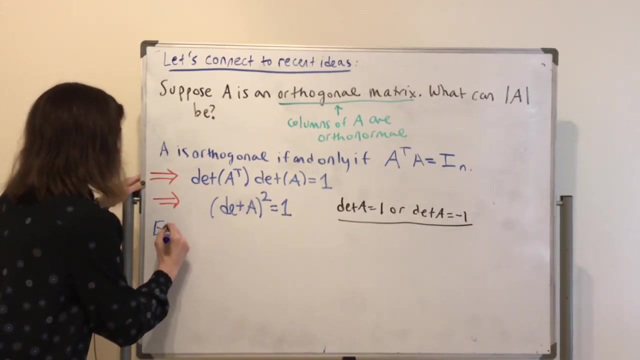 be 1. so you see, when a is an orthogonal matrix, there's only two options for the determinant of a is 1 or the determinant of a is minus 1. these are the only two possibilities when you have an orthogonal matrix. now let's look at some examples that do each if you have this matrix. 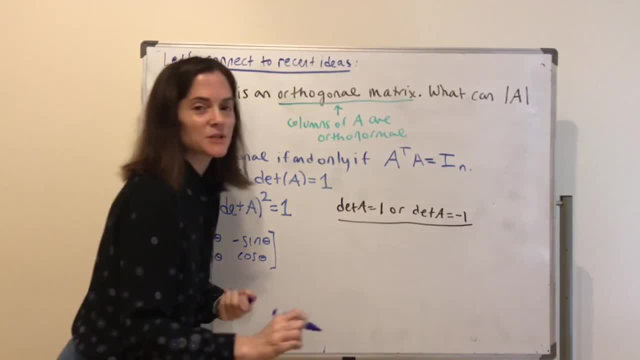 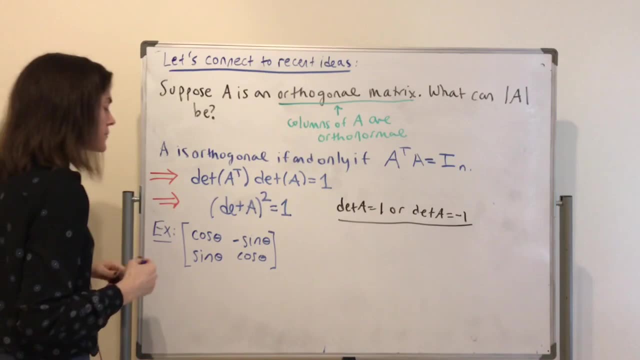 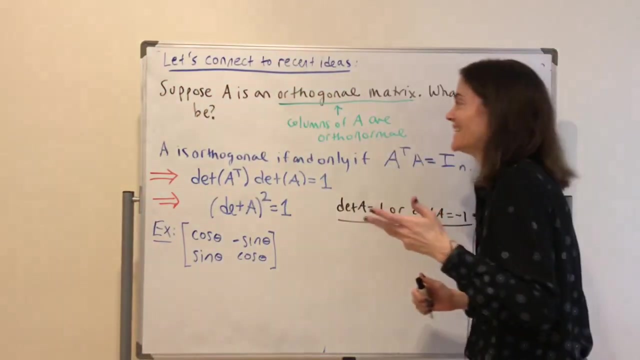 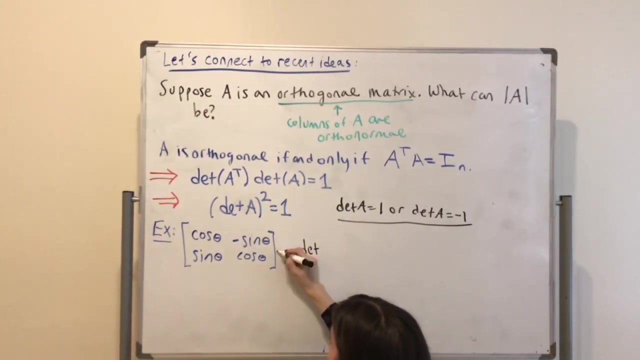 what is this matrix? this is rotation by an angle of theta counterclockwise right. this is an orthogonal matrix. it's one of our examples. well, what's the determinant here? better be either 1 or minus 1, okay, well, the determinant, I call this a. the determinant of a is cosine squared minus. 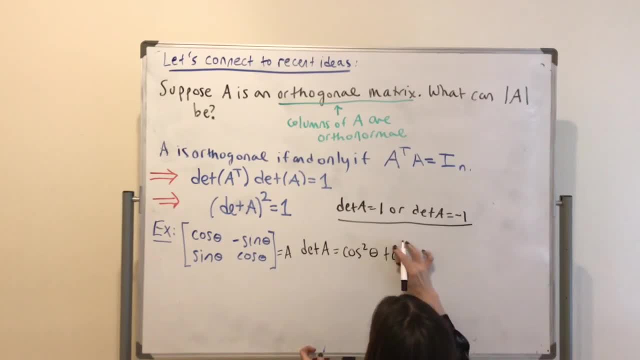 minus sine squared, which is plus sine squared, we get 1. okay, and we see, this is as I mentioned, this is rotation. so we see all, for example, all the rotation matrices, thinking about them, in our to have, the determinant is 1, no matter what theta is here. one more example here was if we had